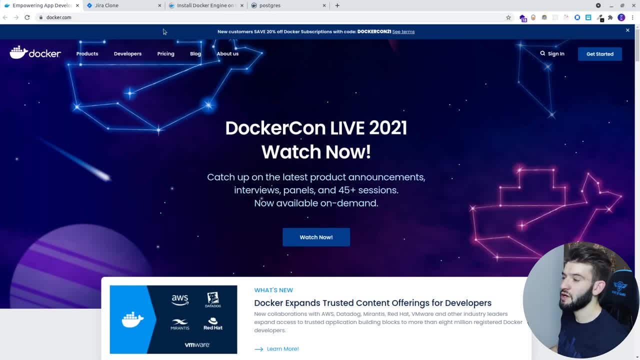 Docker works and all that sort of stuff, and plus we're going to integrate all of those together throughout like a Docker file. So we're going to take a real world application with a client, one on one, React and different technologies and, of course, with a Nodejs server running Express. 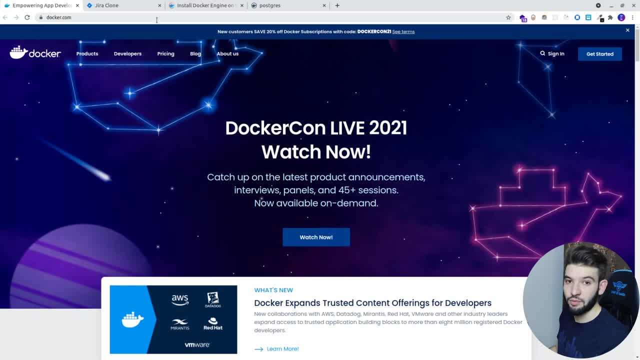 and with actually a database connected which is PostgreSQL. All of those are going to be like taken together as a stack. I'm going to Dockerize the whole software, like the whole stack, using Docker and, of course, we're going to use the advantage and like the CLI of Docker Compose. 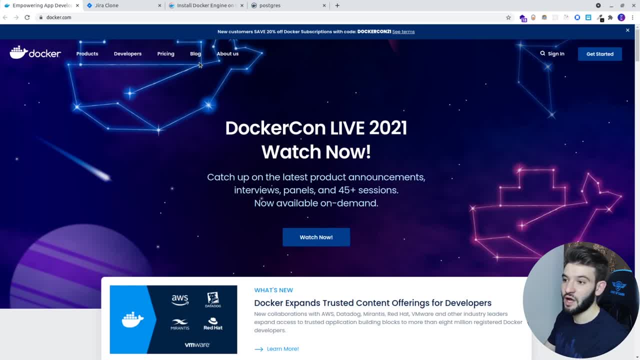 to put all of these services together and run them with a single line of code And of course, I'm going to have all this journey from start to finish into like doing this way on this particular video. So if we start off like in this one, like what Docker is like for a 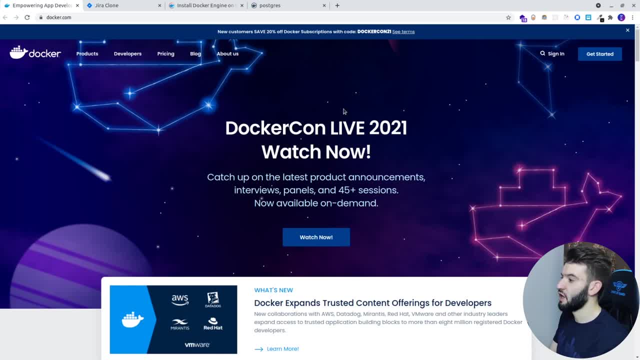 simple, beginner friendly startup on how or what is Docker is in this particular sense. So you'll see, this is actually the website of Docker. if you're not familiar with it, If you're like complete beginner to Docker and you don't know exactly what Docker is, Now Docker is simply is a set. 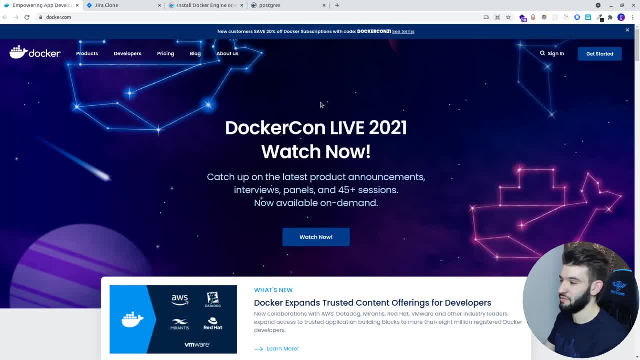 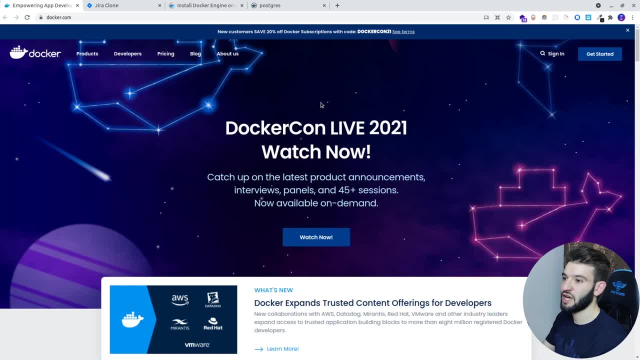 PaaS, or like products or platform as a service. So if you're familiar with PaaS or like products or service, sorry. So this is what Docker is it just like, provides you with this kind of like abstraction, like OS or operating system abstraction, and it's kind of like an alternative, I would say. 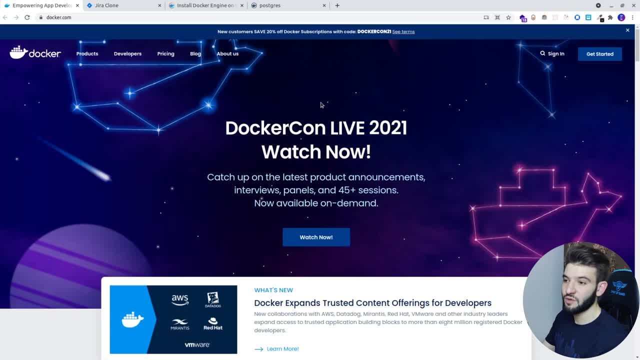 a really good alternative to virtualization. if you're familiar with that, we're running different operating systems, isolated from each other's, on top of host or something like this, where like virtual box or VMware runs. So this, where Docker comes in handy, it does kind of like. 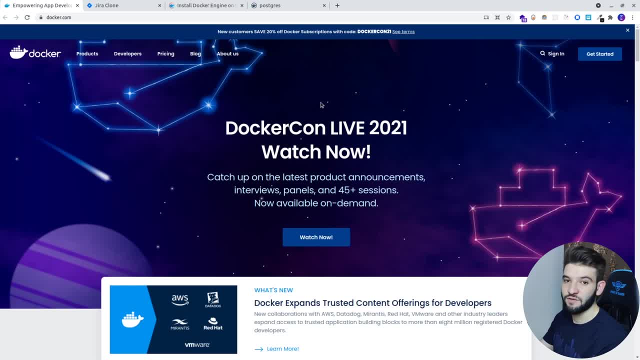 do virtualization, but I do it in a special way. it's kind of different from the other way around. do virtualization, but I do it in a special way. it's kind of different from the other way around. It does like an operating system, kind of like virtualization, which makes it super. 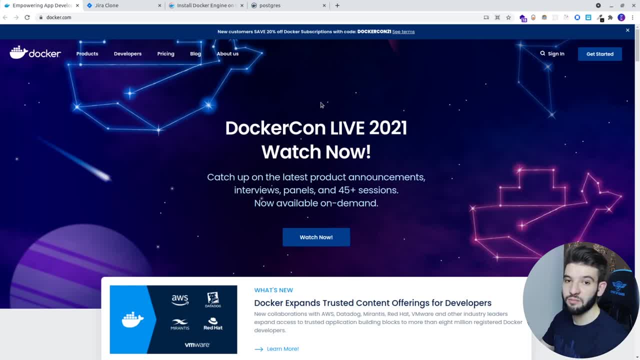 performance, super safe and processes are completely isolated throughout the whole kind of operating system, and he also to run tons and tons of containers at the same time without losing your sanity or without losing your much of RAM and resources of your computer. So that's basically what Docker is, and Docker, of course, allows you to run basically applications independent. 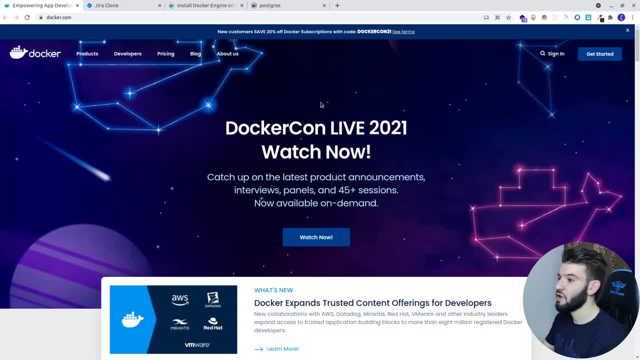 from each other's like, completely isolated from each other's, without the need actually to go into virtualization, without the need to write a really complex code. or you've got a need to go to run essentially a couple of like lines of code and you can turn your static, regular, standard application. 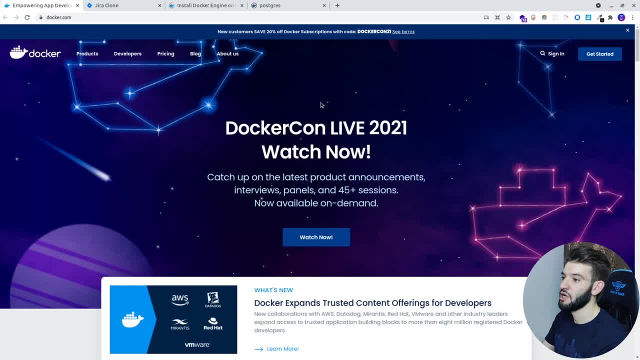 into a Docker compatible image application or like a compatible Docker container, running isolated from other containers, running isolated from your own host, running all in just like a completely bare Linux kind of like operating system or Linux kind of like container, having all that info. So that's basically what Docker is and that's basically what Docker does in that particular. 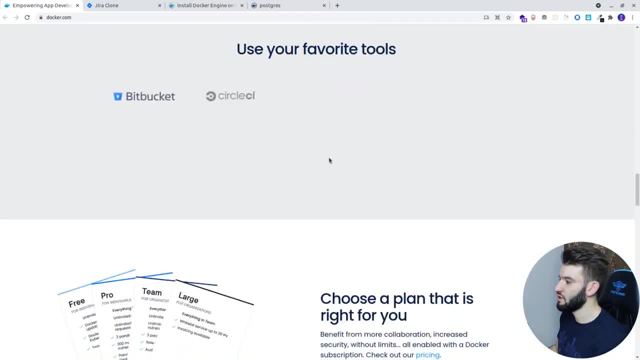 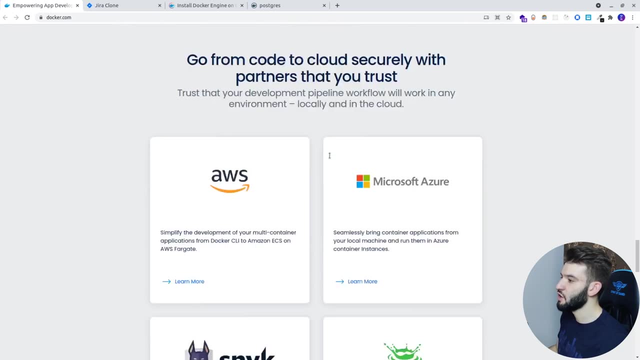 sense and that's why you've seen Docker have been shining throughout the whole years, and it's basically if you'd like been seeing this and didn't get have the time to actually go into Docker, well, this video is actually for you: to jump into Docker and know exactly how to go ahead and start with. 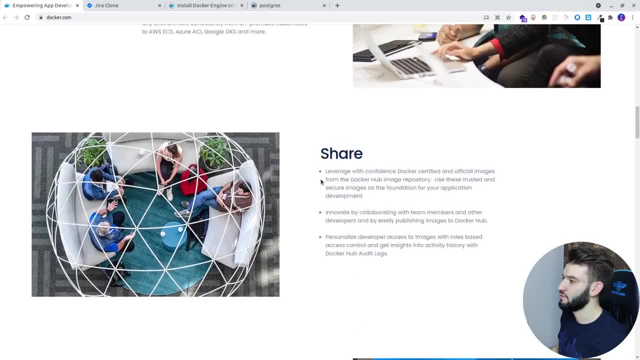 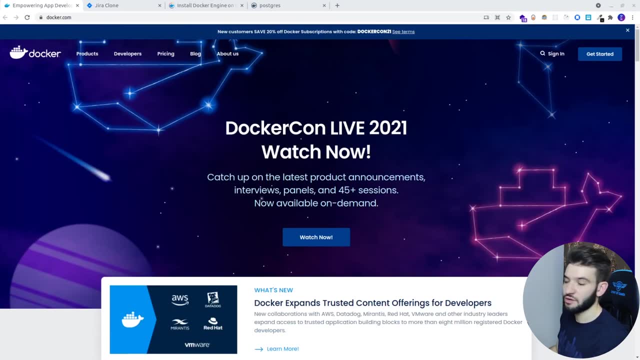 Docker and how to work with Docker And learn Docker from start to finish. So, if you see, this is basically the Dockers, or basically what Docker is, and in Dockers website, like how you do Docker and why Docker is very important, Right now there's this Docker cone live going on. Of course you can go in and watch it. whatever I'm going to. 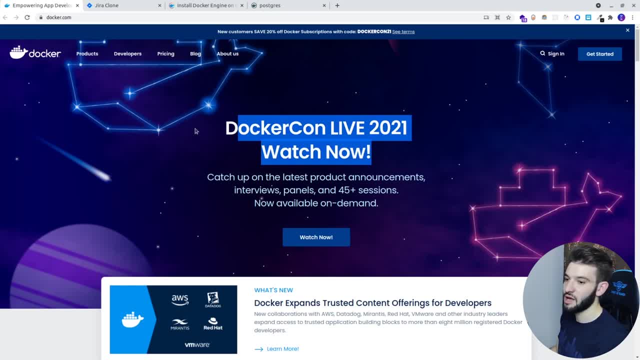 catch up on this, like on the kind of like recaps or something, but whatever. So that's, that's basically just like a simple introduction to Docker and how you do Docker basically. Now, the other question in here, before starting the video, is actually for your guys to know exactly like. 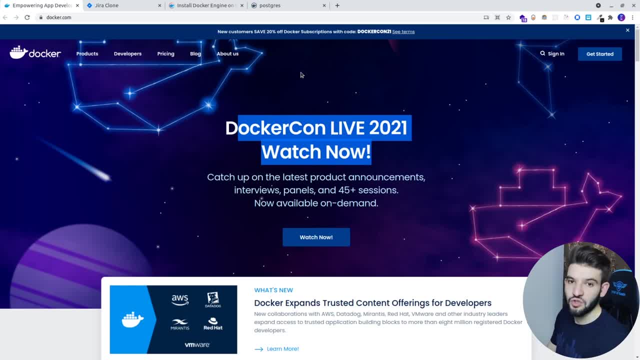 whether you start with Docker or not, Like. why should you choose Docker versus other kind of like technologies like VMware or virtualization in the first place? Well, Docker gives you the opportunity to run or Docker as your application in a really, really simple way at the lowest cost. 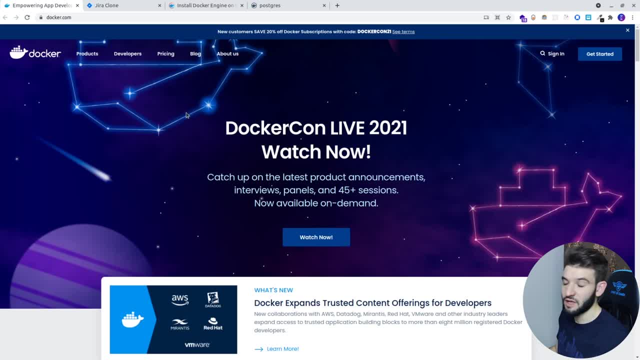 It's basically available everywhere. I mean it. it's everywhere, like servers running Ubuntu, Sen OS, Fedora, any kind of service, and like AWS, Google Cloud platforms and any kind of like platform. nowadays has Docker integrated with a huge capability and huge components integrated. 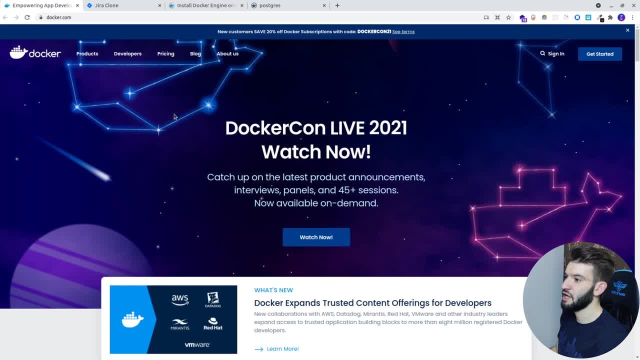 throughout the Dockers ecosystem. Now for Dockers in this side, you can actually take your own application and you can turn it into a Docker compatible. Then you can have this application actually built into a static image, and this static image- what it does- is just like a static. 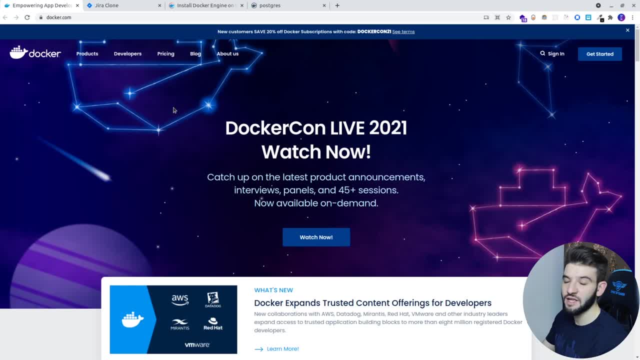 with the whole instructions, with a whole source code and everything you need. Then you can take this image actually distributed with your, with your team, with your rest of the developers over the rest of the world, as a lot of people are doing open source stuff and those images can be pulled. 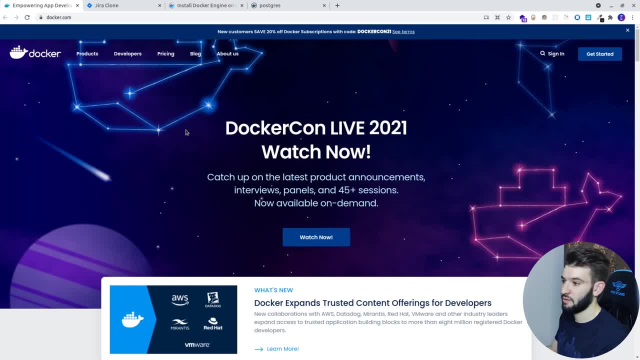 down into like local machine and they can like run this like images or run this containers, which of course, images turns into containers like never before. and those containers, what they can do is pretty much anything like running an isolated, simple and minimal and really small kind of like operating system. 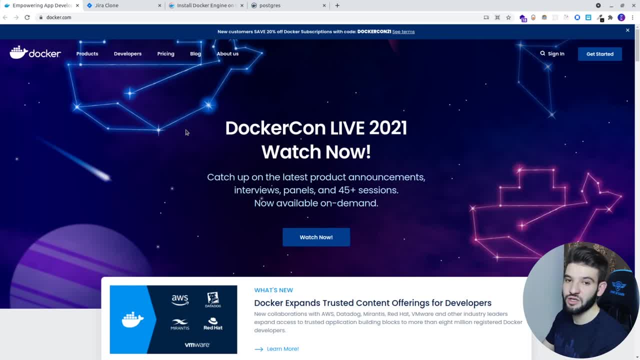 inside of your operating system. that does it really well. So imagine you can go in and run like a MySQL server without going to do like the fuzzy and the ugliness of installing MySQL on your server like Ubuntu or something like this, or you've got to go and do like go with Docker. 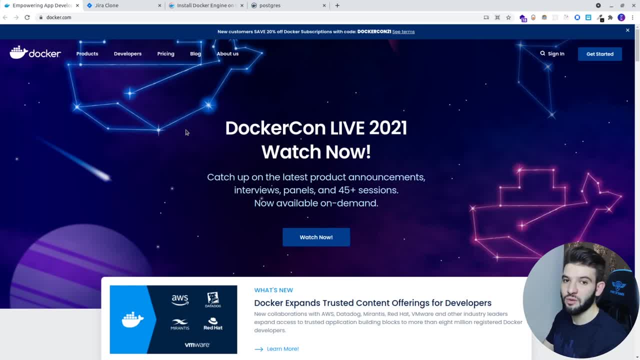 you pull the image, you do Docker, run MySQL, ports 3306 or something, and, hallelujah, you got MySQL running into Docker and everything you needed. All you have got to do is actually connect to MySQL and get up and running with your servers. 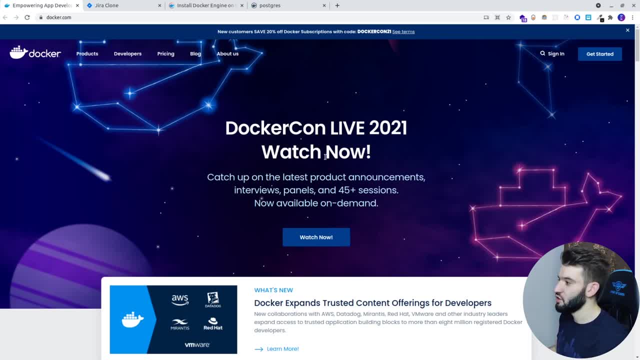 So that's basically what Docker is- if you'd like summarize it, of whether you need Docker or not and how to do that, And, of course, in a DevOps perspective, Docker makes our lives much, much easier as developers. We don't have to worry much about how deployment is done. 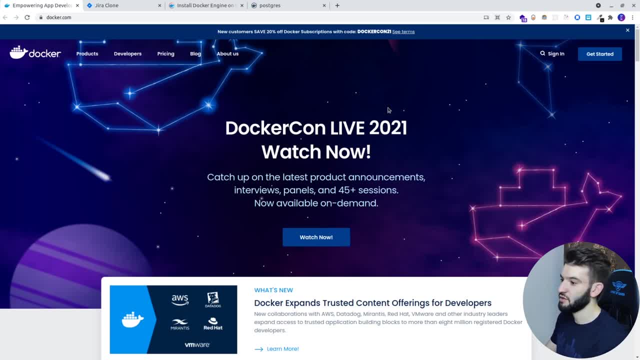 and how servers configuration is done and all that sort of stuff. All you need to care about is actually Dockerizing your application, adding the proper configuration file for Dockers and boom: just build the image and deploy it and you're ready to go. 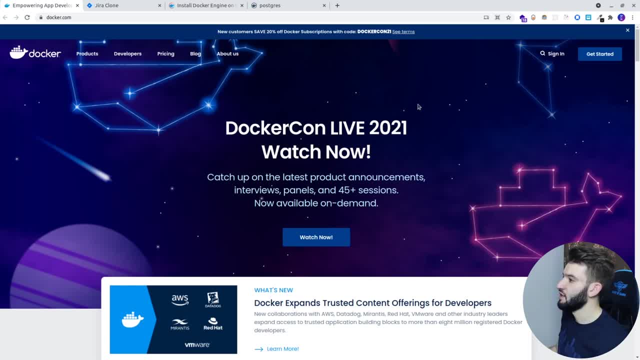 That's it, that's how all it does with Docker and that's all you need. So, yeah, so let's just like a simple kind of abstracted description of about Docker and how it works with that. So we're gonna be just like going and starting. 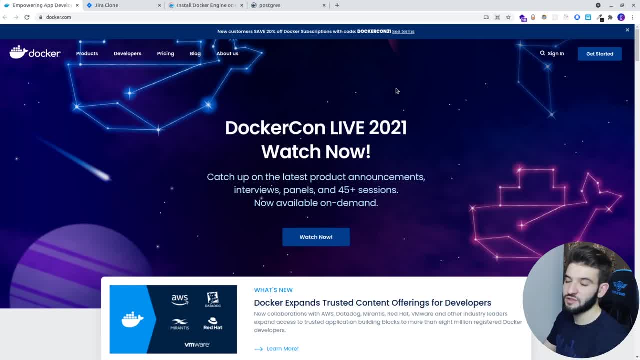 with installing Docker and get up and running And of course we're gonna get all the rest of the stuff about like Dockers and what Docker containers are and Docker images and managing all of those throughout the actual CLI And eventually, of course, as I said before, 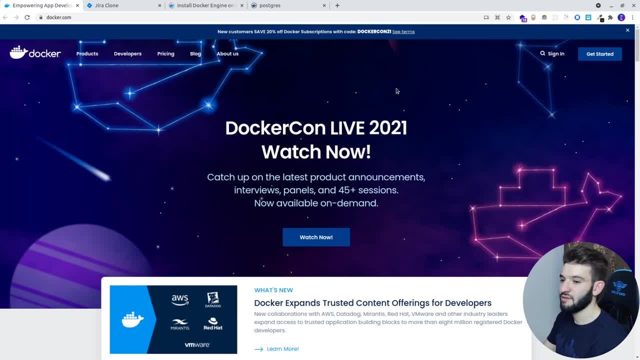 we're gonna Dockerize the full application. we're gonna use Docker Compose and we're gonna make sure that we do this in a really funny and awesome way, as we always do it on Code R1's channel. So if you're new here, make sure to go in and subscribe. 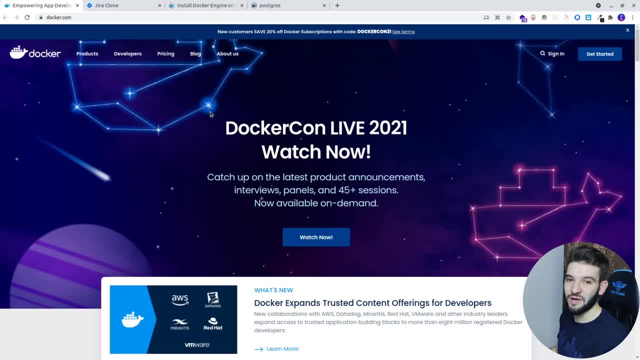 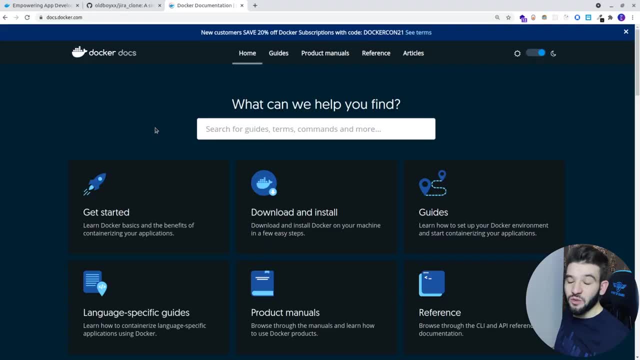 and push that like button And without further ado, guys, hope you guys enjoyed it and we'll go ahead and get started. So let's go ahead and get started And first things first, what we need to do is actually install the Docker engine. 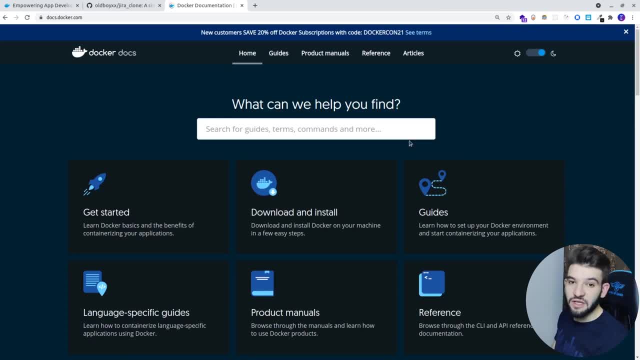 So if you're familiar with the Docker engine and everything, how it works basically underneath, well, you have got to install the Docker engine, which is basically the whole engine, or what's called the Docker demon. that's gonna empower how Dockerization is gonna work. 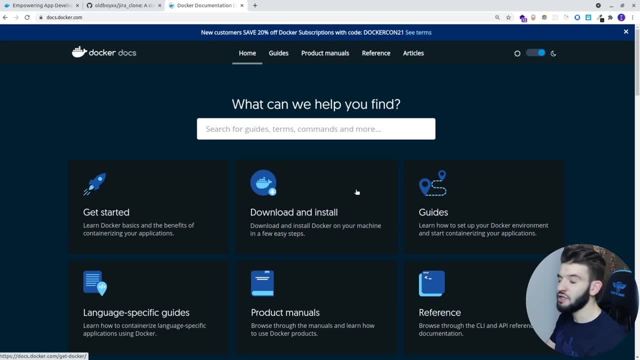 or containers are gonna run on the host machine. Mainly Docker best works for the Linux operating systems. So right here I'm running Linux Ubuntu, latest version of Ubuntu, and it's pretty much gonna run as smooth as possible For all the kind of distributions. 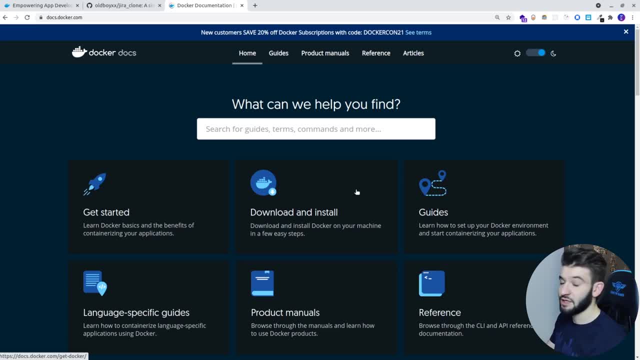 Docker works really really well. But what I mean by this acts like Docker is really supported on Linux and more specifically, on just like Linux operating systems. But for other places like Mac OS X and Windows, yes, it does work really well, And installing there is just like kind of straightforward. 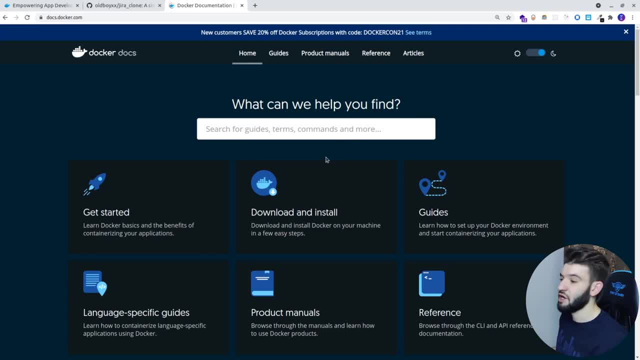 and pretty simple to install, because there's just like this kind of like binaries and executables that you click, you run, you click next, next, next, And there you go, You got the installation done for you and everything. So this is pretty much what I'm gonna try to say right here. 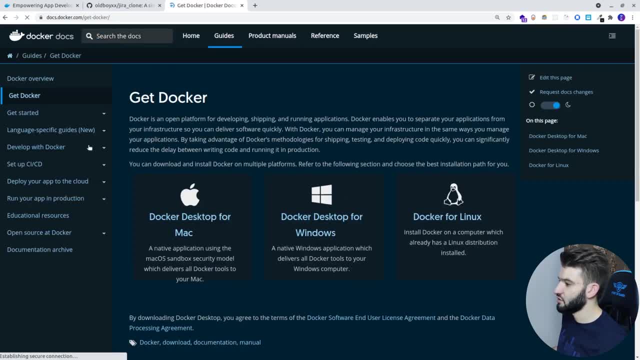 And we can just go and access the Docker or the download and install sections. So you see, there's a ready-made Docker desktop for Mac and a Docker desktop for Windows, But for Linux it's quite completely different. And if you're on Windows or Mac, 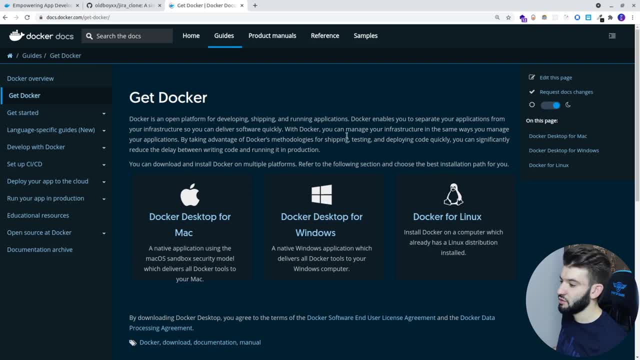 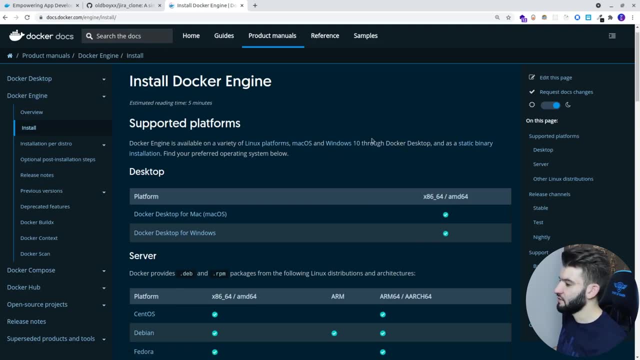 just click on one of these in here. I'm gonna take you down with the executable. You click it, you install it. that simple. Now for Linux. it's quite different. It's quite kind of like a little bit kind of hectic. 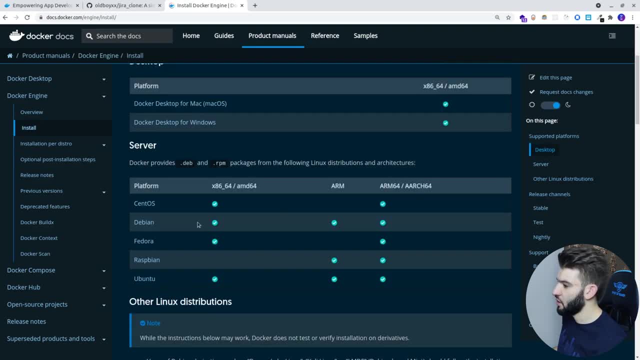 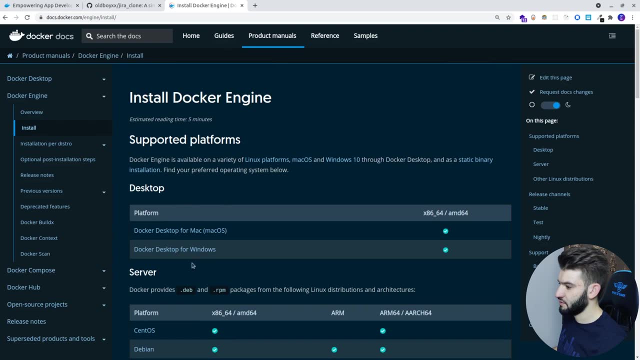 You have to go ahead through it and read more like what architecture you're on and a different. you know the servers in here. There's actually desktop security for both of these, but this one is more specifically designed for servers and how they work. 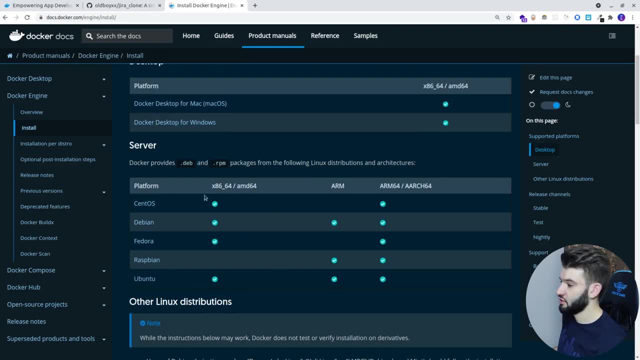 So, as I said before, I'm running Ubuntu and my architecture is like x86. So, yeah, we don't have to worry about ARM or something like that if running any kind of like CPUs. So if you choose Ubuntu in here, it's gonna take you to a lot of things. 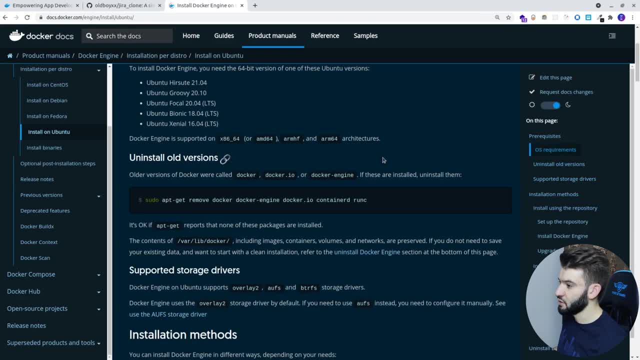 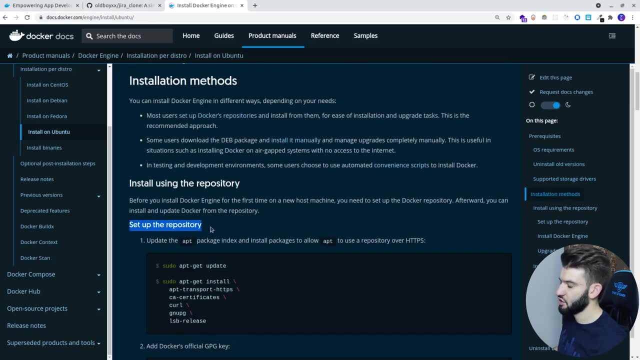 It's gonna take you to another page And this is where you need to like install the new Docker. If you've got like an old Docker version, you can even install it first, but the installation method should be pretty simple, And this is the installation method I'm gonna use in. 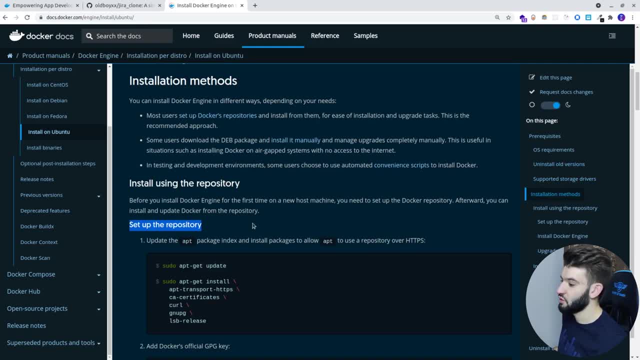 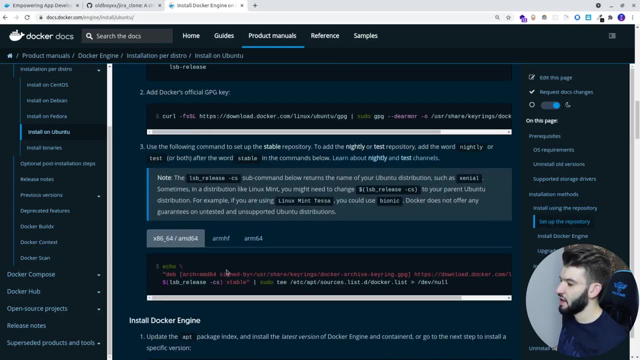 which is basically just following the installation throughout the repository, which is officially how it should be done. So you just like you update the install, then you just like you know, download the script and run that and just like install the Docker engine and that's it. 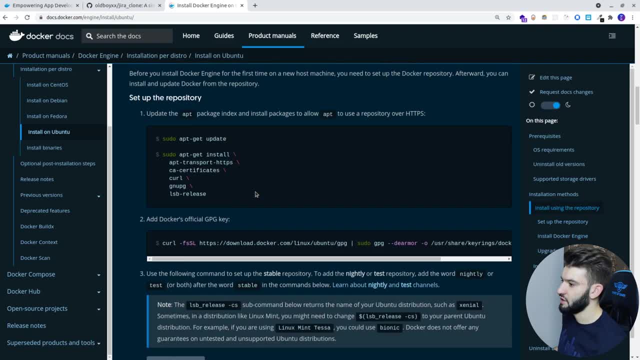 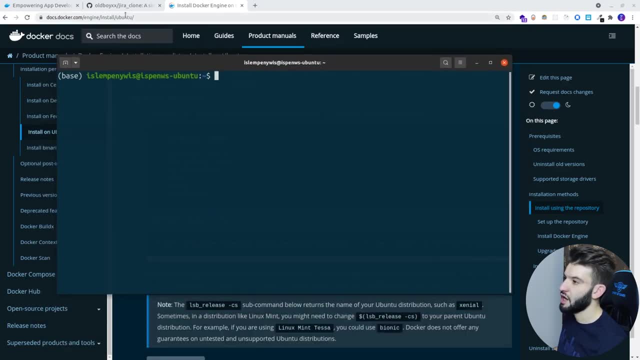 So that's pretty much all you need to do. That's pretty much all you need to do for that particular case. So, yeah, we can go ahead and just like walk you through on how you do this on like Linux in here. It should be pretty simple, as set before. 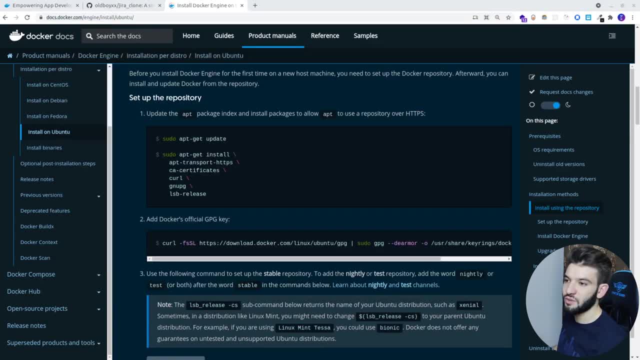 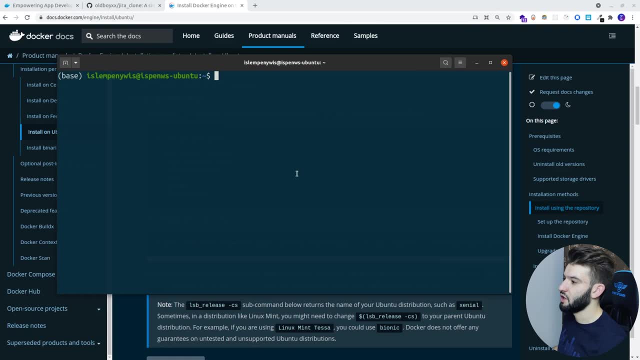 Nothing really so too complicated or something. So all I'm gonna be doing is just like copy pasting scripts and that's it. So just like following this tutorial should just be copy pasting scripts to install the Docker engine on Linux. And yes, I'm saying it one more time. 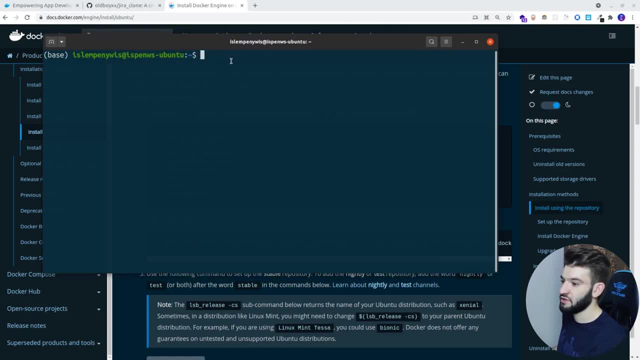 This is gonna be on Linux, For Mac or Windows. just download the executable, execute it and you're ready to go. So you have got nothing to do anything other than that. Okay, So pretty good. Now let's go ahead and jump into how installation. 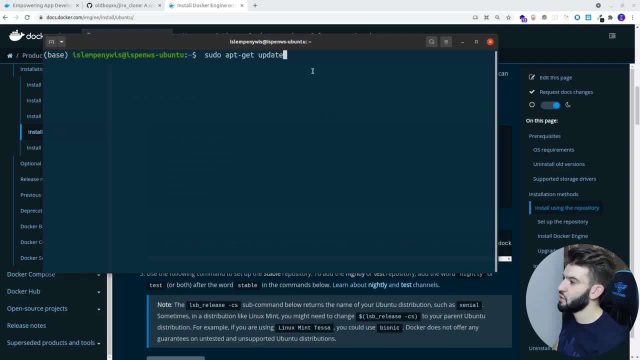 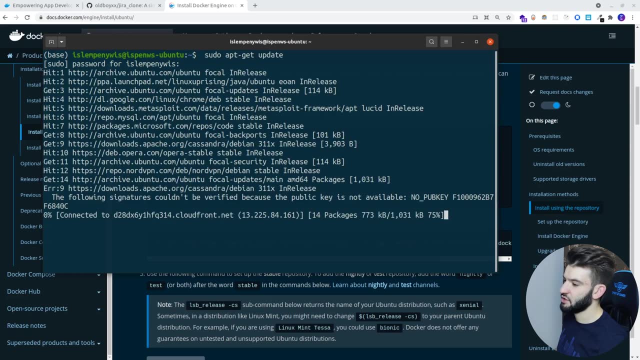 So first things first, what I'm gonna be doing. I'm gonna do sudo update, which is gonna update everything for us. I'm gonna install my sudo password and everything. It's gonna do the full update and everything. So it's gonna take a couple of time. 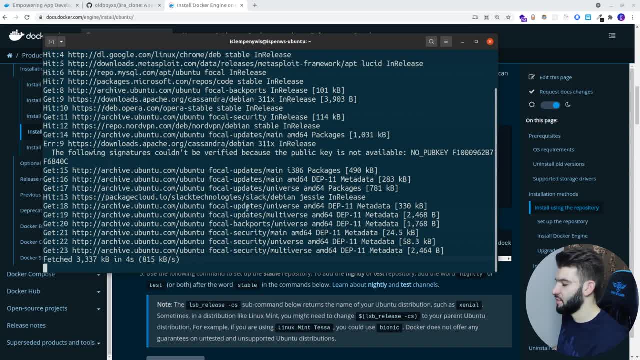 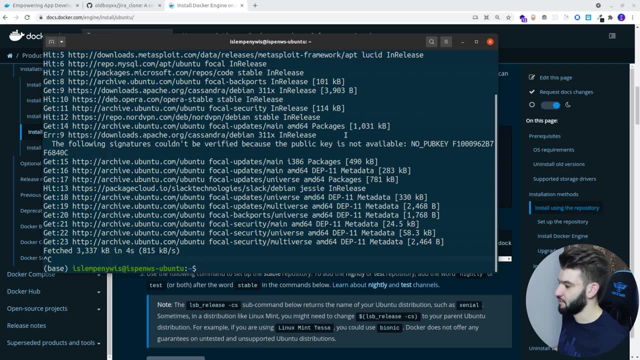 And, to be honest, I've already installed a Docker, So I don't wanna just like spend thousands of times waiting for Docker to install. this is not a tutorial about just installing docker. there's a bunch of stuff. we need to go through the tutorial. okay, so after updating here, uh, we need to go ahead and add a couple. 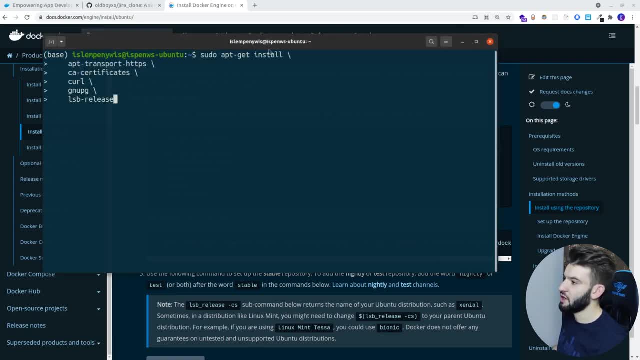 of repositories. so this command in here, which should go ahead and add um, do, apt, install, and it's going to install all of these, like the upper user support http, uh, corl or curl, cs certificates, plenty of stuff that docker is going to use underneath uh, behind the scenes. so make sure. 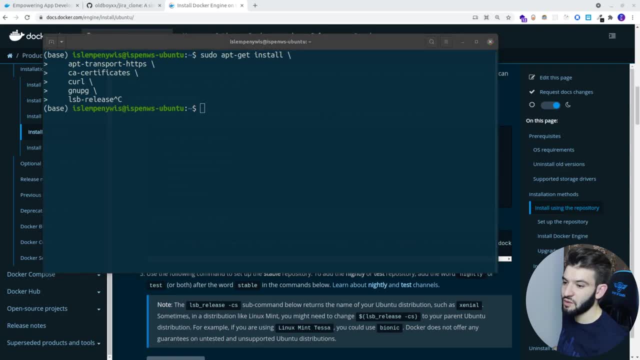 to install this properly in order to work. now, the second thing we need to actually to add docker to our like active repositories and add the gpg link, which is just like uh, for making sure that we are pretty much downloading and executing authenticated docker stuff. so nothing, nothing really. 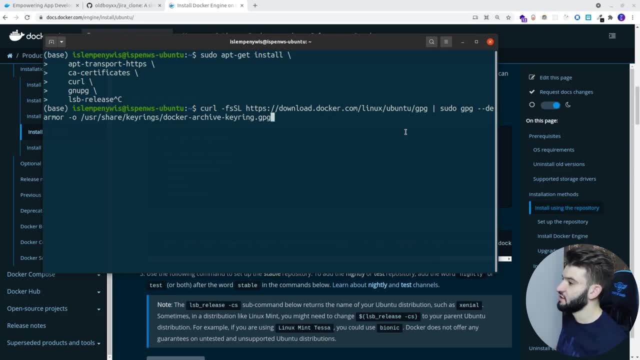 messed up or you know, uh, counterparts, something like that, parts, so just gonna just run this one and this one is gonna just like verify and make sure that, okay, you got the right version and you got the, uh, the right gpg game and you're ready to go um. next thing thing here is actually depending on the architecture, so it. 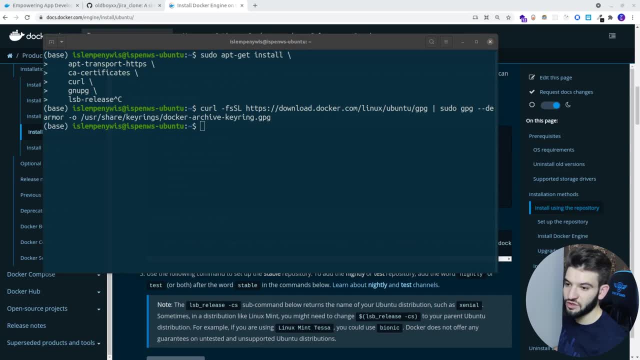 just gives you like, uh, what type of scripts you're going to be running? and of course it depends on what kind of like operating system or distribution running. so, yeah, it goes from like, if you're ubuntu or center west or debian or something like this, and yeah, so you make sure. 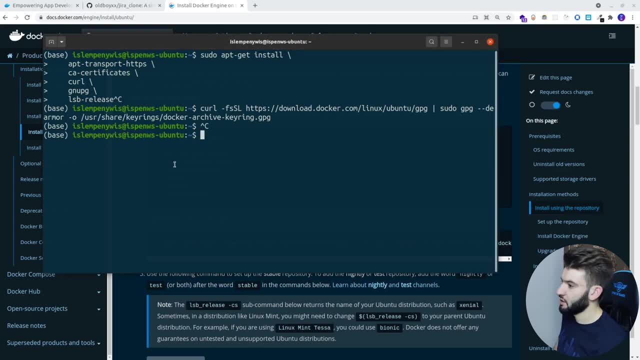 you just like you choose your own- uh kind of like- distribution in here, and this is basically just going to go ahead and do add docker to the system. and then we're going to go ahead and add docker to sources list and just download to you the docker stable release for ubuntu. so click that, enter and 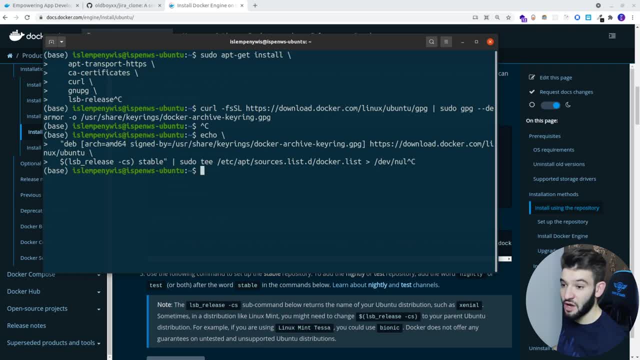 that should be done and, last but not least, what we need to do is actually run another studio update, which is going to just like update from the newly added repository that we've just added right now. so make sure to run the update and afterward what you need to do is, last but not least, is actually 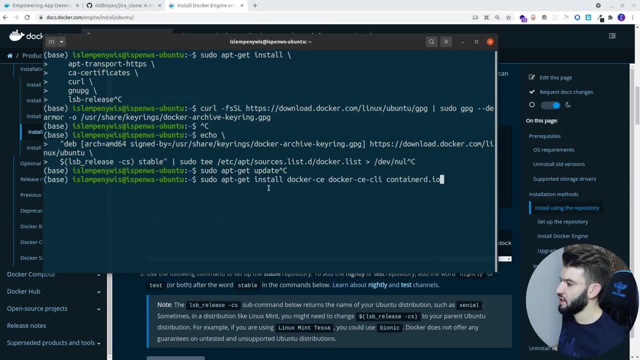 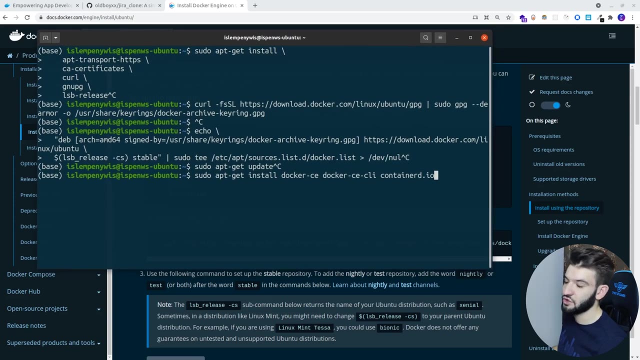 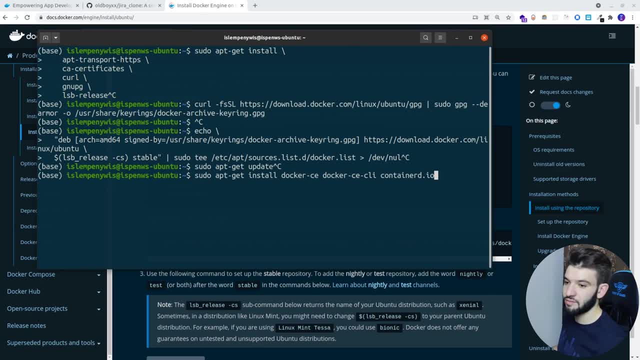 linux operating system and more specifically, into ubuntu. all right, pretty great. so that should be making it all work together in a really really good way and we should all be actually working really really well in that particular sense. so this should be all the dependencies and all the. 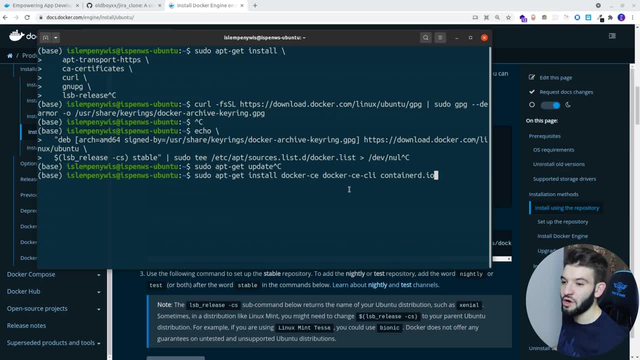 steps that you need to follow. yeah, it might kind of like differs from one operating system to the operating system or from one distribution to another. so for centralize or debian or fedora, i don't know um, it will be quite different and a little bit kind of different from that on ubuntu. 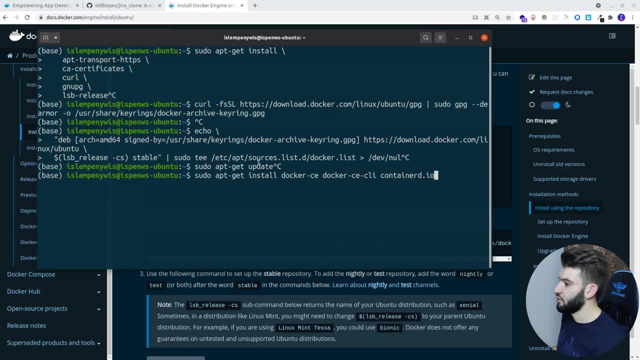 but yeah, they're still all the same. just copy pasting scripts, just putting them there, and make sure you copy the same order. you don't get like pretty messed up into that and no weird errors along the way. and yeah, you got that actually working absolutely fine, all right, pretty great. 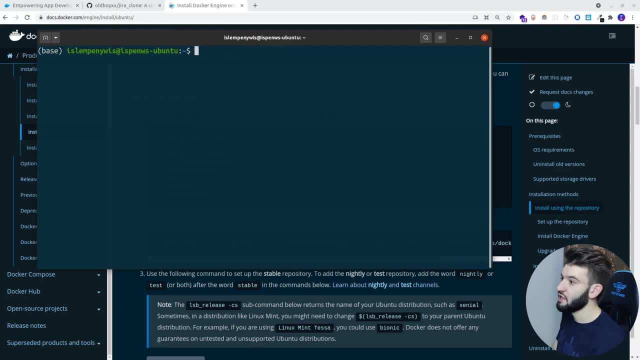 now to make sure that docker is actually installed on your machine. now you need to actually use the docker cli to run hello word, more like a simple hello word container, just to make sure that it's actually installed. so to do so, go ahead and do docker and you do run hello dash word and click enter, and this is just wait. and if you get this, 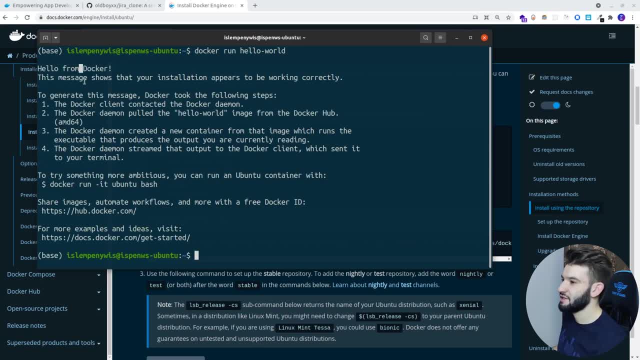 message which says: oh, hello from docker. and this message shows you that your installation appears to be working correctly. well, yes, this message indeed tells you that you've got docker installed, docker engine and docker cli pointing perfectly, with path, set it up correctly, so you get everything as you want it to be. and if you do, uh, docker, dash, dash, help, you know, of course you can. 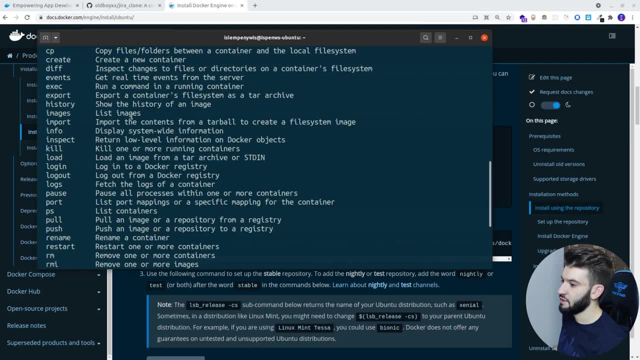 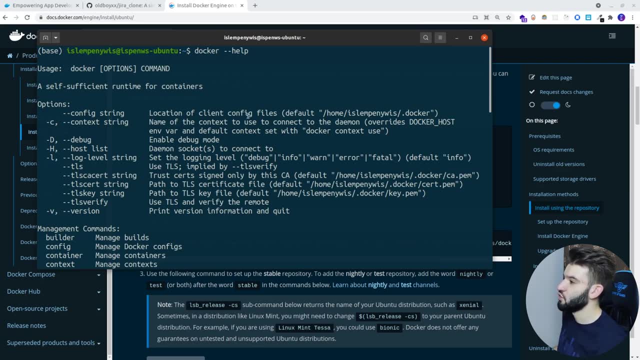 get the full help message in here and with different commands that you can use and all that sort of stuff. yo, hallelujah, pretty good, we got docker installed and everything to be running the perfect way, as we want it to be. all right, pretty sweet. now docker is actually installed. 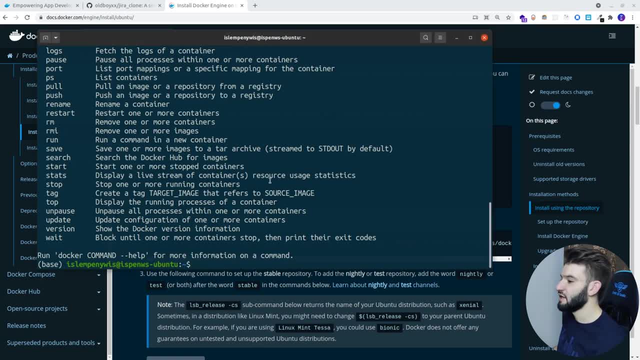 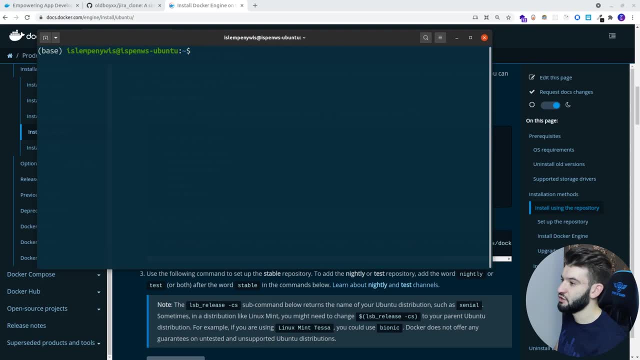 working fine, as we want it to be. all right now we run our first container as clearly see, i'm pretty sure like you're still kind of like not familiar with docker containers and how they won. yes, we're still going to go into details about this and how they work all right now, the most. 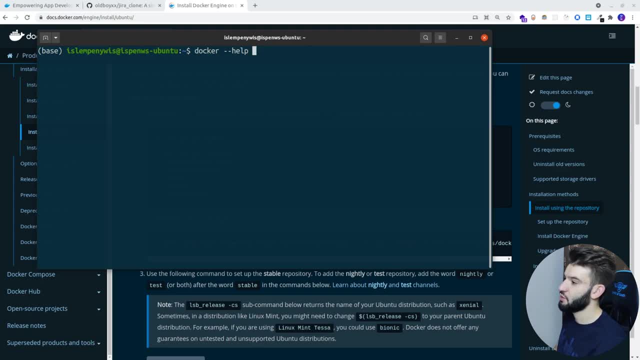 basic docker commands. of course, what you can, how you can learn them, is actually throughout the cli. so the docker cli is this is how you access it, and i said before, the docker cli is already added into your path, and what i mean by this is a path is pretty much like um, an environment variable that tells 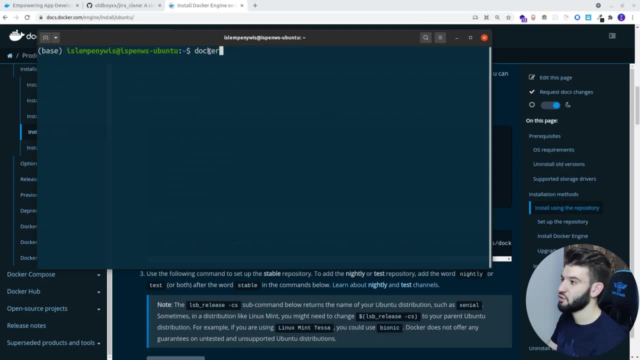 linux more specifically if it's available on windows and mac as well. but i'm talking only like this perspective. so path is just like: tells it where to look for binaries. to uh, pretty much execute them and docker in here, of course, is going to be putting on our like. 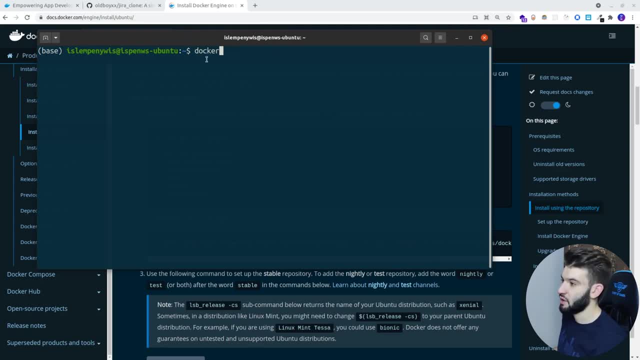 local user binary or something, and yeah, it knows exactly how to run that. so, just like, by typing docker, it's going to go in and search for the binaries. it's going to find you know, a binary, this name you put in here, docker, and it's going to execute it. for us, that simple. so this is why. 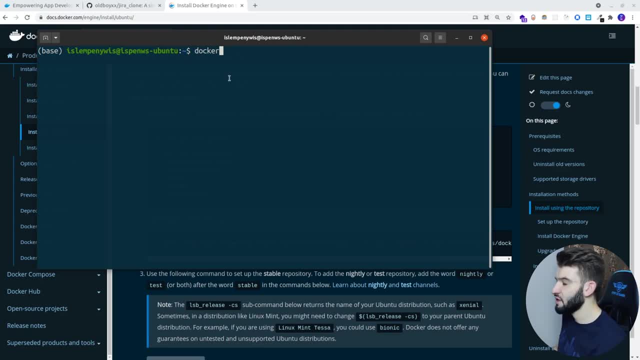 the cli here is is actually working for us this way. now. the second thing you need to notice is actually the cli is pretty much the client now behind the scenes: docker. so as soon as you install docker, there's this like docker demon or docker d. so this docker demon, what it does. 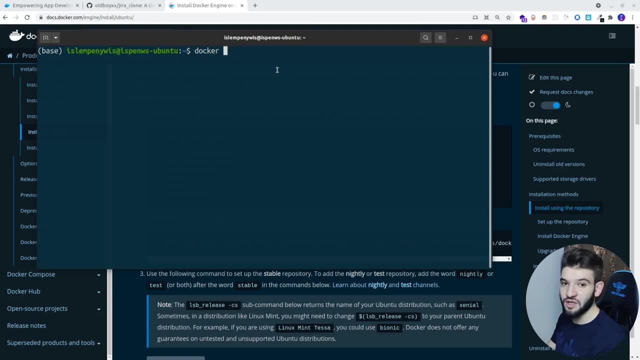 is pretty much always running in the background. so as soon as you install it on your machine, it's always up and running. so whether you restart your machine, uh, you log off and you log back in, whatever it always is going to start the docker engine behind the scene, it's always going to be. 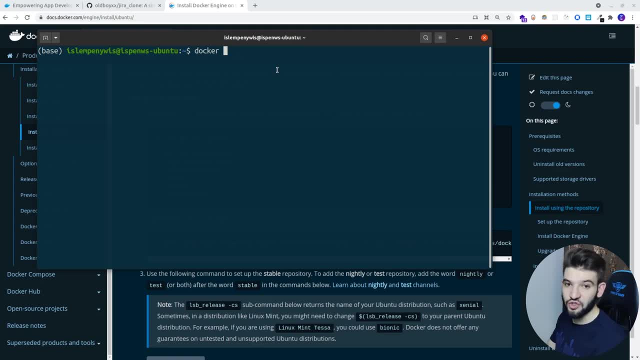 in the background running somewhere, and this docker daemon is pretty much like the server of docker that is going to control everything from containers installing images, controlling how virtualization works, how to handle os operating system, kind of like level isolation- and all the sort of stuff that docker's needs to be taken care of really, really well. so yeah, so this is. 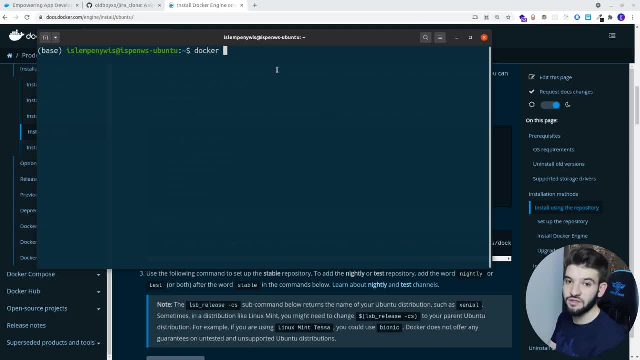 the docker client and for the docker client in that particular part, what it does. so as soon as you give it a command, this command is going to be sent to the docker daemon and the docker daemon is going to, like you know, do some handling some low level stuff on the linux, or linux kind of like. 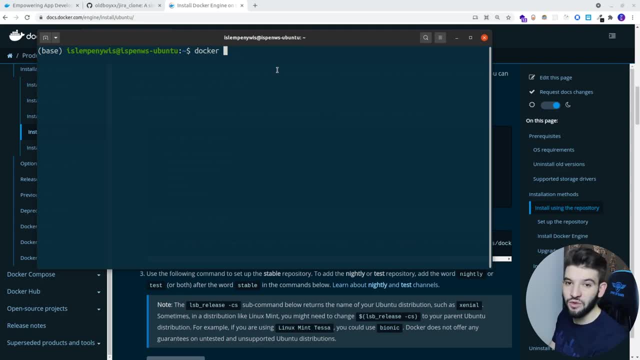 operating system really low level and it gets back with a response to the docker client. then the docker client shows it up, uh, in the cl line. here you the terminal and it shows it like shows a really friendly message for us. so this is basically the simplest architecture of how docker actually works and operates behind the scenes. so just for you, 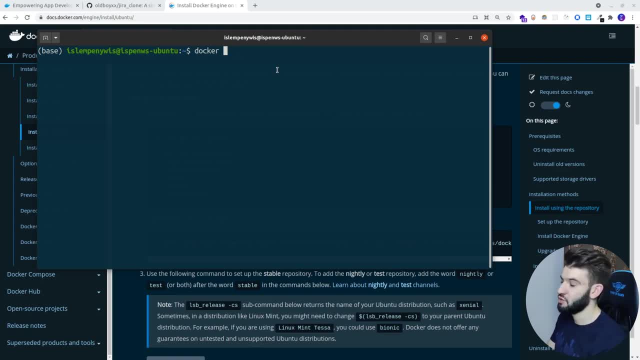 guys. uh, to get a grasp of how docker actually works and to be able to know exactly how docker is manipulating all of its commands, all right, so yeah, as i said before, this is docker cli and this is what you're going to be using for pretty much accessing everything, for doing any kind 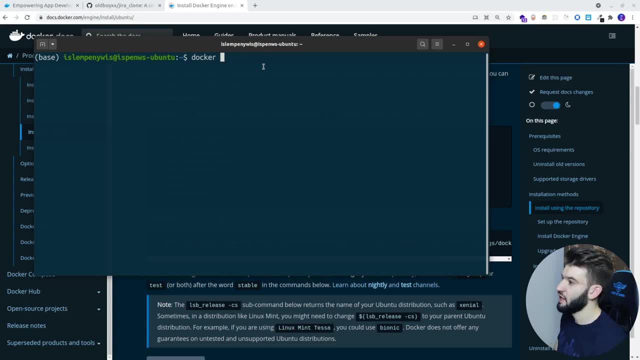 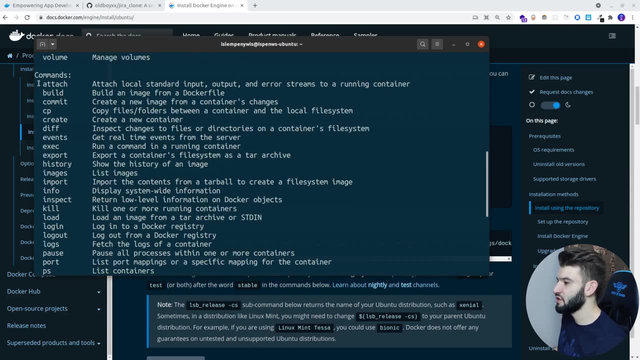 of command for running containers, stopping them and everything, and the docker command in here. if you do help, you're going to have a bunch of commands listed in here, and what i like personally about this cli- the docker cli- is actually it gives you a pretty well, uh, descriptive messages of commands. 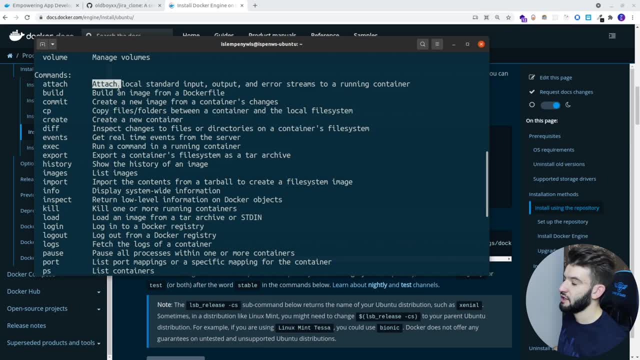 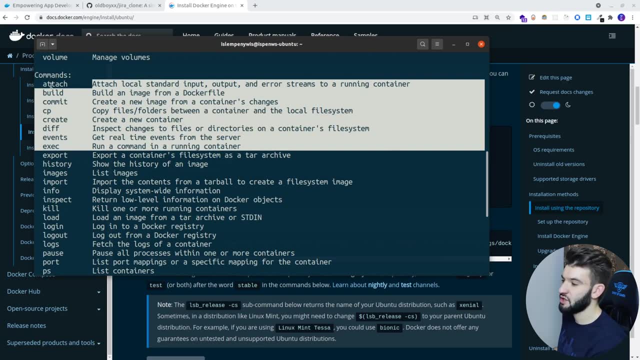 and what they do, for example, for the attach that does like attach local standard input into an output and an airstream to the running container. so you just like, by looking into this command and read through this like command and you're going to be able to see what's going on in the docker. 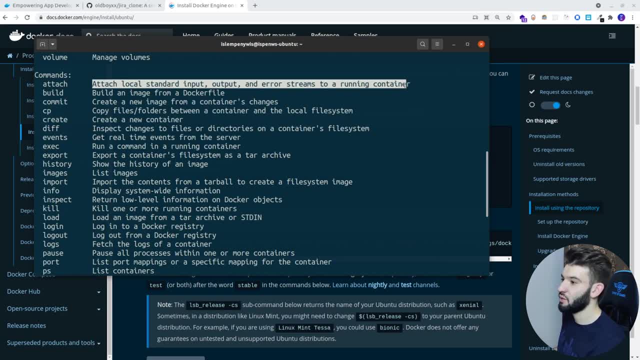 and you're going to be able to see what's going on in the docker simple one line description. you know exactly what this is doing and, yeah, you're just like, oh, this is doing this, all right, that's good, i'm going to use this command so, without just going. 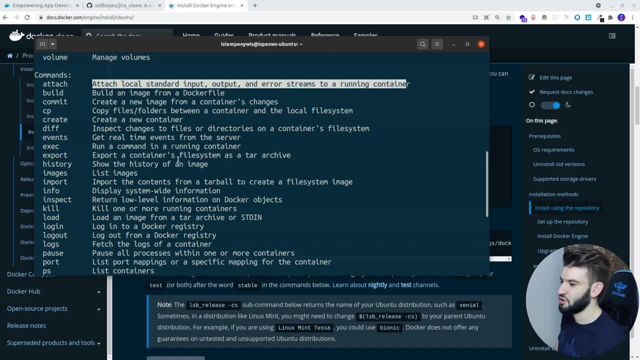 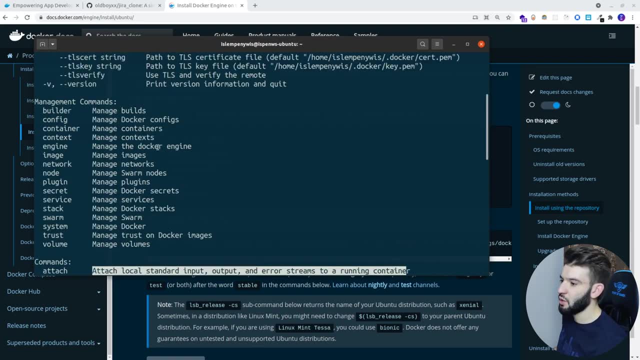 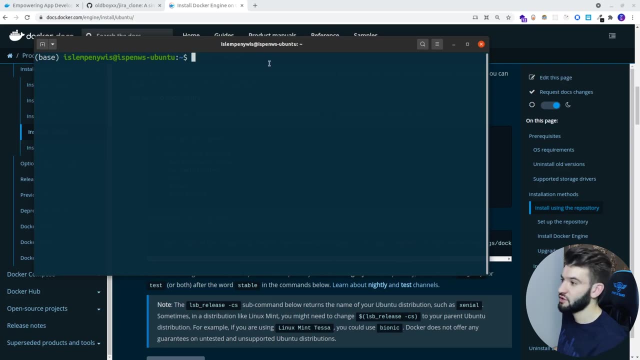 and looking into google, stack overflow or even the docs, which kind of like awful to do all the time, especially for us as developers. all right, so this is pretty much the whole commands. now there's a bunch of commands that you're going to be using throughout. i'm going to be using pretty much more than the others, and the most standard and common 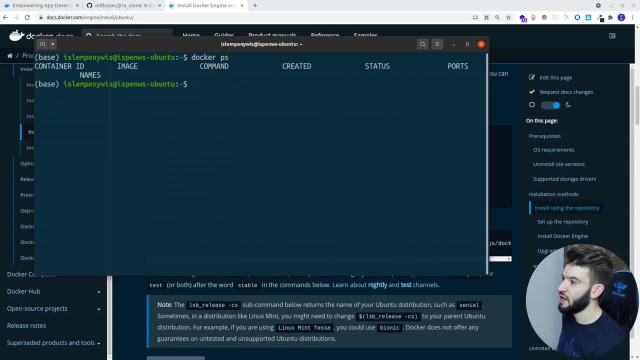 commands that are going to be needed, for example, is the docker ps, and this one stands for process status, which is going to give you, like the currently running containers that are currently uh, running on the docker engine. right now, there's no docker containers running, they're all stopped. 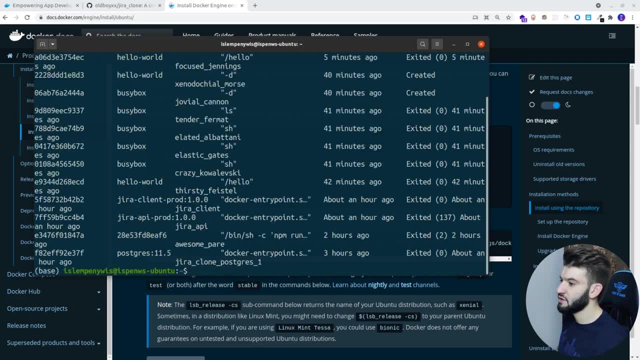 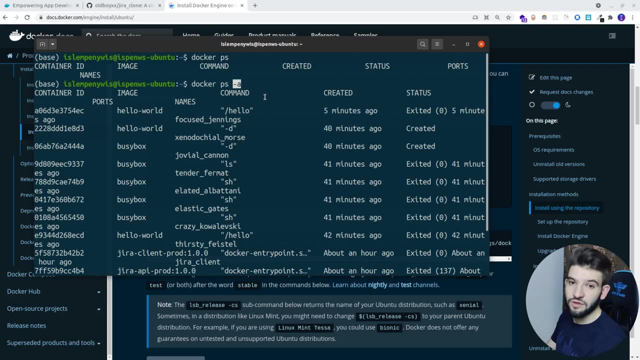 and, if you do like, docker dash a, which shows you all the containers- excuse me, there's a bunch of them- and this a, a flag in here, where it does just like shows you all the all the type of standards of containers, which is what i'm going to be using today. so if you're looking for a container, that's. 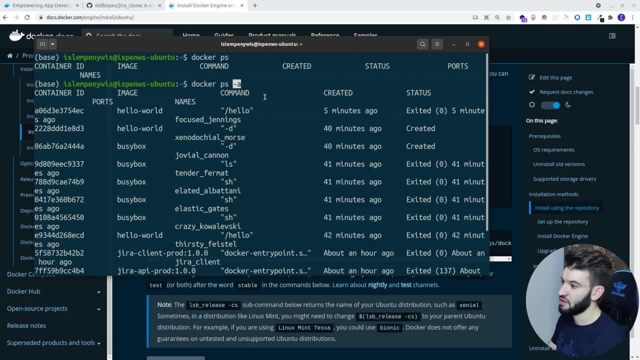 whether it's stopped or whether it started. it shows you that and as clearly all of these containers are stopped. uh, if you see this like hello word that we started it just like five minutes ago. it stopped right now to exit it. uh, just like after zero seconds and five minutes ago. 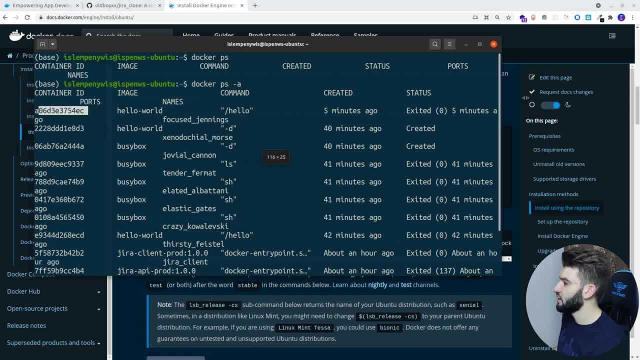 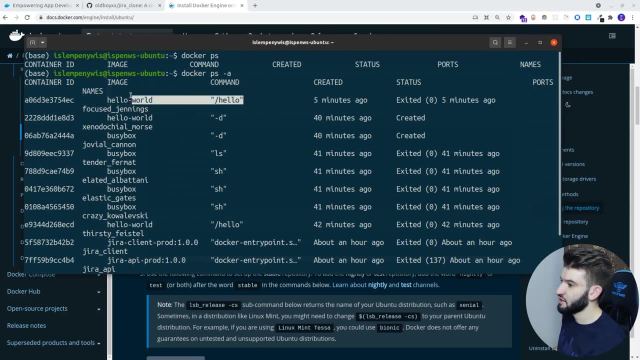 and it gives you, like, the container id and, yeah, it gives you like this basic information. i'm just gonna, you know, give you a little bit more uh space in here to see what exactly happening behind the scenes. so, yes, clearly this is pretty much. it gives you like, uh, some kind of descriptive. 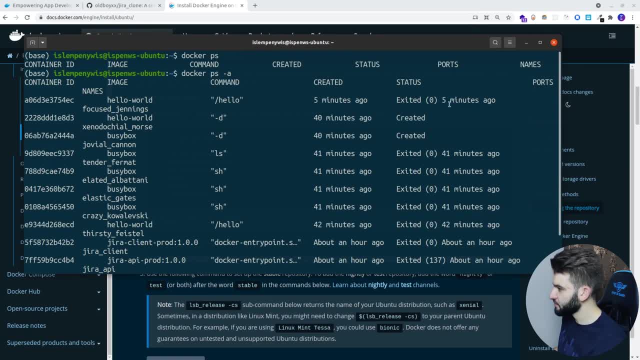 of what is happening behind the scenes and and stuff like that. as you see, it looks pretty, pretty great and it gives you the whole repositories, or pretty much the containers that are already stopped, because i use this a flag. okay, so this is just basically for the ps or process status. 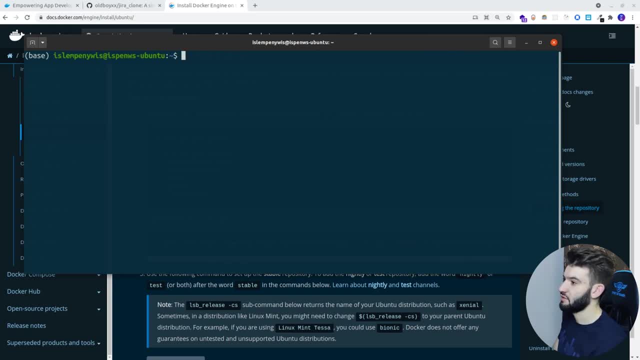 because we don't have any kind of docker container currently running or something from that sort. now, the other other cool command and that you're going to be using a lot is pretty much to check your images, and if you do like docker images, you're going to be using a lot is pretty much to check your images. with an s at the end, you click. 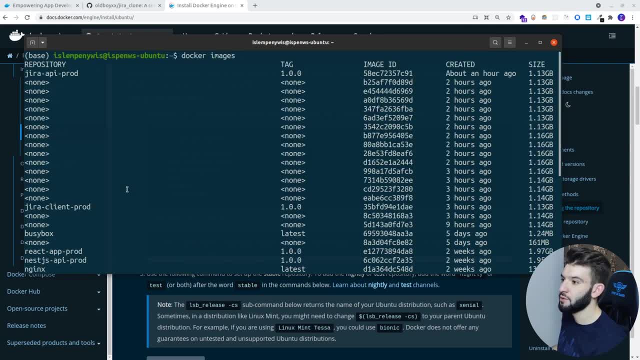 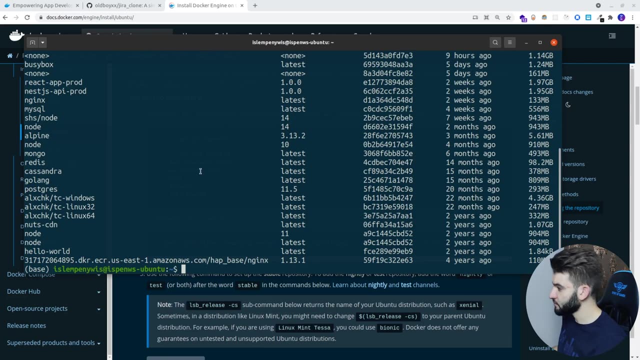 it and it's going to give you the full list of images available on your system, of course, so you can have images downloaded and pulled down into your system at any time or built from you know your own uh kind of applications all the time, or what you can have. it's pretty much like just. 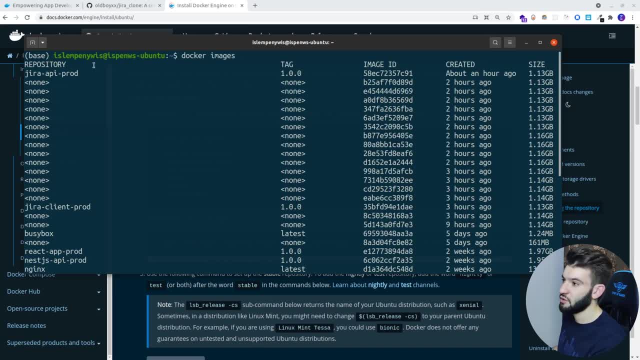 pulling images from from the kind of like repositories, and the most common repository to pull images from is actually the docker registry or the docker hub, which has mostly- uh, the free or output source kind of like images or even private images. you can host them there or whatever. so this is pretty much the full list of images you've got on your 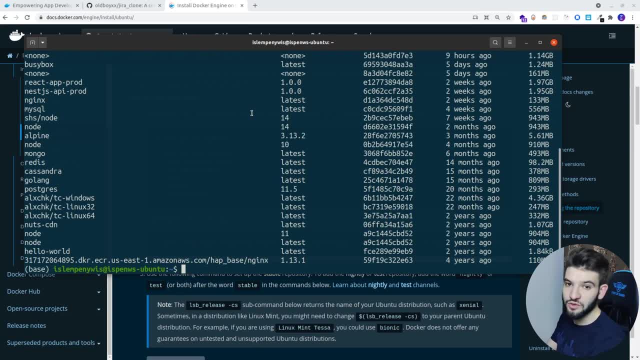 own local machines and what i mean by images? pretty much like a built kind of like container which is just an image and it's. it's not like a running container or something like that, it's just like image sits down there and it has all the instructions abstracted. so docker later on, if you. 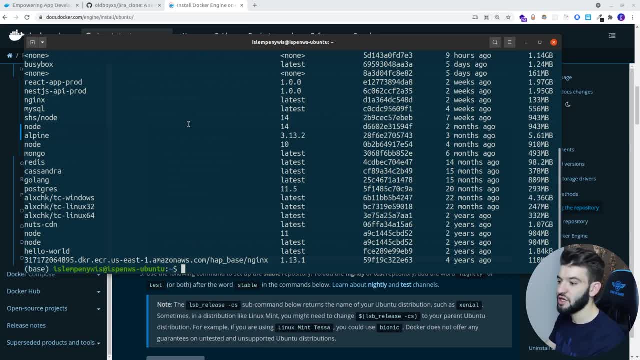 want this image what it does. it takes this like kind of like image, just like this, this kind of like a small image, and it puts it inside of like a container, where the container is pretty much more like a small manipulated linux container and you can think of a like a separate operating system. 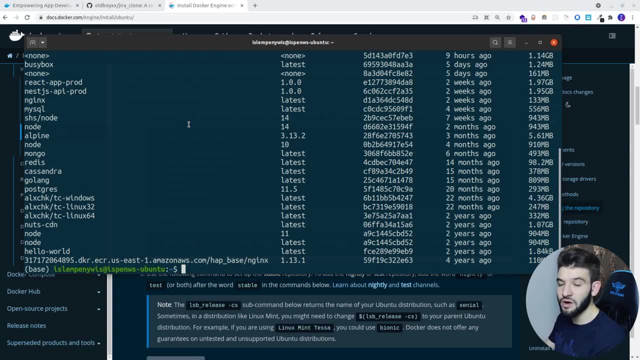 like a separate machine on itself. so if you're familiar with vmware or virtual box or uh, virtualization in general, so this is what it does. it just gives you like the full. it allows you to run multiple operating systems on a single operating system. so this is kind of like what. 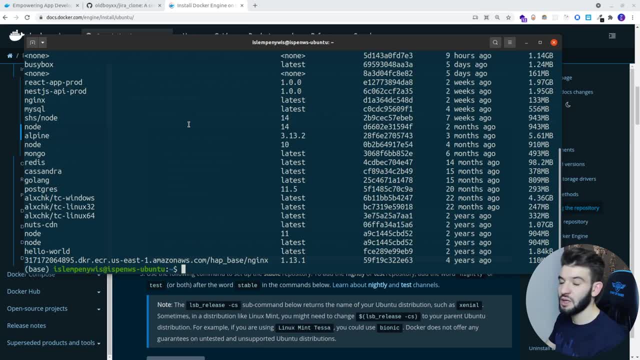 docker does, but it's not doing virtualization in in low level or like uh for type one and type two operate virtualizations anyway, but what it's doing is doing like os kind of os level virtualization, which is uh kind of really really speedy, really quick and really performing. that's why docker is. 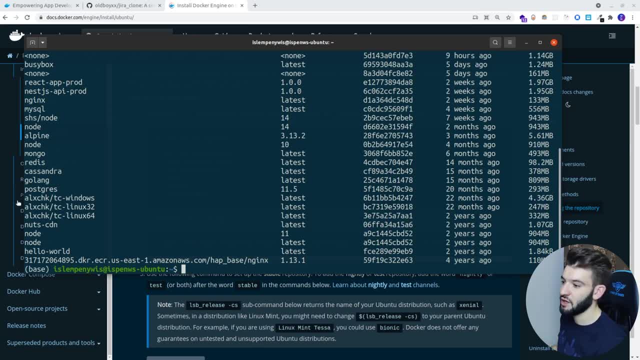 really preferred in this field- and of having containers and running uh applications. just like a couple of seconds, just like less than a couple of seconds, that allows them to run these images. so this is basically what it does and this is why we have images in here. so if you've got for 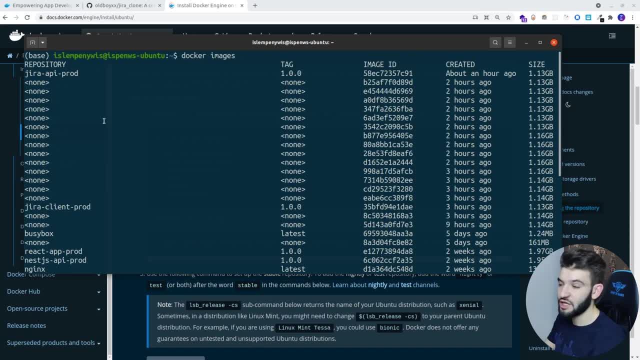 example, like a source code: uh, which is your application. so first what you need is pretty much go ahead and create, like some configuration file to tell docker how it's going to build this image. now, after creating the configuration file, you're going to tell: oh, i got this. 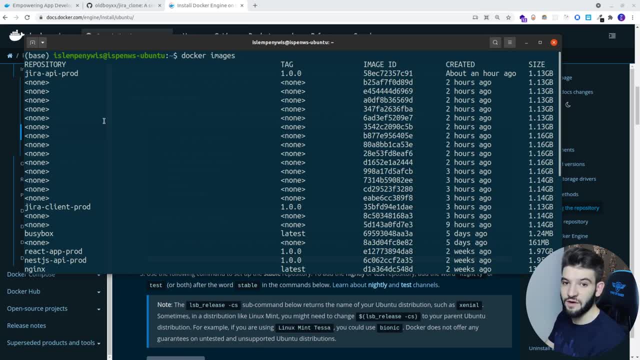 configuration file. now, docker, go ahead and pick this config file and build me this image, which is my own personal application image, and this image has all the source code, all the commands, everything that you need to run the actual application now, after that, you can take this image, you can distribute it, you can. 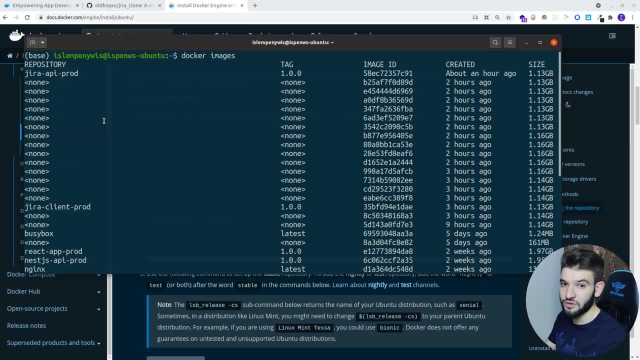 you can put it on the docker hub. you can even have your own registry hosted on your server or other kind of like third-party servers and afterward you got this image. you can. you can have this image distributed throughout the whole team um like with all the third-party teams. 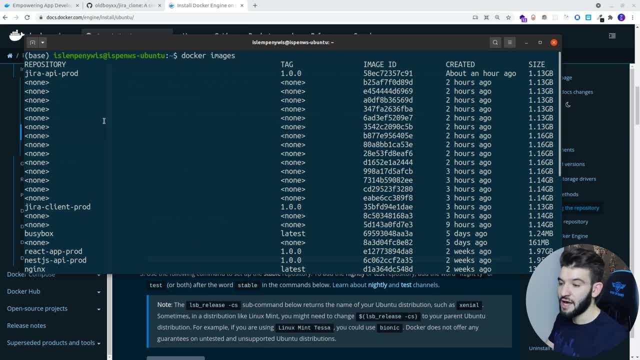 whatever, now, this image can be pulled down by anybody and as soon as they pull it down, they can just, like do docker, run this image, which is going to run the image inside of a container, and this container is going to be a live container. that's going to be like a live, small operating. 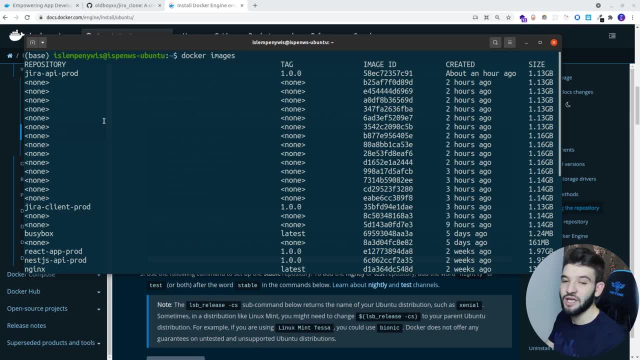 system running linux and running this specific image and this specific image only. nothing more, nothing less. just this image running, and it has all the data, all the info, all the commands and all code needed to run this image specifically as you configure it to be. so this is, this is basically. 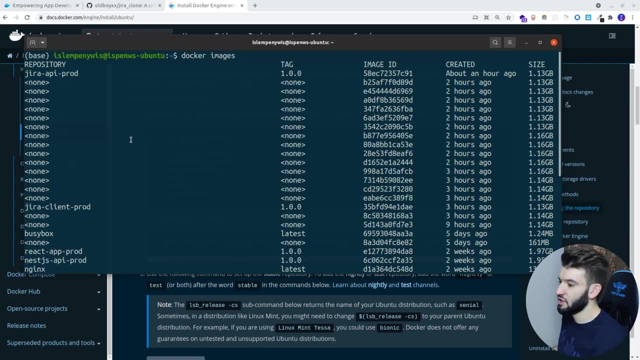 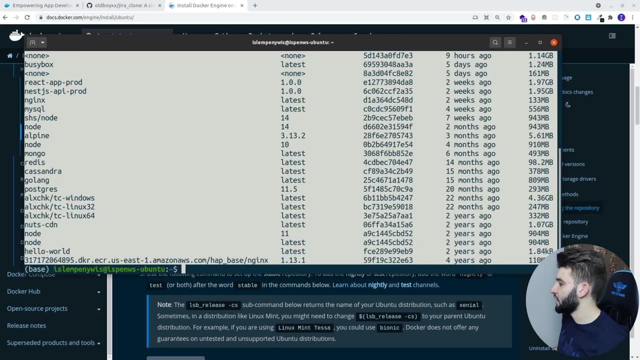 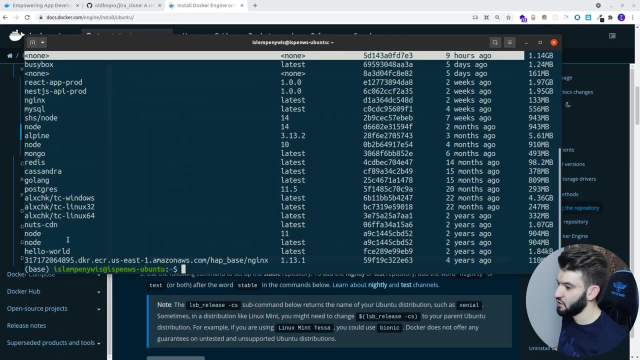 what images are and this is how, uh, they basically work. let's close in here: as i said before, we got this old image. as you see, they are ridiculously uh when it comes to, like, um, you know, space, and this is mainly because i'm using, uh, more like nodejs, and nodejs images is kind of huge. so 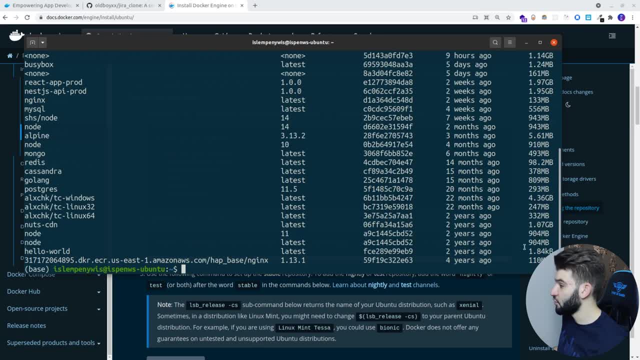 take a look on this. this is node image which is 904 megabytes, almost a gig. and if you add on top of it your own kind of like source code or your own application running on top of node, yes, this is going to be added up and that's why you see, uh, this, this huge size in here. 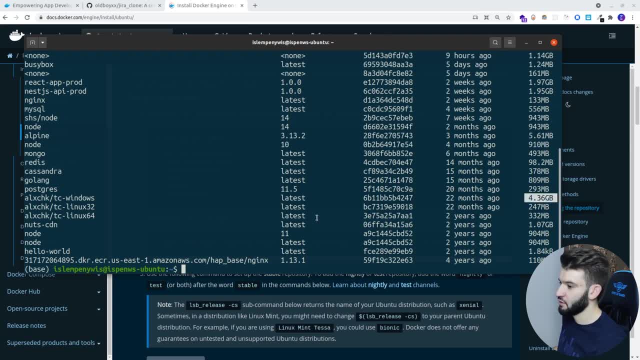 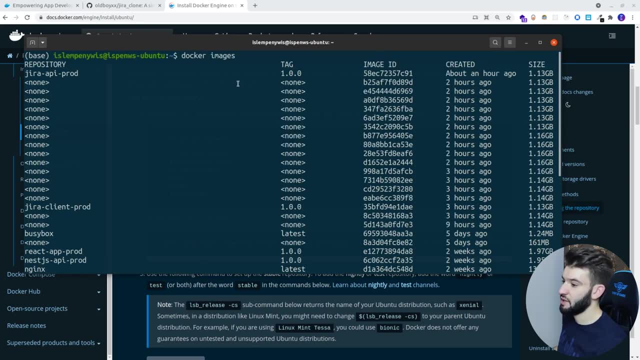 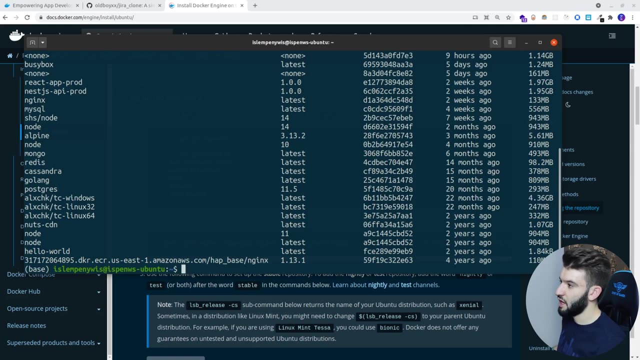 for more, like one gigs and and up, uh, even here like four gigs and all that sort of stuff. so yeah, um, i mean this, this way of doing docker is really well and images plays a really major role. now, what you can do as well, uh, there's an alias command for this, so this you can do. image ls for. 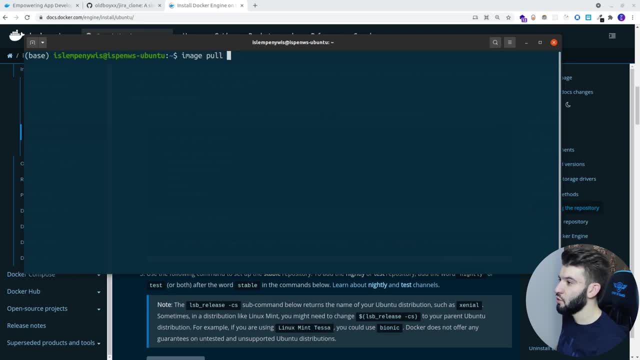 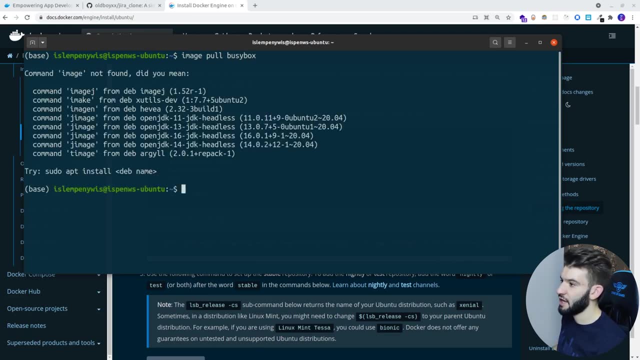 image, ls doesn't really matter, and you can what you. of course, there's another command called pull, and this command allows you to pull a specific image. for example, it's going to pull the busy box image and um. so yeah, sorry, i haven't done it right, so you can do like. 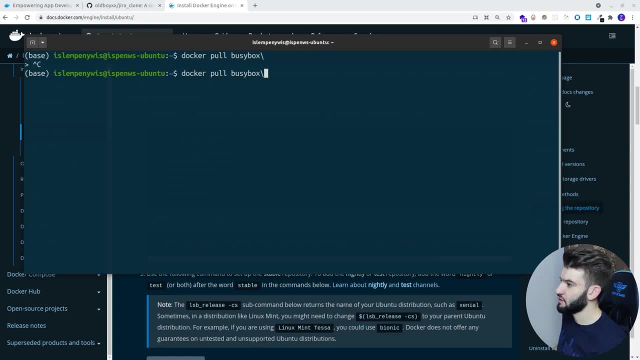 pull busy box and there is actually a busy box. okay, i can't type properly. uh, this busy box image is actually setting up on the docker registry. and what this busy box just does? it just emulates, or pretty much like simulates, a small kind of like unix uh operating system that just 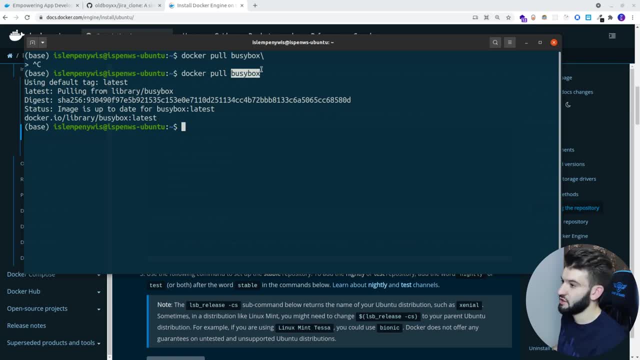 pretty much provides you with unix commands like: so yeah, just a small container there to do it and it's crazy. i already pulled that out and it already like pulling the latest from library busy box and images up to date. so i already got that on my host machine. this gives you all the information. 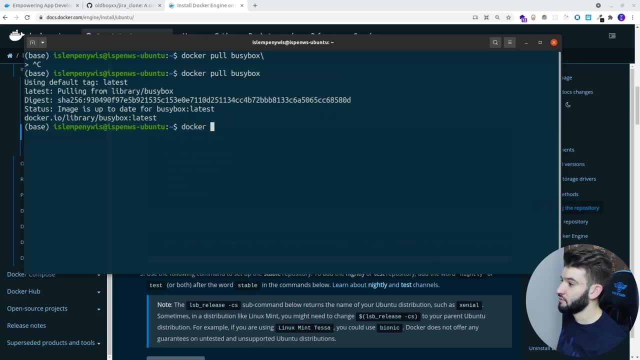 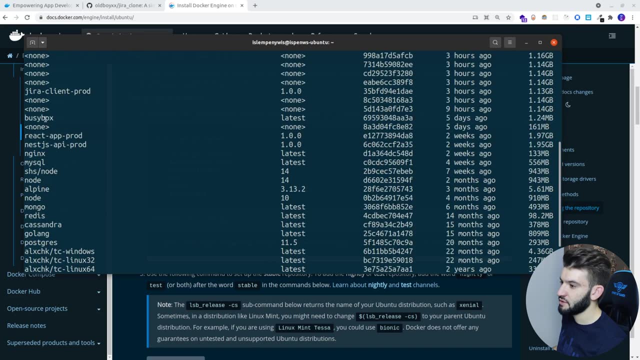 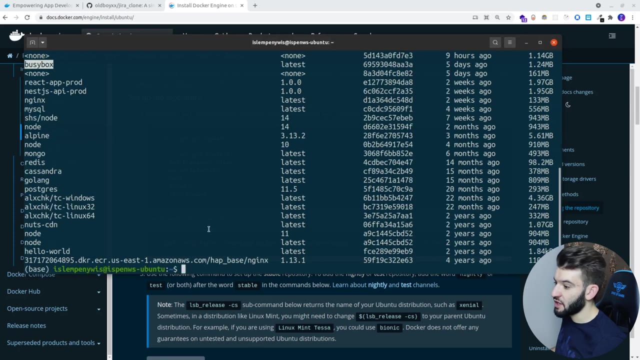 you need, which is pretty great. and if you do something like um docker images and you're gonna use a little bit of this image, you can also use the busy box image. so if you take a look, um, where is that? so there you go. we got busy box right over there and you can now use this image. 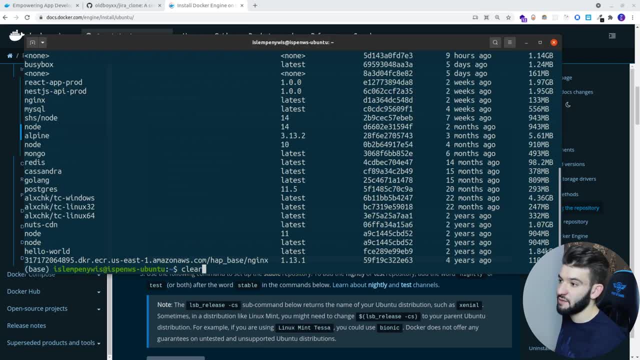 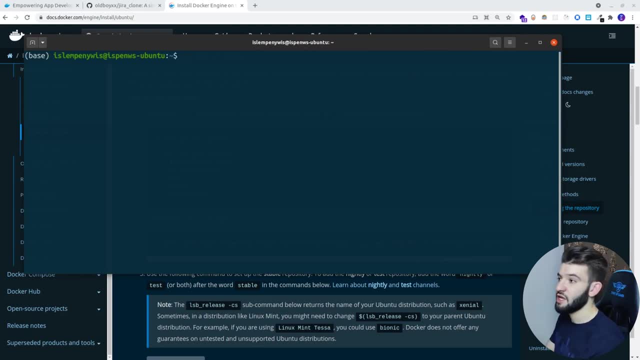 more particularly this busy box image and run it as a container. now it's just like a sitting frozen kind of image, just like sitting there doing nothing. now you need to run, use like run this container with, or pretty much run this image in order for it to convert it to a container. 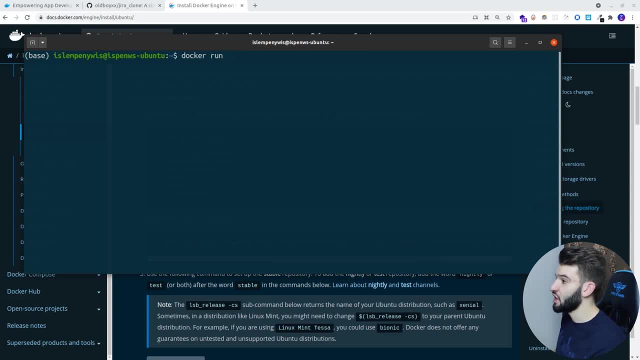 and be alive and work, pretty much. so. to do so, you can use the run command, which is, of course, another very important command. And this command, what it does just like runs you a particular image. I mean it just like runs it inside of a container. 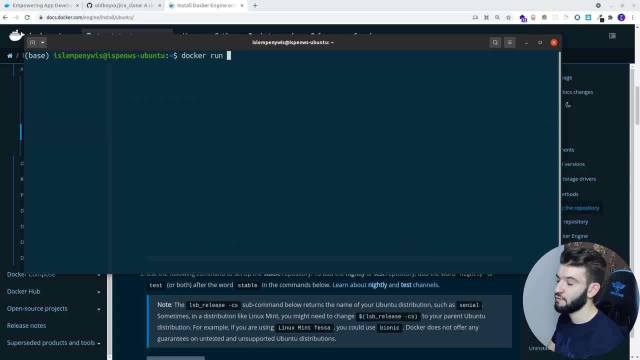 and you give it like a bunch of like flags on how to control that, For example, if you want to control ports or to control volumes or all that sort of stuff. we're going to be seeing this later on as we go a little bit advanced into Dockerizing a full application. 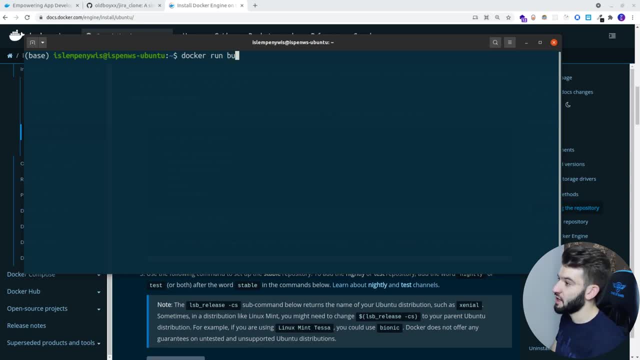 But for now I'm just going to use a busy box command, So I'm going to run it bare busy box. okay, So I'm going to do run busy box and you're provided with the image name. More specifically, if you want to like use a specific tag. 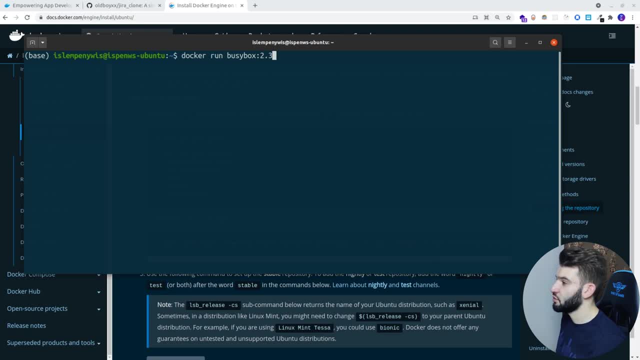 for example, you got a busy box version 2.3 or something or you want to use the latest version of busy box. you can do it this way, Mainly if you just like ignore that it's going to use the latest version. 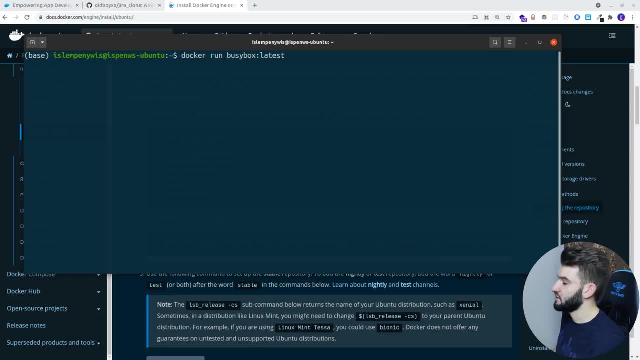 or if you provide that, that will be good as well. Belt, yeah, so that would be good. So just do a Docker, run busy box and this is going to take us through. you see, it's really really easy, It's pretty fast. 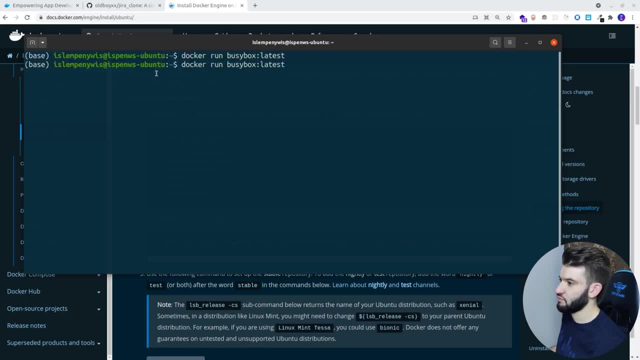 You see like how responsive it is to run it. It takes like two, three, five seconds or something just to run the Docker container. So what it's doing in here behind the scenes it's running or starting the Docker container. It's pretty much like handling some kind of stuff. 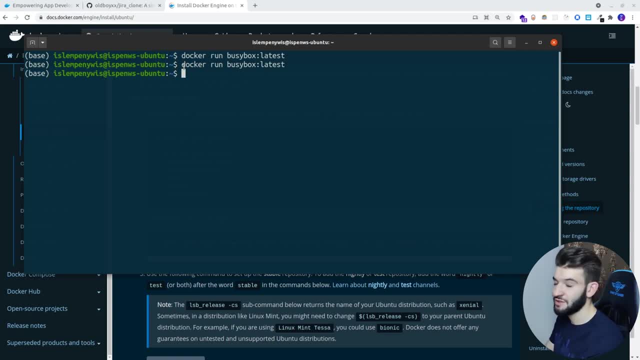 inside of the container, Then it's stopping the container. So this is all of it taking like five seconds. Imagine if you did this particular step on an actual virtual machine or like in virtualization, how many, how many kind of seconds this is going to take. 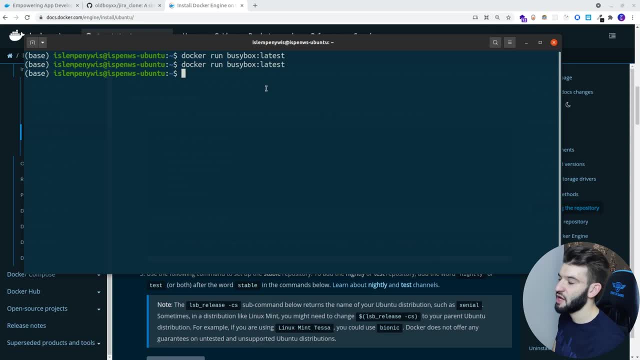 It's going to take a ridiculous amount of time, Like, at least I would say, five minutes or something, which is kind of a moments when it comes to development and deployment and all those sorts of stuff. So the busy box in here, what it does, it does nothing right. 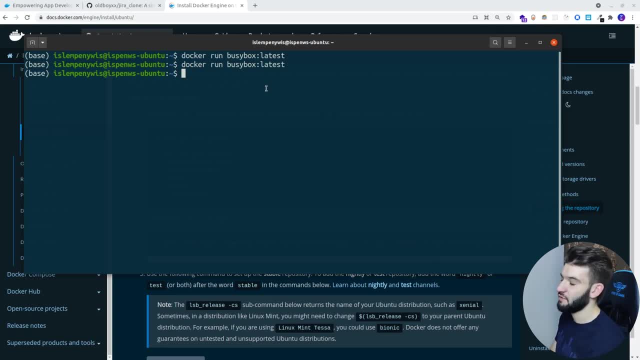 This is just a study alone, basic kind of image that's going to just like run. as I said before, you provide it with particular command. a Unix command is going to run it. So, for example, what we can have, for example I'm going to say, oh, you go ahead. 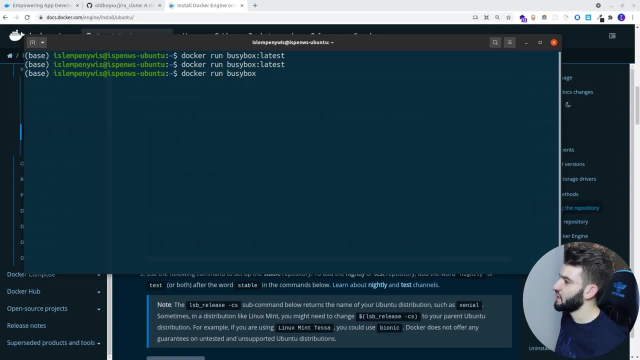 and I don't like this latest. let's go ahead and get rid of it. So I'm going to say, oh, run me this LS, And if you take a look on it, what it's going to print? it's going to print this LS. 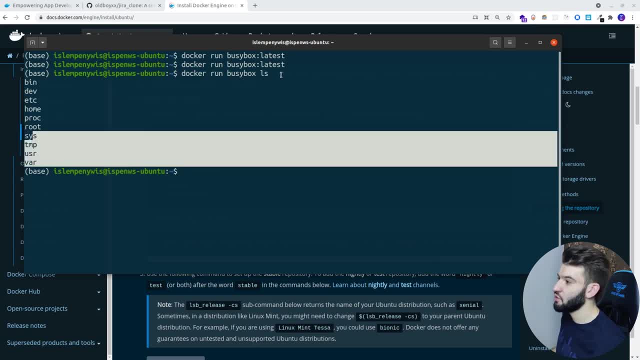 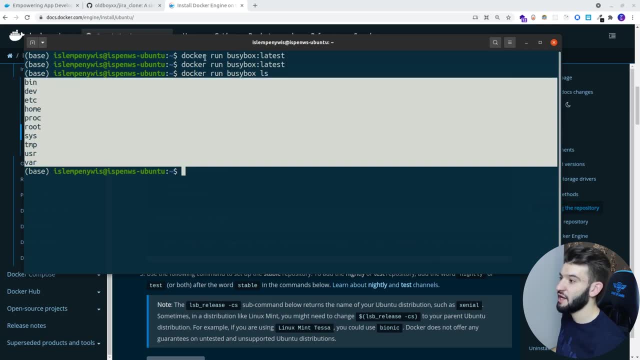 And indeed this is not my machine. This is actually. it's going to do a list, It's going to do LS command inside of the busy box container. it's going to create which is going to print me this And instead of the busy box, 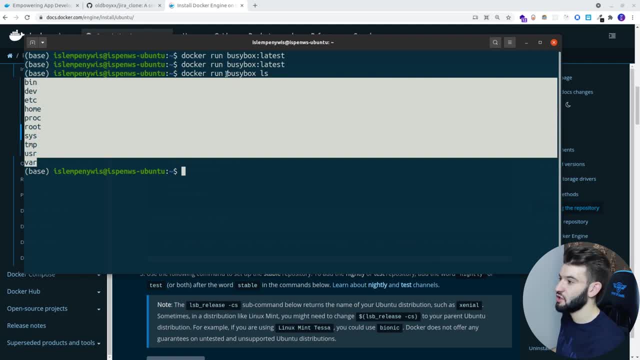 indeed is going to be the Linux distribution or the Linux Docker container running there, with a busy box image in there running, And this is what it's printing me. So, indeed, this is actually what's happening. We can, for example, do LS, and I want oh. 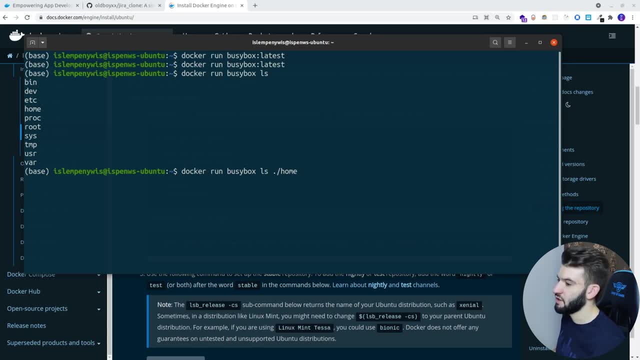 I want to go ahead and see home if it does have anything, And luckily I don't think home does have anything. So yeah, you can see that there's another, for example for Ben. we can just take a look what binaries is available. 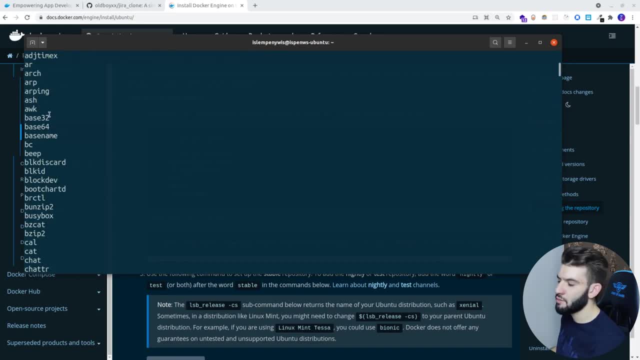 And there's just like basic binaries that is provided with bare minimum Linux distributions And this is like what binaries it has in there. Basically it's based on Debian or Debian, sorry, And yeah, you can use like commands, like everybody gets, and everybody get update. 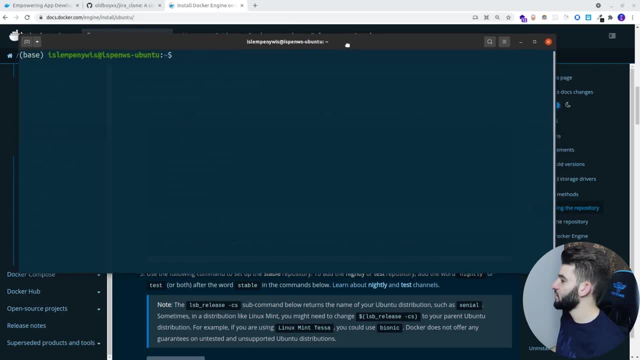 to install different packages in that particular sense, All right. So yeah, that's a that's pretty good on how to run in basic stuff in this and how to run kind of like basic commands or basic containers on Docker and using it this way. 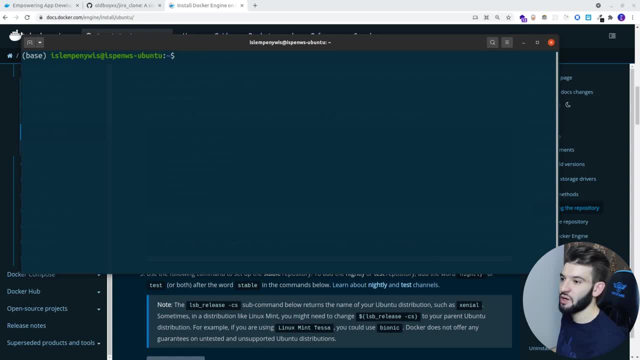 So that should be. that should be pretty simple. There's actually another thing we want to like go ahead and run, for example. So let's say I want to run the Postgres kind of SQL or Postgres DB using Docker. So in this particular sense, 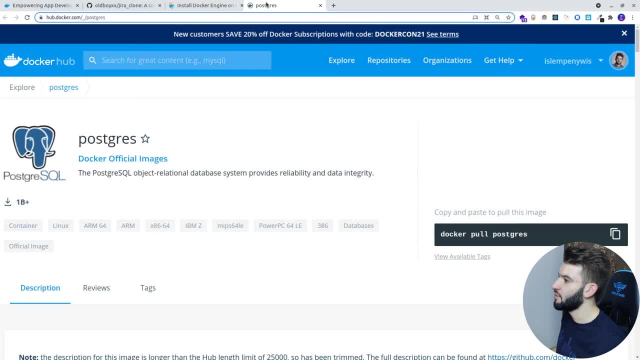 I'm going to have this image in here for my Docker hub, So let me just point you to this. So if you're sitting in, this is the Docker hub, So it's called hubdockercom And this is where most of the images 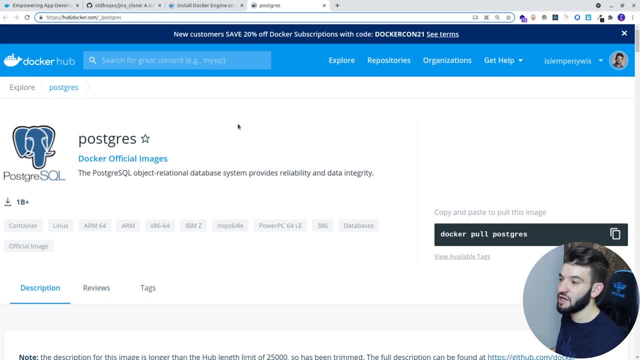 where most of the Docker images already created, an already pushed up images are actually live. So this is the Docker hub And those aren't shady like some official open source images that you can find, of course, for Postgres and stuff like that. 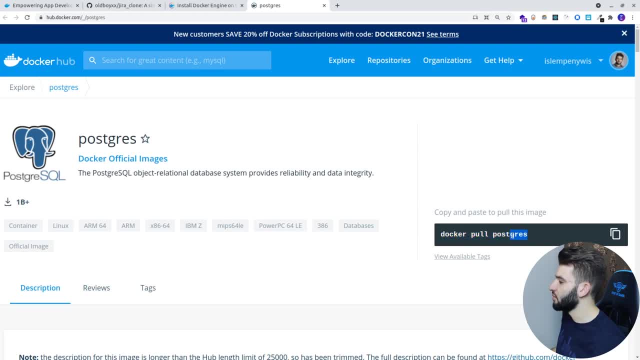 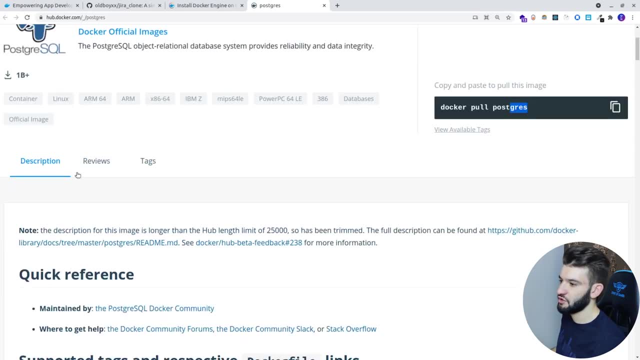 And you can only, all you need to do- just go in and do like Docker pull Postgres and you're going to get this particular version And you're going to get have like particular stuff, like description And inside of description. 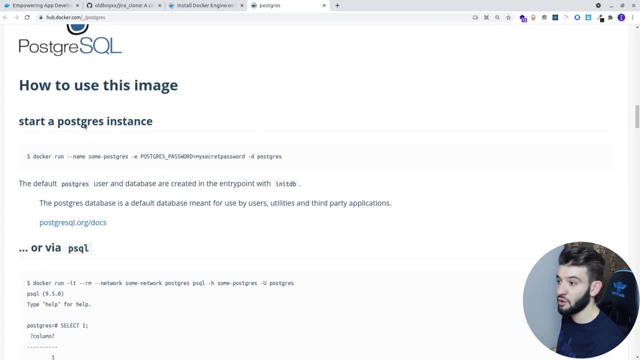 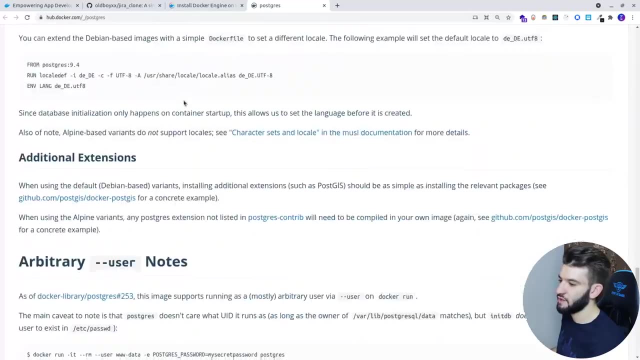 you're going to find, like some version in quick reference, what it does, how to run it, basically like what commands you need to take a look on how to use it, for example, with docker, compose and plenty of stuff like information and how to run this and. 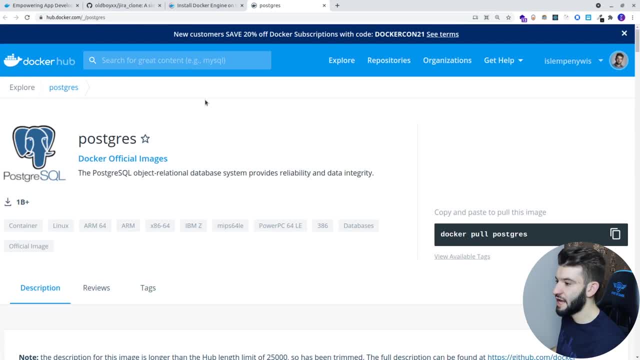 environment, variables and configuration, all sort of stuff. so it has everything you need to pretty much run pretty much this image and like put it out and start working with its own locally. and why not use docker files or extend this image and use it to pretty much work with your application or use it throughout docker? 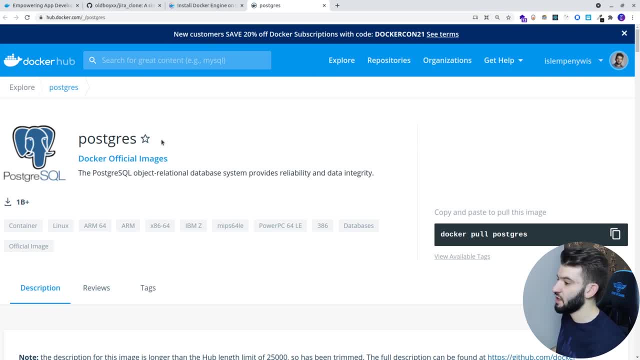 compose alongside other services or something like that. so that is all available throughout the docker hub. so let's go ahead and see- I'm gonna run this docker Postgres sequel throughout the docker command and run it and see what's actually gonna happen. so let's say when it's like start up this. 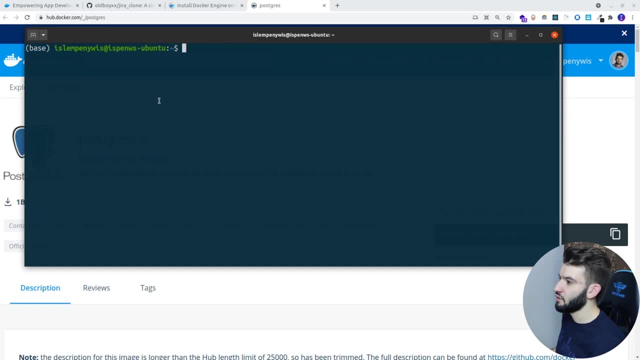 Postgres sequel server luckily in here. so for this I want to go ahead and do docker run, or what you want to first do is actually go ahead and do docker, pull Postgres and you can specify a version, for example a 11.5 or something, and for 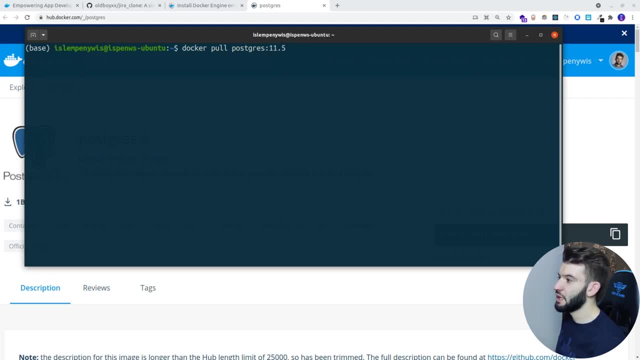 some reason I'm choosing 11.5 in this particular video because latest versions, like 12 and 13, are not basically working, with no GS connection and with no GS project. so there's some really weird error that's happening behind the scenes. that's why I'm falling back to this version, which seems safer and it seems 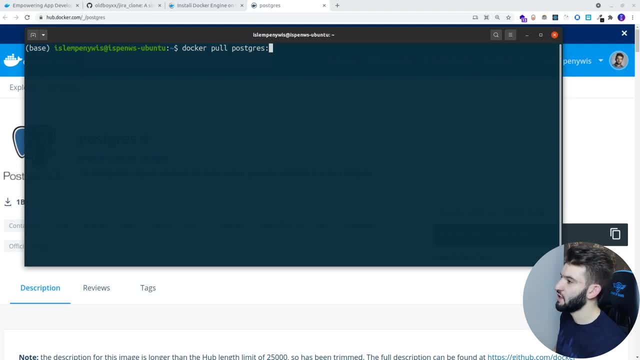 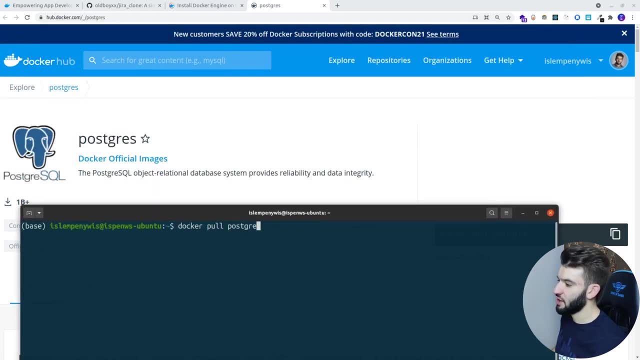 working perfectly. so just like a quick notice about why I'm using this. so just docker, pull and it's going to pull the latest available version on this hub. or what you can do is actually go ahead and like: run docker, run directly and docker is going to be smart enough if it doesn't. 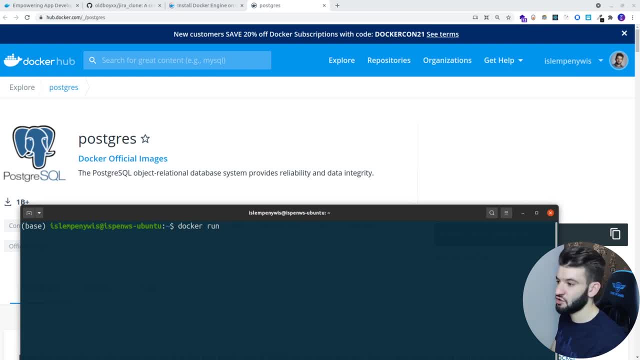 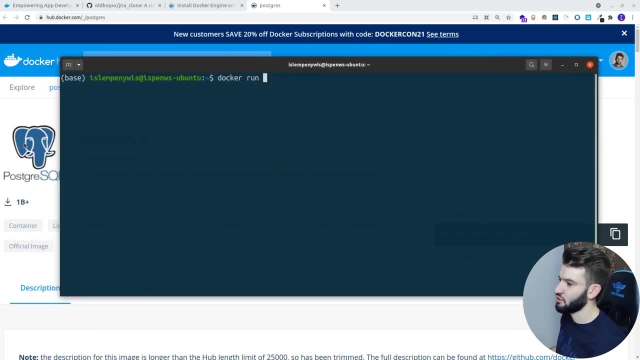 find the actual image in your own machine. it's going to try to pull it first, then to run the Postgres, so make sure to do it anyway, uh, the way you like it, of course, to make sure to run it this way. so if you take a look on the 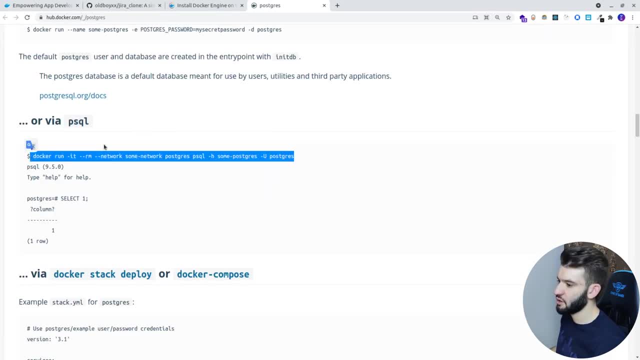 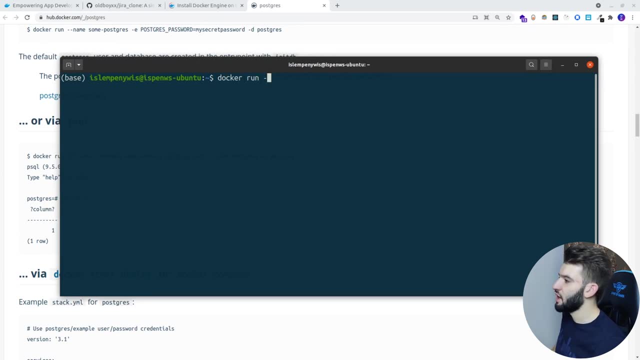 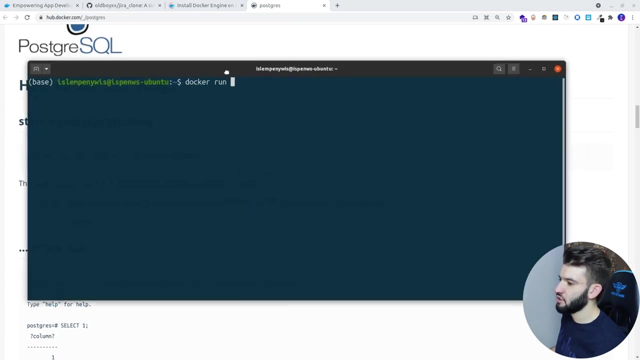 documentation real quick in here. I'm going to find, like this real simple command that tells us to tell on how to run docker more particularly. so this is going to do like docker run uh, for example, or uh, let's see. so yeah, there's this pretty much command, sorry, and we're going to run, so I'm going to. 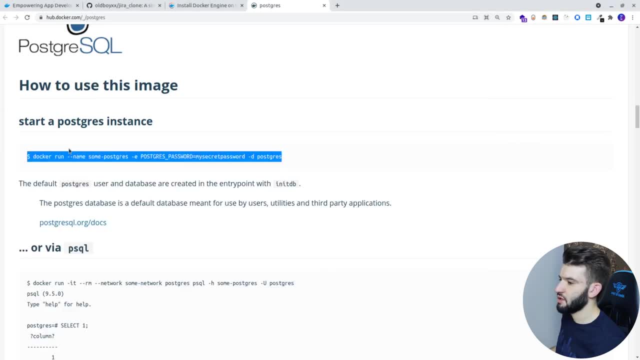 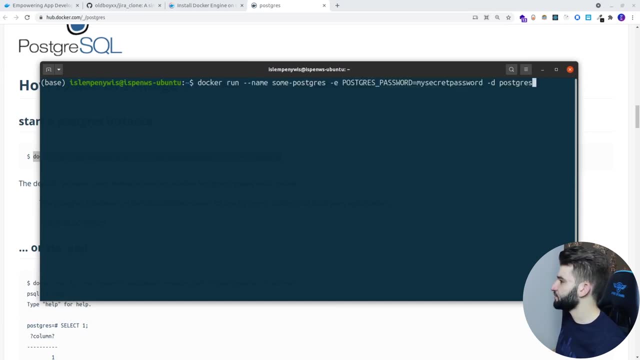 do? uh, let me just see, let me just go and copy the command. all right, I don't want to just like keep seeing the command and just like explaining, I want to copy it, explain it, and that will be all good. all right, so you do docker run and this is. 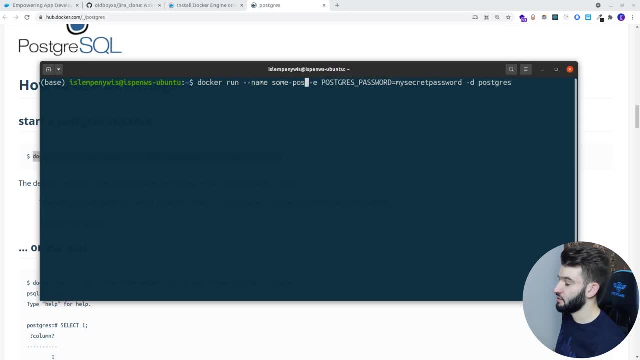 the name of the container I'm going to be like giving it, and the name of, like, the document container, the running document container. so, uh, let's say I'm just going to name this Postgres. okay, now for the postgres password. this is gonna be the, the root or the Postgres. 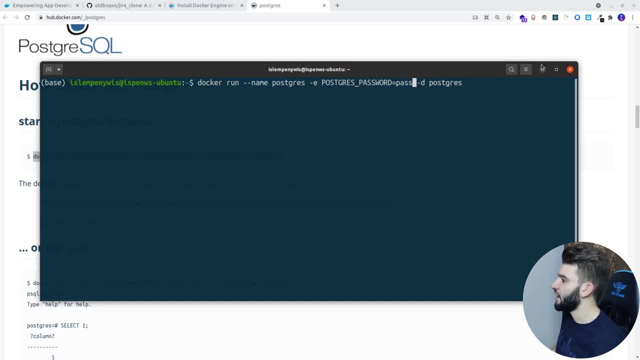 users password that's going to be used. for example, I'm going to use something like pass123. and if you're wondering what is this E flag, this one stands for environment, so E we're going to set this postgres password variable as an environment variable inside of, like the running container, which is going to be the 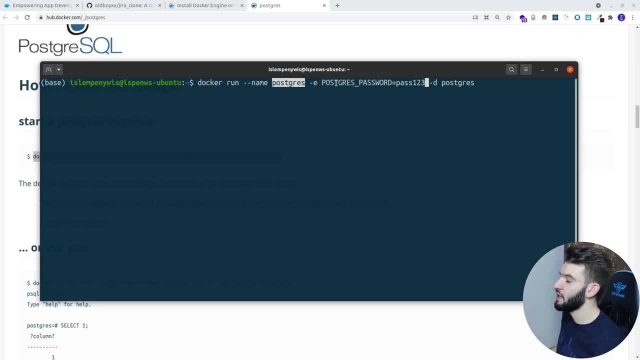 Postgres running container. so this one is going to be like simply an environment variable inside of that particular container and the d1 is going to be like as a daemon and, last but not least, we're going to provide what- the image name we're going to be using- you can use like version for. 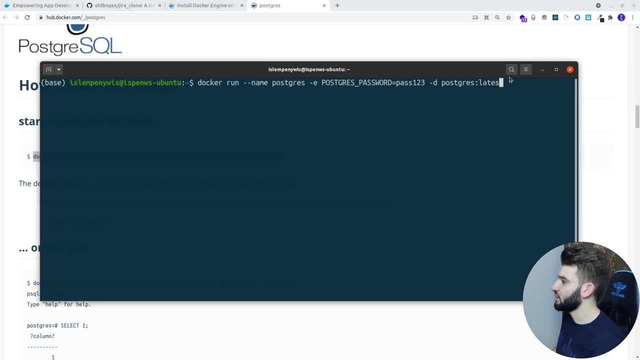 example, 11.5 in my case, or you can do like latest or something like this, and it's going to pull it out, so i'm going to use 11.5 of this particular version. click enter and this should run as: uh. postgres sql security returns this: uh, sh8 or this particular unique id about this container. 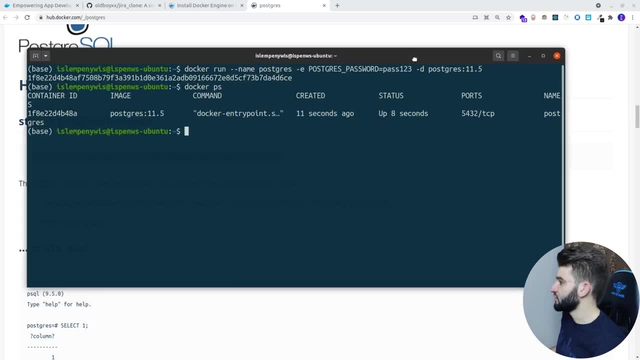 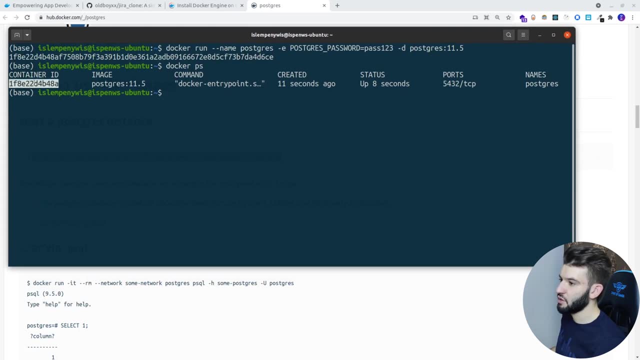 if you take a look on docker ps or uh process status in here you're going to find all the info part like postgres and and the currently running the docker container, so like unique id, which is just like a portion of this. um, the image, like i'm using, the version, everything, the command that is. 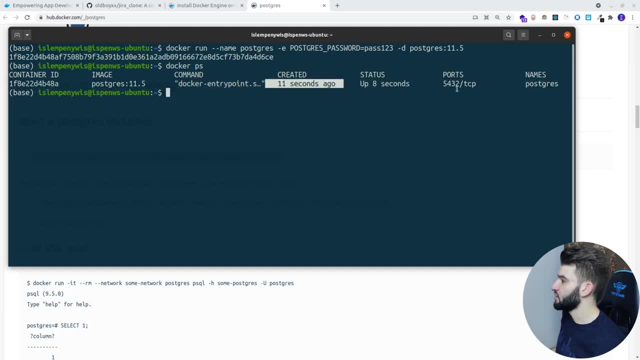 already run. uh, when it's creating the status you, there is actually a port which is 5, 4, 3, 2, and this is actually the exposed part, or the port that postgres is used to run on and, as clearly say this port currently only running inside of. 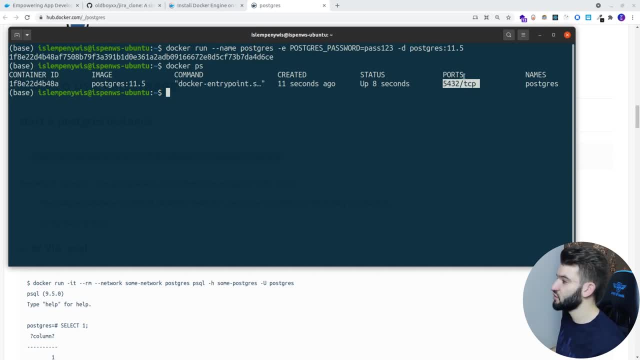 the container, it's not exposed to us on the host. so if we try to access this port uh from the host from our machine in here, we can't access it because it's not exposed to us, uh, to the host from docker. so to expose this, all we have to do is go ahead like tell it to expose that particular. 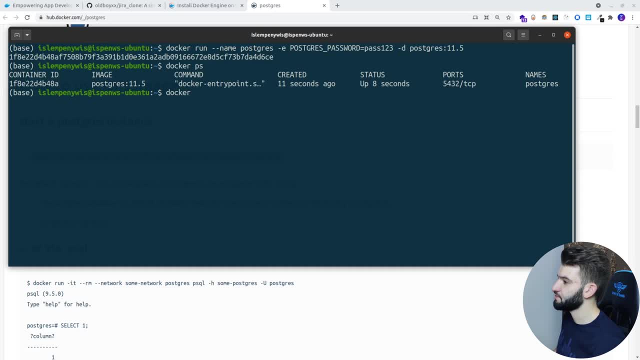 port. so let me just go ahead and like: stop this container. so i'm going to do stop and to stop a container. basically, this is another really really helpful command you're going to be using- is for like getting rinv or removing containers. you've got to first stop the container, then remove. 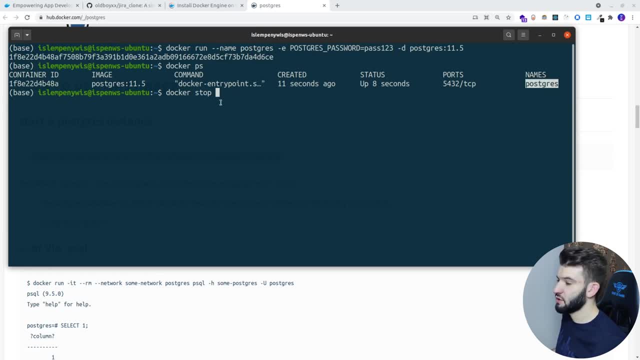 the container, so you can either provide the name in here for the particular container or the id. so yeah, whatever is going to do the job perfectly, just to stop it, just i would use the unique id. that would be safer and just docker, stop um error. there's no, uh, let me just see all right the same. 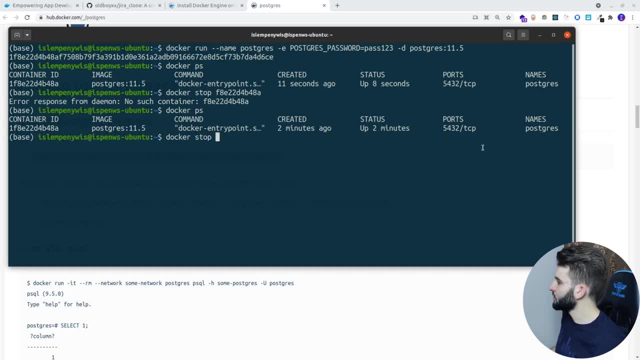 something odd. let's go ahead and try, uh, postgres, try to name and see what that does for us. there you go. it stops. uh, some reason. maybe you copy this wrong or something, or with the space. yeah, i think that's. uh, that's a wrong one. that's how it seems. i don't know why, though. 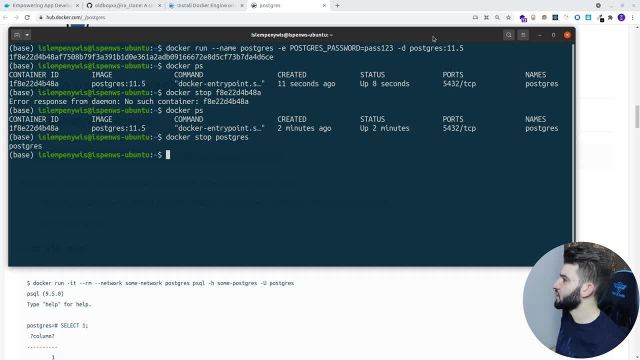 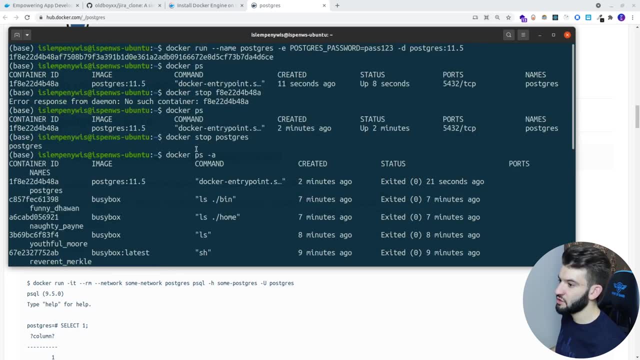 okay, um, so yeah, whatever. so we got this particular docker kind of like stopped and if you take a look again on the process status with the a now, as you see, the docker container still exists. it only stops it, but it didn't actually remove it and what we want is actually to completely remove. 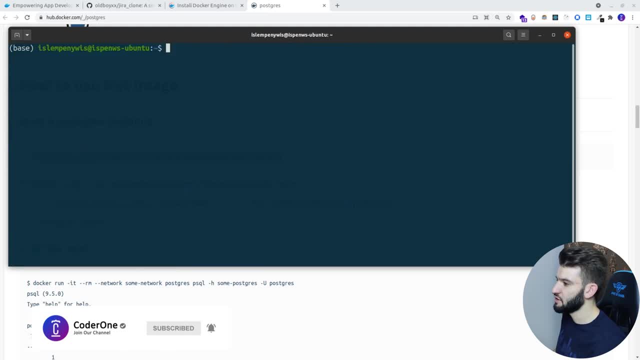 the container to start a particular new one container. so to stop or pretty much completely remove the container from, uh, the hibernated or from the stops containers list, you have to use the rm, which is, you know, pretty similar to the linux or unix kind of like command to remove. 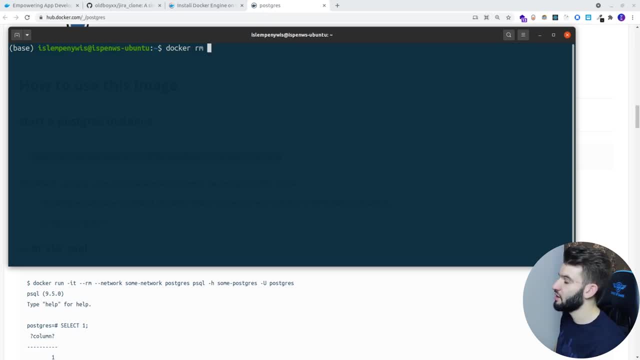 files and all sort of stuff or to move resources. so rm in here you give it like the id or the name, or what i would like to use a lot is actually to remove all the containers that are already listed and all the containers that already run before, because actually you can use the rm and there 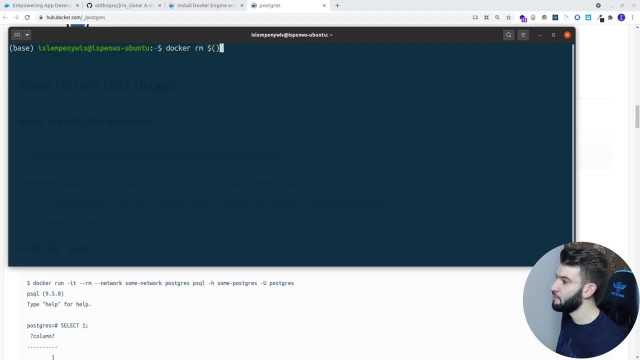 is this like really handy script which you can actually embed another shell script inside of it, which is you can do like another docker, ps, dash, a, dash q, and this one is going to bring you all the list. and this one is going to bring you all the list but it's going to just like do it into the. 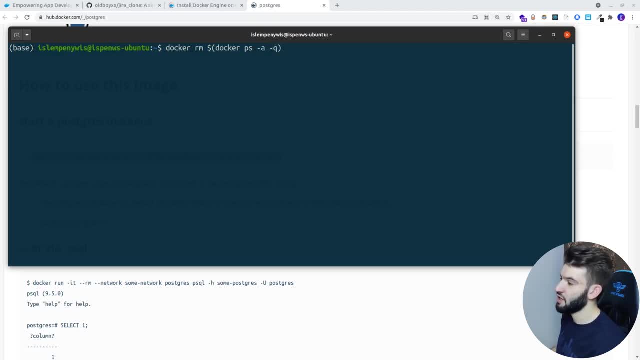 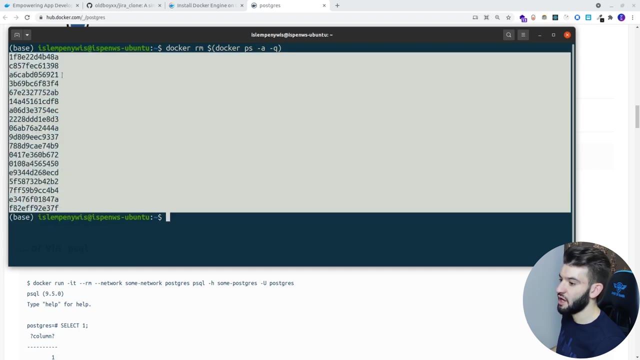 std in, not print it out, but into the std in. so the rm command in here can, can use those kind of like values, and what this one is going to do is pretty much going to remove all the hibernated, all the stops, can it containers for us. so we click enter, so you see, we get a bunch of ids, uh, printed. 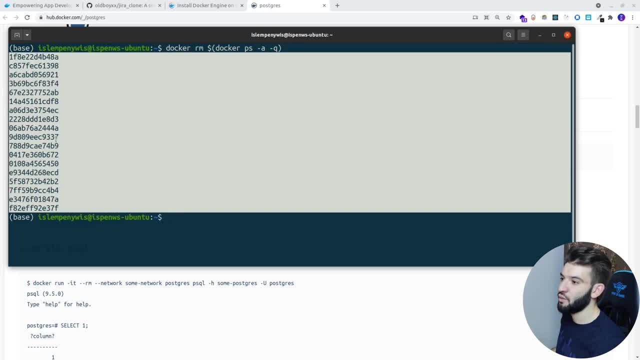 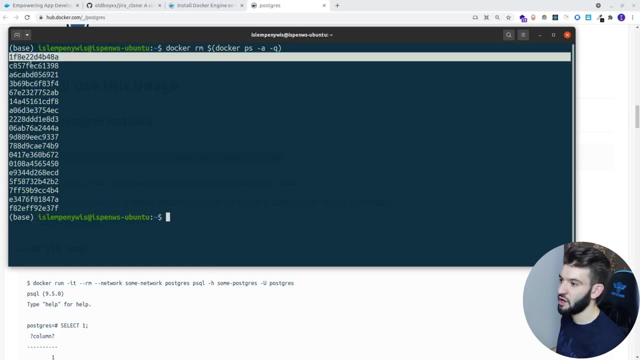 for us? and what does that mean? it just basically means that we got the commands particularly executed for all of these containers, which means, like, all of these container ids are deleted, so as soon as a container is deleted, just going to spit out and display the id of that particular. 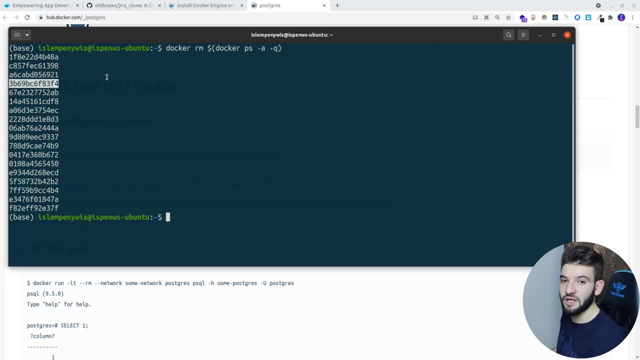 container that say: oh hi, this is the- uh, this is the deleted containers id, and, and that's it just like for your acknowledgements. all right, so yeah, pretty good, we got all of that we're doing again, so let's go ahead and docker. ps-a: no images, nada, even even the like stopped hibernating images. 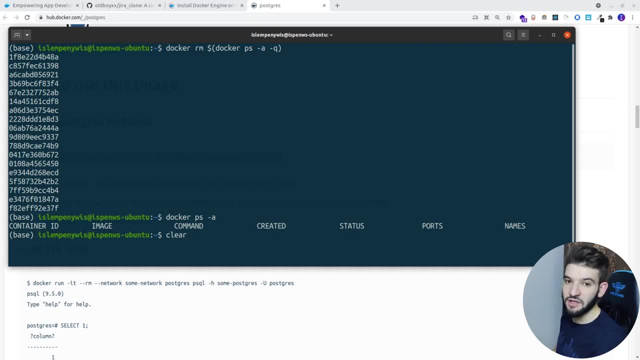 all of them are gone and from time to time, of course, as developers- me and you- uh, from time to time we have to clear this. you know, sticky cache, that is. that's pretty, pretty bad. it's gonna just like eat up memory and you don't even realize it, and it's gonna eat up a lot of memory, believe me. i. 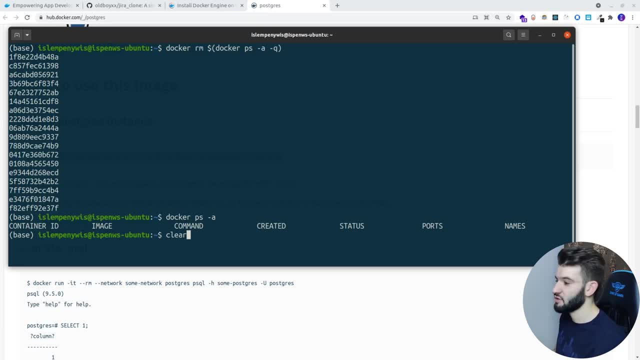 tried this a couple of times and even end up with like 200 gigs of docker's images and docker's cache and all that sort of stuff. so from time to time make sure you check out um the docker cache and make sure to clean that up before going to bed every night or something like this. all right, 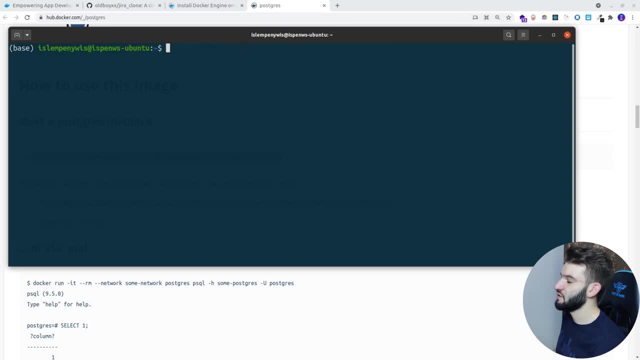 uh, pretty good. so, coming back into our main stuff in here is actually running the docker command, and let me just gonna just use this. okay, i want to get back into the postgres now. the postgres set before is going to run this, but what you want is actually to expose the ports, like postgres in. 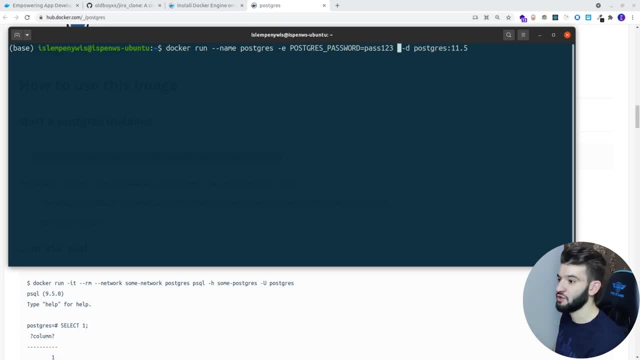 the docker container. so what we want to do is we want to expose this to the host, which is our current machine in here, from the docker's container, in order to be able to access and connect to the database. so to do so, we can use the p command, which is just like stanzain for ports. now to 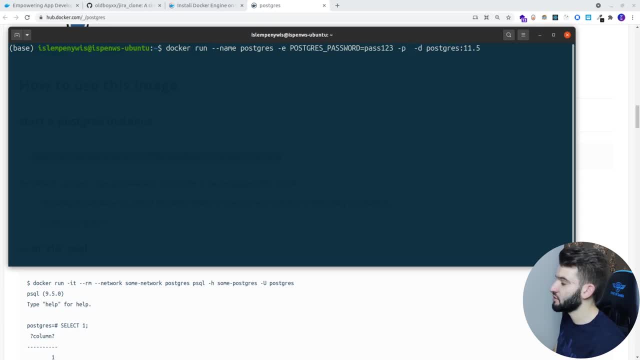 expose this first. we provided, like what is the host pros we want to bind this to. so i want to use the same port like 542 and we're going to use the same port like 542 and we're going to what is the containers port we want to bind to? so the container support, of course, like what port is? 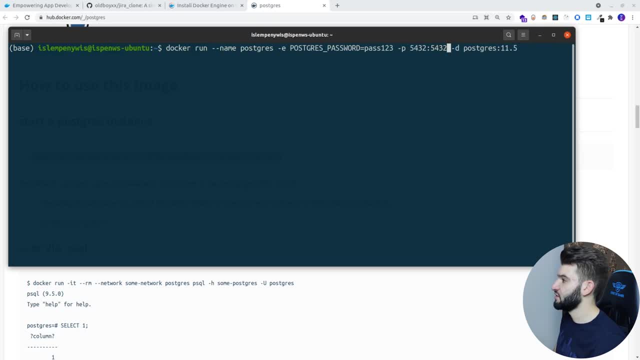 being opened inside of the container by postgres and obviously this is actually fire, five, four, three, two. but for the first part in here, like what you want to bind to, you can choose whatever. you can choose- 8 000 or something, and this is going to bind 5, 4, 3, 2 to 8 000 ports on your own. 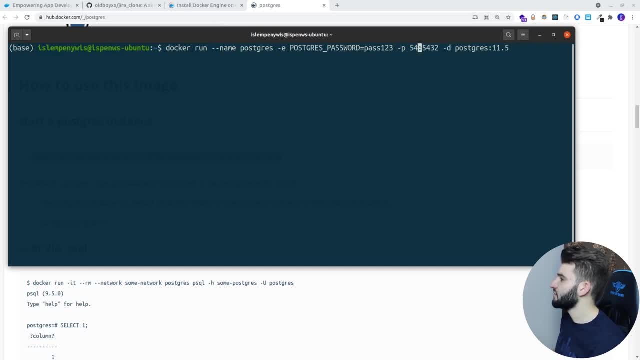 host machine. all right, uh, i'm gonna just like make this a little bit more um more accurate for you. so we're gonna make this like 8 000, all right, just to make it a little bit more simpler, and go ahead and run this. so this should run the docker container for us. we do docker ps. 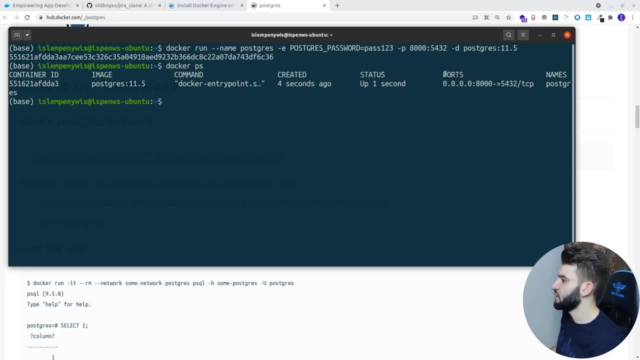 now we're gonna see another piece of information which is pretty important. i'm going to see the porus and the porus right now, excuse me, this 8 000 which is on zero, zero, zero, zero would just basically represent our local host with an 8 000 port is bound inside of the tcp. container, or on your sound of the docker's container, to fire our mix and download it. all right, so let's do that. so let's use the docker great, and let's see, now let's open up another. we can see this. so docker container. so we're going to see another piece of information. 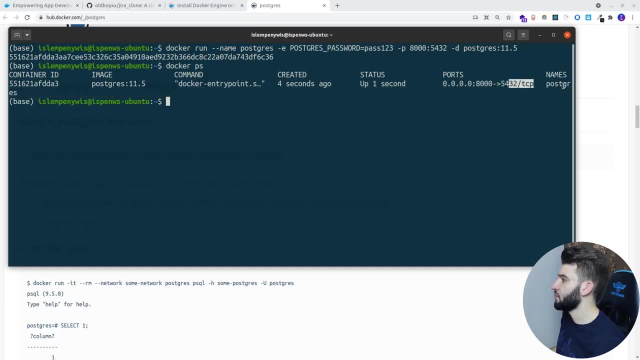 which is pretty important. i'm gonna see the pores and the pores right restvideo. see this 8 000 which is on zero, zero, zero, zero. we're four, three, two TCP ports on the Postgres container. Now we can use this port to connect. 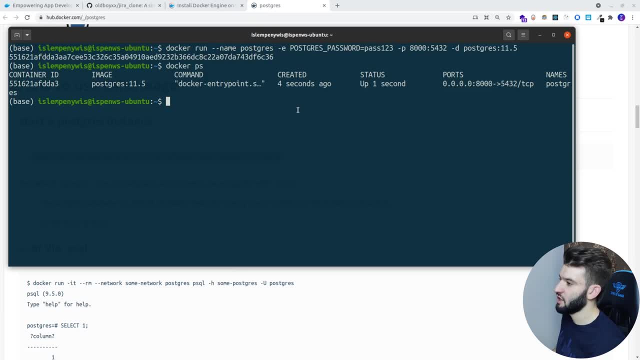 to the actual Postgres container, And that should be all good. Now we can go ahead and use like the P SQL pretty much command line, which is like a client that allows us to connect to Postgres kind of like databases, And we can, for example, say, oh, we want to have this house on the local. 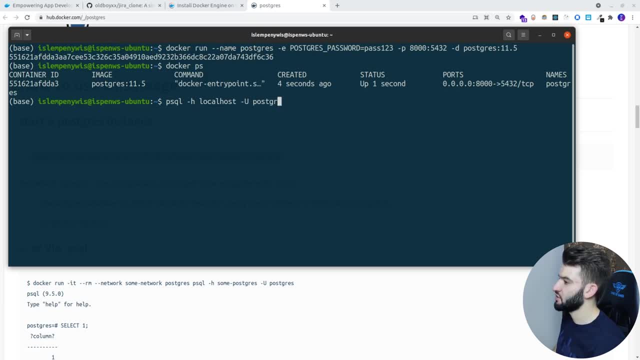 host And we can say, like the user is Postgres, which is by default created by the Docker container in here for the Docker or by the Postgres image, And you click enter, like it doesn't know the port. of course, by default it tries to connect to this port, but we change the port, So we're 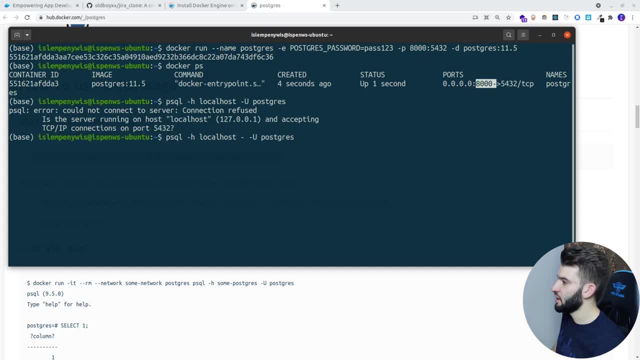 using a different port. So make sure to provide the port here, Like, for example, say, P 8000, and then get asked for the password. we already provided password like as pass 123. So we're going to do that, And then we're going to do that, And then we're going to do that. 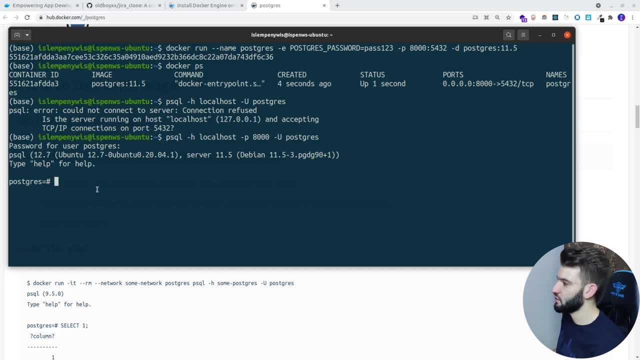 So pass 123. And hallelujah, we got access to our server that is running inside of Docker. So, even though you're not going to be using Docker for development or something, you can even have images and Docker containers running your own kind of like databases servers and like MySQL. 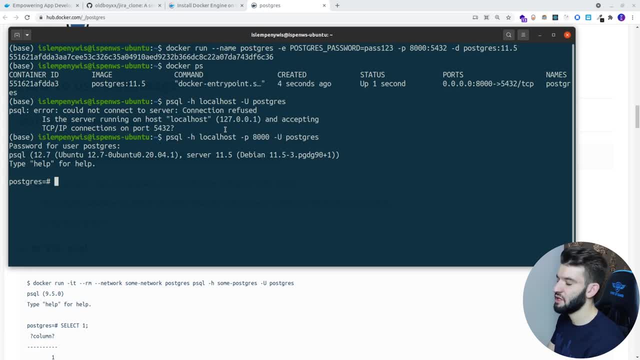 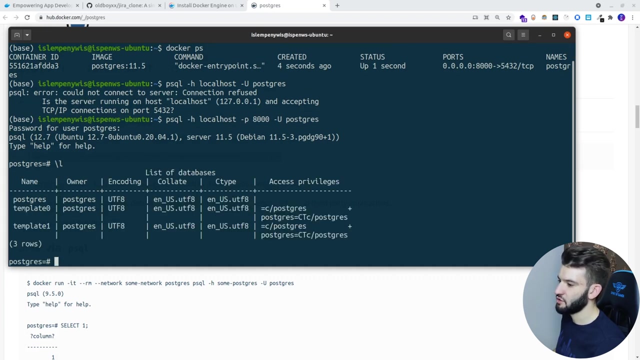 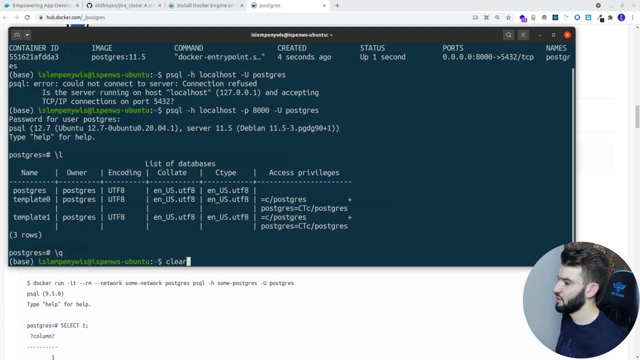 Postgres from time to time, And this should be pretty, pretty simple. It should be like really easy to set up, really easy to destroy and really easy to download without just having going through the mess of installing inside of Ubuntu. copy gearing is going to the config file and you know version mismatch and all sort of awful. somebody hates about this, But Docker makes it super sweet to handle and super easy to work with. Sweet Now, yeah, you can. you can do whatever throughout the CLI, like list, whatever kind of database or variable there, whatever you can do with Postgres, of course. So I want to quit and I want to go into something completely different Now the Docker. 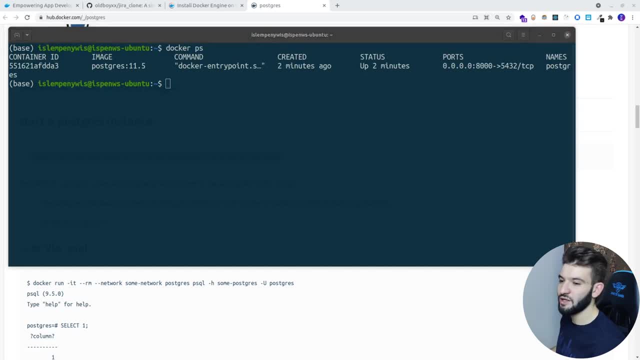 container is already running, which I don't need any more, because what I need now is pretty much to go ahead into the Docker file. So, Docker, stop. And you can, of course, use the same command that I used before to stop it all, But I'm just going to use it: postgres. we're going to use its name to stop it and make sure to remove it as well. I don't want to use any like jargon or something, And that is removed as well. Pretty sweet. We got darker, everything made up in a really simple way. So that is pretty sweet. Now it's like a docker, docker, docker, docker container. And then what I'm going to do is I'm going to say container and I'm going to go into my Docker And you can see, i'm going to define my Docker, docker container. So I'm going to go into the container and I'm going to define my Docker container as well, And i'm going to say container and i'm going to go into my Docker container. And when, 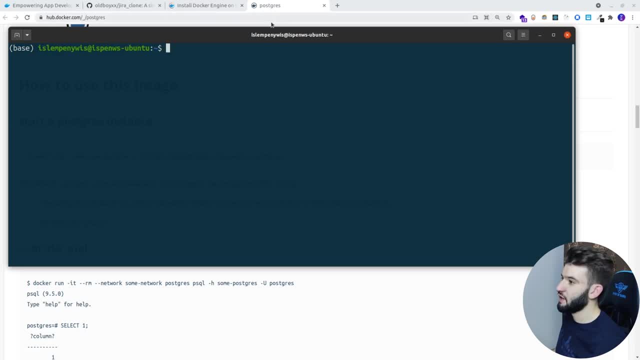 really awesome way. Now, enough Docker basic stuff. Now let's go and jump into creating the most important one, which is the Docker file and Dockerizing a real world application. So the real world application here we're going to be using is actually called the Jira clone. So the Jira clone. 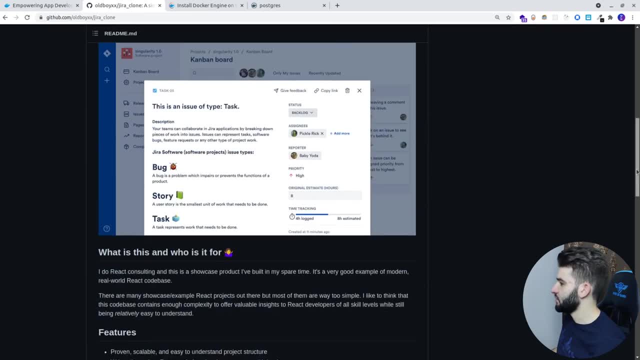 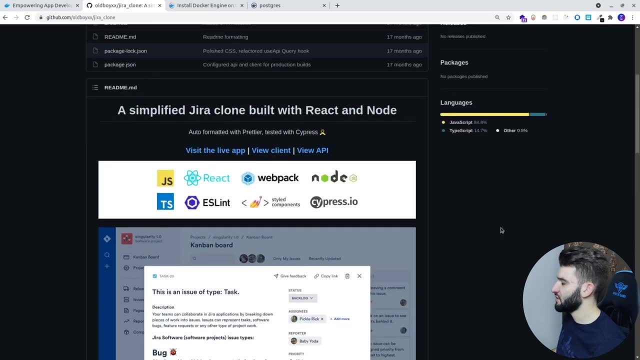 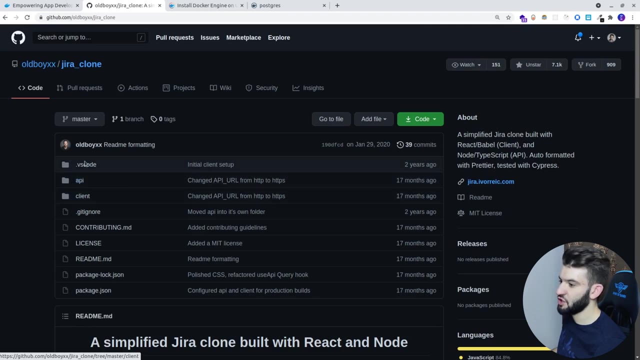 familiar with Jira. it's like you know the task management here, this, you know Scrum and different techniques which are used by developers and teams, And so, yeah, this is actually a really well made up clone that is made up between two parts: the API, which is created throughout Nodejs. 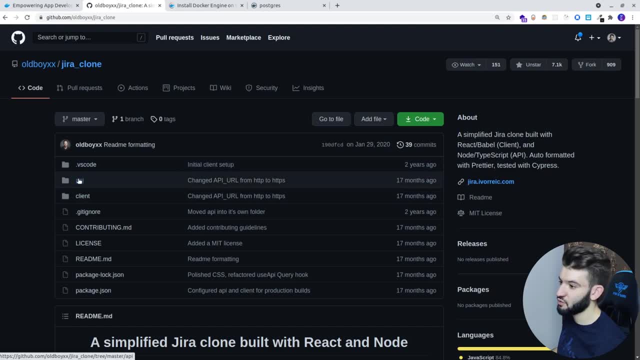 with Typeform and Postgres database running And the client is actually using like React and everything to run that. of course, some Nodejs to run this, So it's basically a full Nodejs, kind of like full stack Nodejs application with React running, Postgres and many stuff like Express for 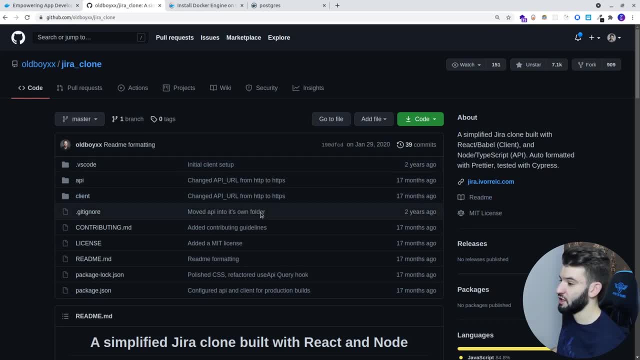 Exposed API and everything. So what we're going to be doing with this application more particularly, I'm going to clone it, I'm going to take this application for granted And I'm going to just like Dockerize this application from start to finish. And, last but not least, we're going to also add Docker compose to create this kind of 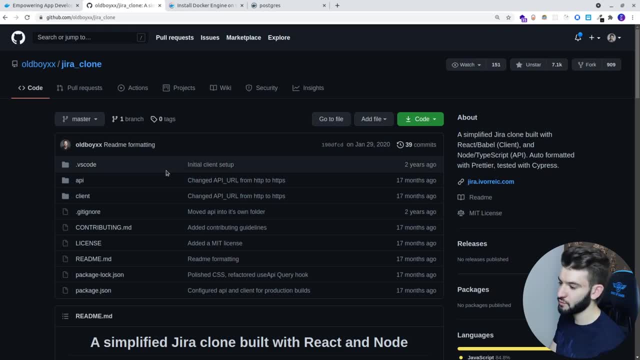 like services, kind of like architecture of how you can pretty much integrate everything is in this into a single Docker file And with a single command we can have all our servers will all stack running, up and running without any issues. So, for example, we can have Postgres server running. 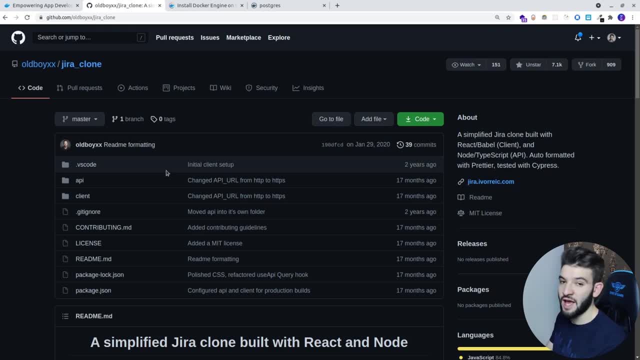 up alongside the API server, alongside the actual react client server, running all with a single command, with all configuration and everything throughout Docker. So we're going to be using this if you want to use this kind of like demo or when you're going to use this kind of projects for. 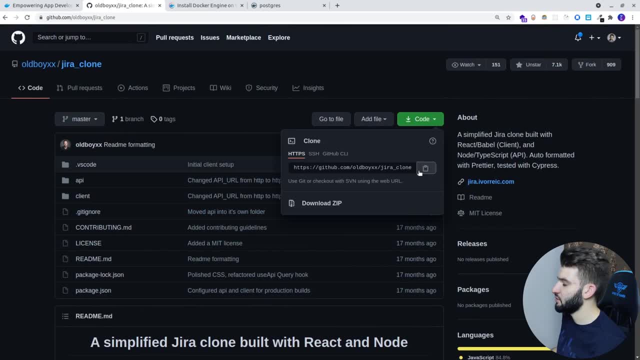 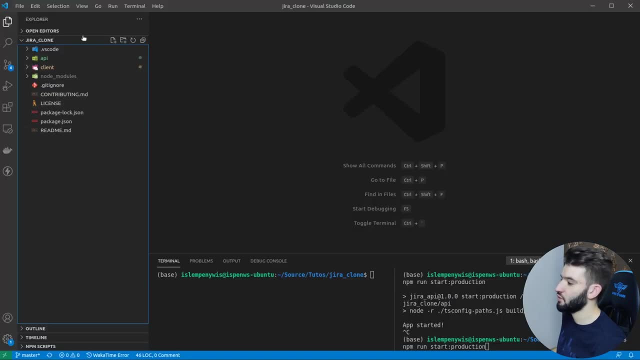 demoing and make sure it works perfectly. You can go into like cloning up using this link and just click it, cloning up whatever you want and you can have it. so I already got that, already open this throughout my VS code in here, And I got some jargon in here, I don't know why. So I'm going to completely get rid of this. 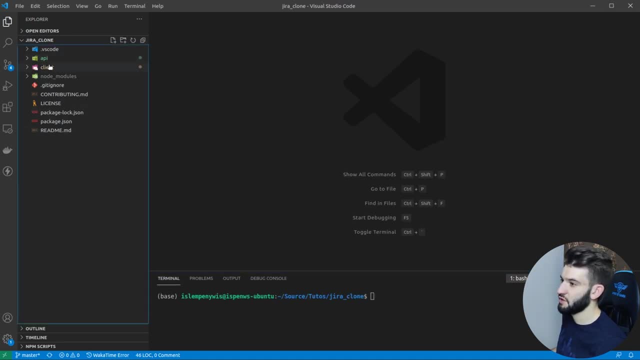 as soon as, like I need it. So there's actually a bunch of stuff in it. So, for example, the client, which is its own kind of application, and there's the API, which is its own application as well, And there's this kind of like node modules is shared between both. 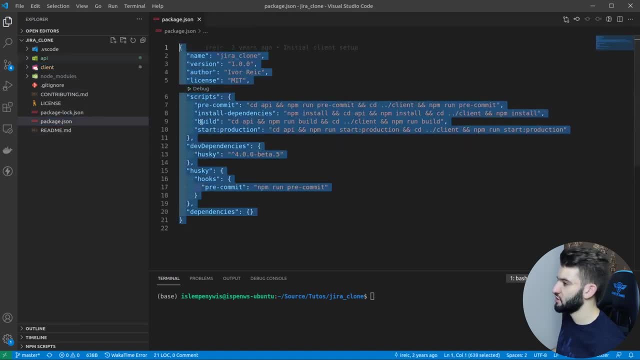 which doesn't really make make a lot of sense. But there's this package or JSON that allows you to, for example, start production for both clients and API, or a stall dependent on the API. So that's kind of what we're going to do here, And then we're going to 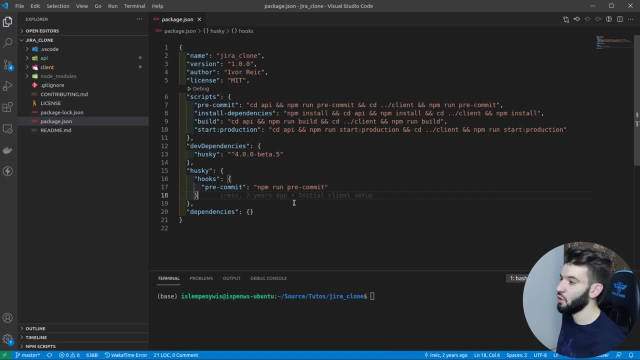 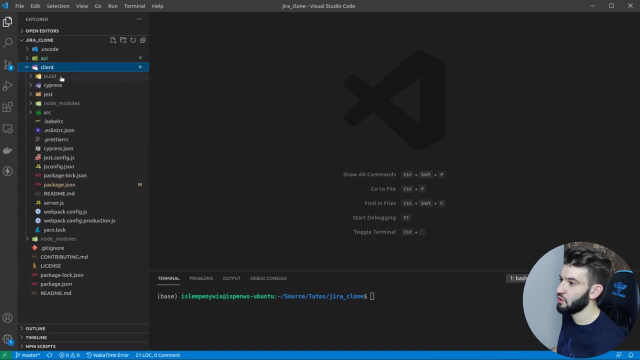 do some dependencies of all sorts of stuff. But since we are going to be dockerizing the whole stock in here, we're not going to be needing that much of this package or JSON. anyway, we're going to be needing, or using the inside, the internal package or JSON for both of these, the client and 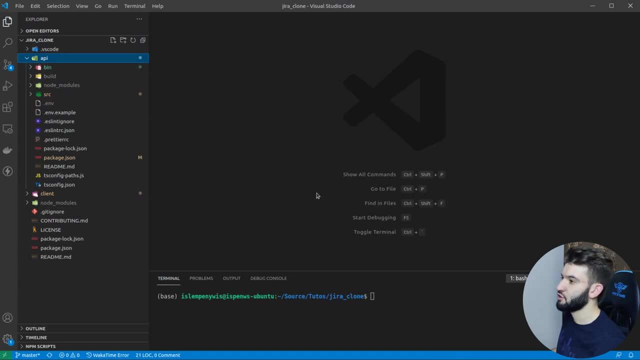 the API to make sure it works perfectly. All right, pretty sweet. Now, first things first. what we're going to be doing is actually dockerizing each part alone. So this one is going to be its own server, the client is going to be its own server and I'm going to be dockerizing. 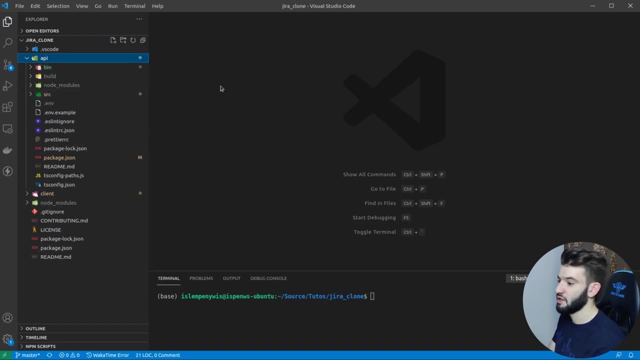 each one in here and actually connect them throughout rest of the API's, since they are already like connecting and talking to our rest of the API's. So we're going to make sure to run them on separate ports and just like define: oh, this is the port, this is one running. 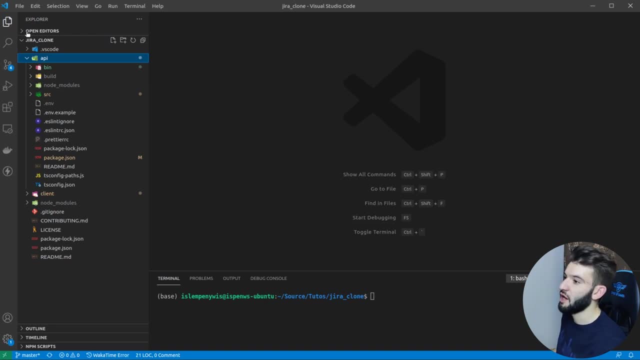 and vice versa. That's basically what we're going to be doing throughout this. So to start, actually for Docker to pretty much work and be able to take kind of like the projects and make it a Docker compatible or create an image from projects, basically it has to have a Docker file, So you're going to have go ahead and do like a. 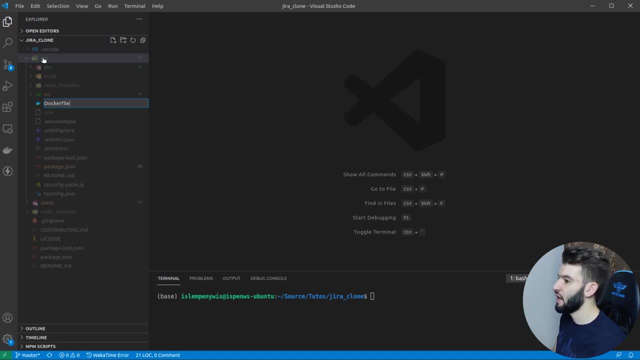 Docker file And basically for international and many, many people uses naming convention is actually to start with a D as a capital and, just like you know, name it this way, with no extensions. nada, just like put it this way and it's, and it's available enough, And actually I'm using 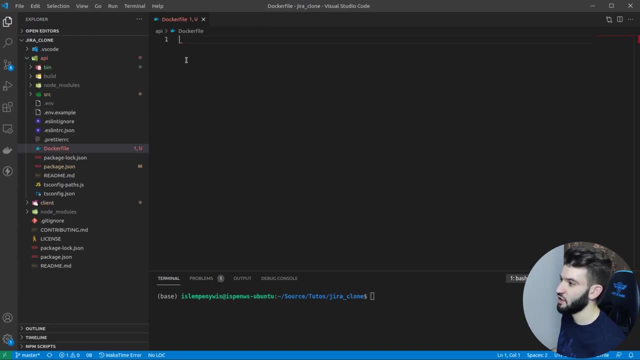 some extensions from VS code to have this Docker recognized and everything to have the syntax really made up with some into license So you can go in and grab this from VS code extension store or marketplace. I'm spelling that right, Okay, so this is the Docker file I'm going to be using And basically, 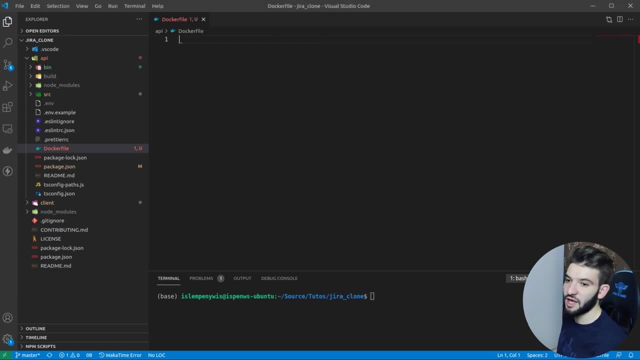 for the Docker file I'm going to be using is pretty much like what's gonna. what's going to happen is pretty much going to take this Docker file or this projects in here and tell Docker how we're going to use this or how the build process is going to be going throughout this to. 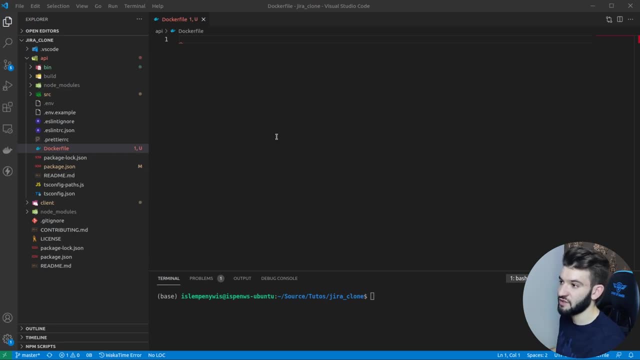 really organize and to integrate natural projects into an image. And what I mean by this it's actually this, this final project, the whole files in here for whole configuration, the whole node modules, scripts and everything There's going to be taken out. it's going to be putting. 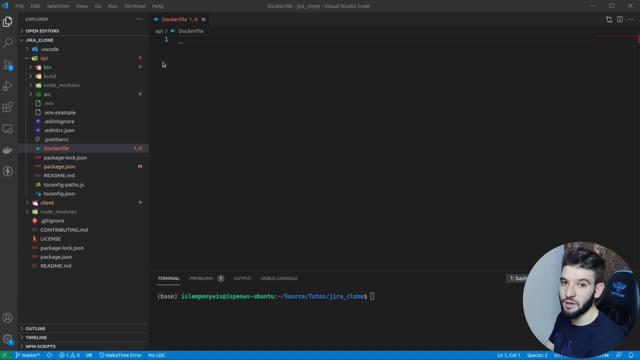 inside of an image it's going to be bundled inside of, like this really compressed and bundled kind of like Docker image. Now, whenever we need this image, wherever we need to run the application, all we need is basically just like this static image, like you. 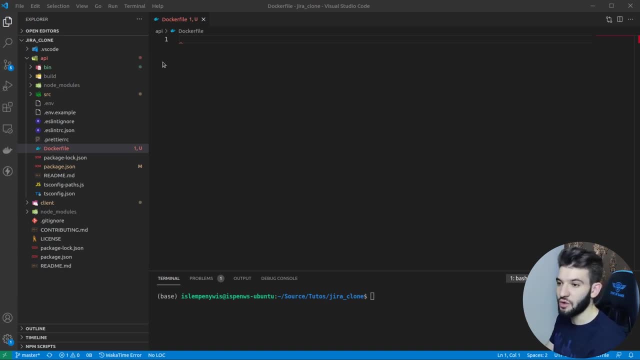 file piece image and we grab this image, we use a docker command run and we run the image and the image runs as expected to be every single time, with no unexpected changes or any kind of like odd behaviors that we didn't include. so that should be just that straightforward about creating. 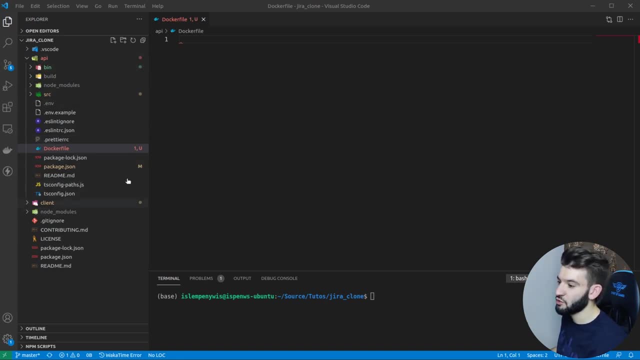 images and we have to use actually this docker file to tell it how to dockerize or how to build the image for this particular project. all right, pretty sweet. now, for every single docker file, what you need to start with is actually the from now. the from in here tells it like what: 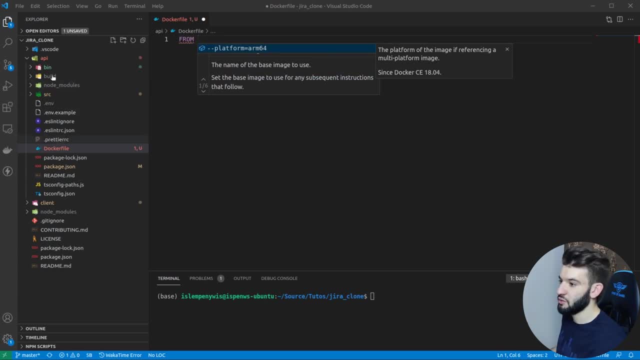 base image. we're going to extend to be able to build this image, because obviously you're going to be needing some base image to run this. so, for example, if you've got like a php- uh kind of projects which presents or runs on top of php or, for example, on top of layerable, so you're going. 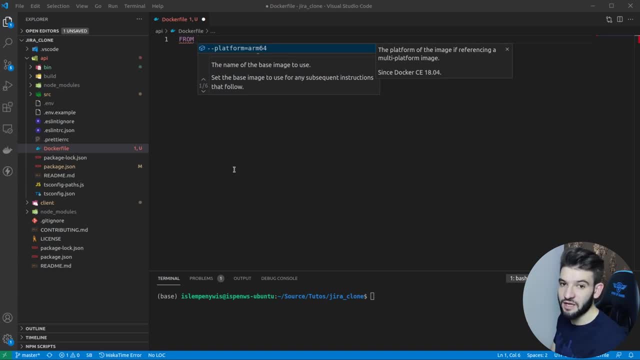 to need some. you're going to need some. you're going to need some: the basic or the PHP kind of image, the Docker image. of course, you're gonna extend this to be able to provide the core, provide the actual PHP kind of binaries and interpreter. 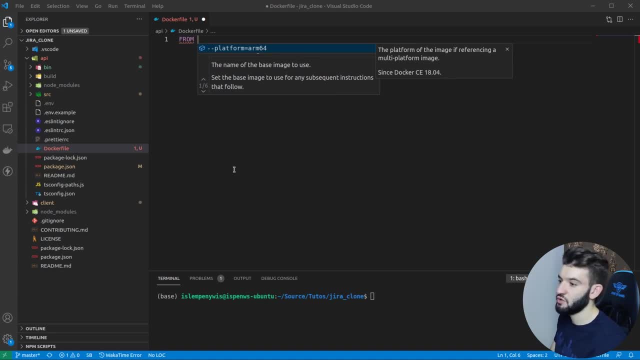 and the whole language kind of tool set to be able to be used to bundle that into the image and be used actually internally instead of the image or the container. So this is what's gonna happen as well for us, So we're gonna extend the Nodejs. 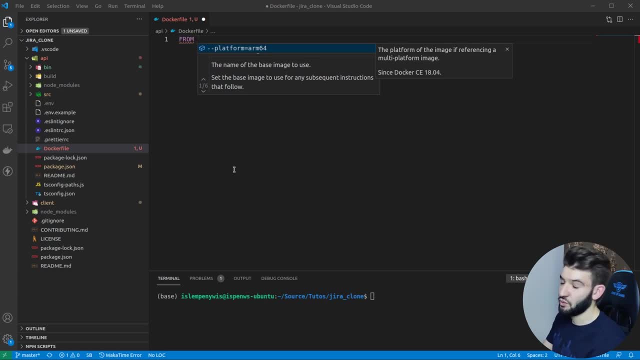 kind of like pretty much image which we already got from Docker, or was gonna already be, like pulled out automatically. if you don't have it locally pulled out on your containers or on your machine, Docker is gonna do the job for this, so you don't have to worry about this. 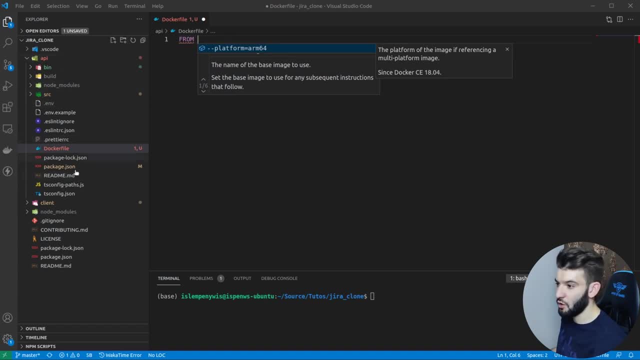 But all you have to worry about is actually you're gonna use a node, because the whole project in here is actually based on Node. The whole project is gonna run on Node, the whole scripts and everything. So, since all of this is actually JavaScript, 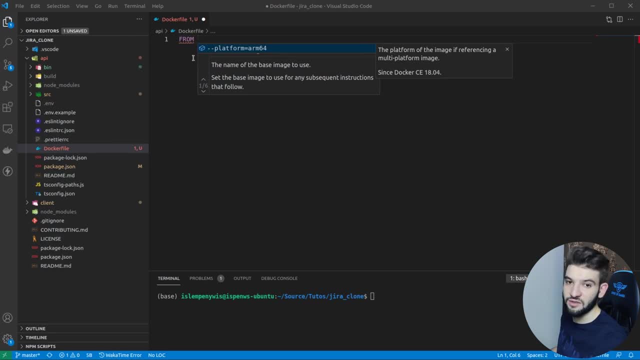 so we're gonna extend it and then Node, I'm gonna add, like our kind of dependencies and how to install dependencies and everything, And I'm gonna start off the projects as we expected. All right, so I'm gonna do from and you give it like the image name. 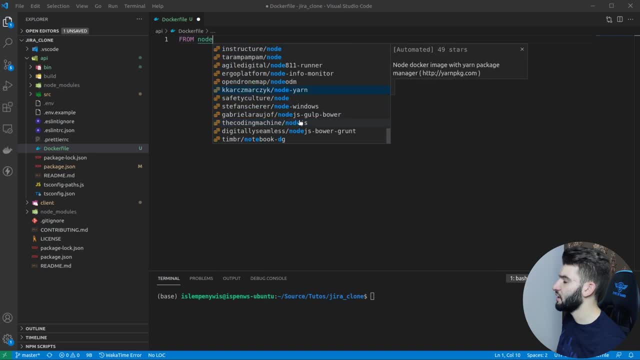 So there's actually. it's gonna give me a list of images that are already available on the hub there, or the registry. I'm gonna use Node version 14 and I'm gonna do the as as this one or this as keyword, what it does, just like you give it like a nickname. 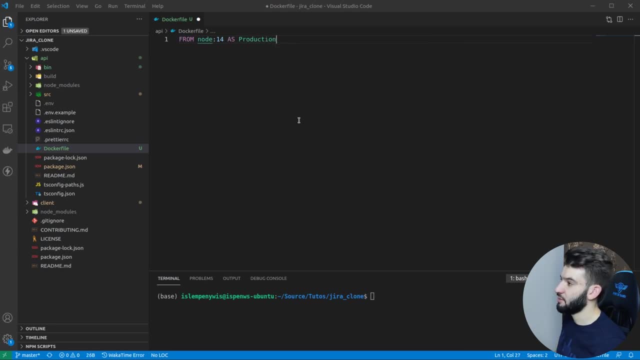 what this image is gonna be doing. For example, I'm gonna give it like this as a production, So I'm gonna use this Node for seen as a production for this particular Docker file. Pretty sweet. Now the second thing in here. 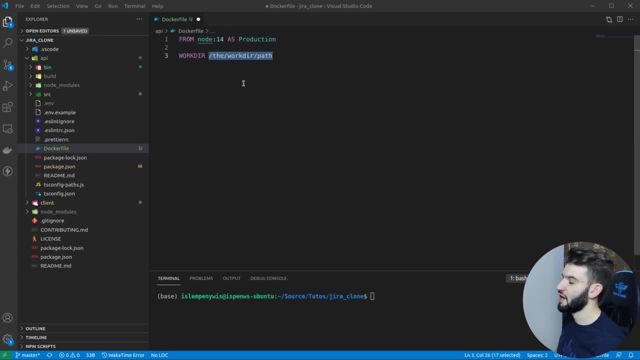 I'm gonna use another command which is called the workdir command, And the workdir command in here it's pretty much tells it like to change the currently working directory to another directory And remember always, always a Docker container or a Docker image. 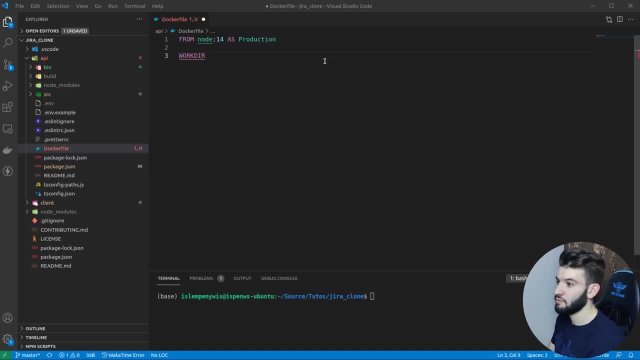 it's just basically a Linux Unix kind of like operating system, small operating system running on behalf of our operating system. So that's it. So any kind of like Linux command, of course Linux basic or Unix kind of compatible command can run in this particular sense. 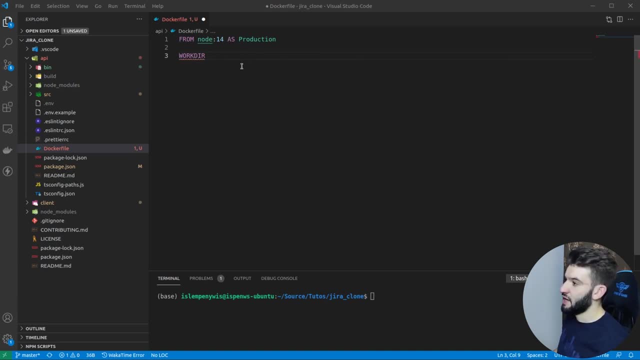 So basically you can imagine this as a CD Unix command, just like to change the directory. So what I want is actually to go inside like, for example, let's say, I'm gonna use inside of like a user SRC, I'm gonna go inside of like API. 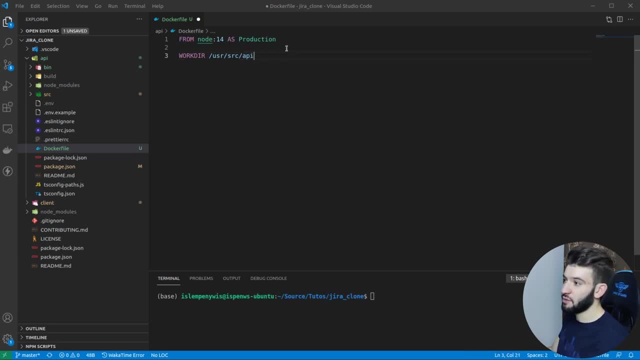 So the whole code or the whole kind of like a application core is gonna be residing inside of this, like this folder, And if it doesn't exist, it's gonna create it for us and everything. So it's gonna handle everything behind the scenes. 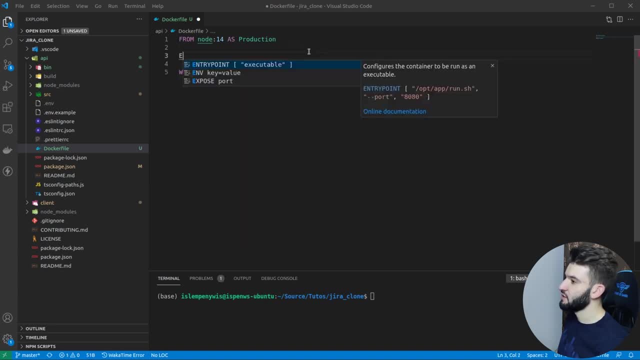 So I wanna have something else which is an environment variable. So I'm gonna put this ENV in here which is gonna set an environment variable inside of our container with a specific value that's gonna be used. It can be used by anything, pretty much. 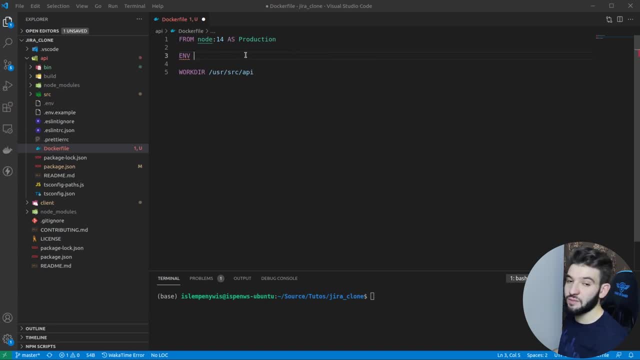 for example, it's gonna be used by our application or something that's gonna be running alongside our application. So, just like an ENV variable is gonna be applied throughout the whole Docker container in that particular sense. So, for example, I'm gonna put in node ENV. 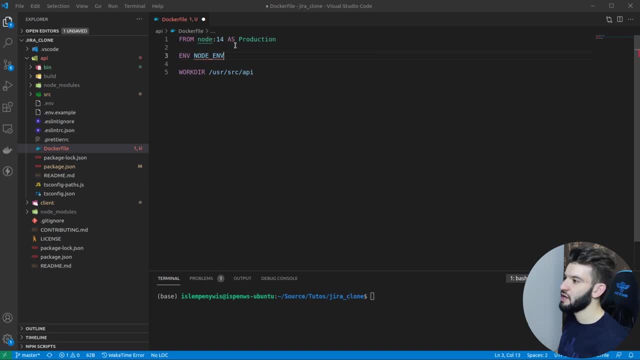 which is gonna tell our application that, oh, we're gonna run this application on a particular or on a production base with throughout the node ENV environment variable. So I'm gonna put like production and this is gonna send it throughout the whole container. 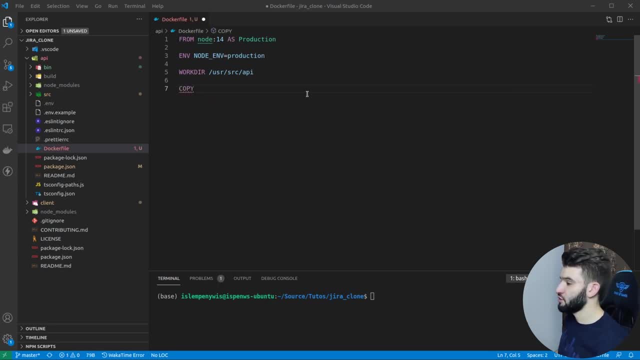 All right, pretty sweet. Now the second one, most basic one, gonna be copying the packagejson. So I'm gonna copy back packagejsondot to dot, or basically. so the packagejson is gonna be copied from this local directory which is right over here. 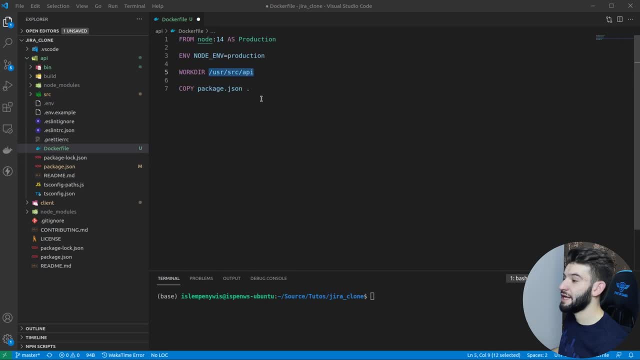 It's gonna be copied to the targets, which is right over here inside of the container. So this is what the copy command does, And I'm gonna also copy the package- sorry, so package blockjson- inside of the container as well. So just like to be able to do that. 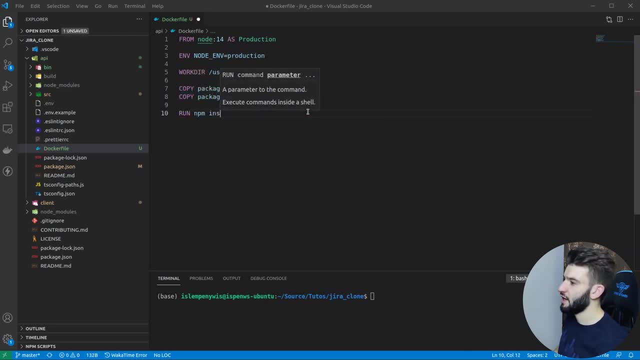 So after copying all these, let's go ahead and do npm, run and install And just like to install the dependencies in a production based environments with that. So it's gonna install all the dependencies on the packagejson. So after make sure the dependencies 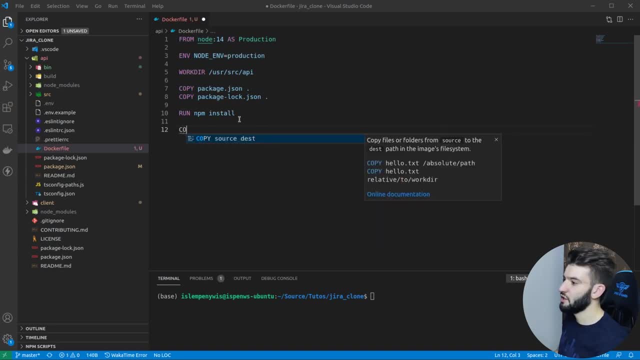 are installed and everything, and what we're gonna be doing is actually do another copy which copies everything from this, like everything from this local directory which is inside of the API, like where the Docker file resides. So everything is going to be copied inside of the Docker container. 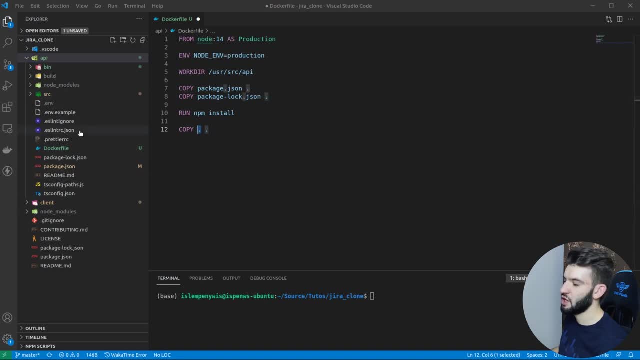 So this is, this is what this means, like dots means the local directory and the other dots means the local directory in relative to the Docker container running. So that's, that's basically what it is, And the other thing that you're going to use actually another run, APM install or pretty. 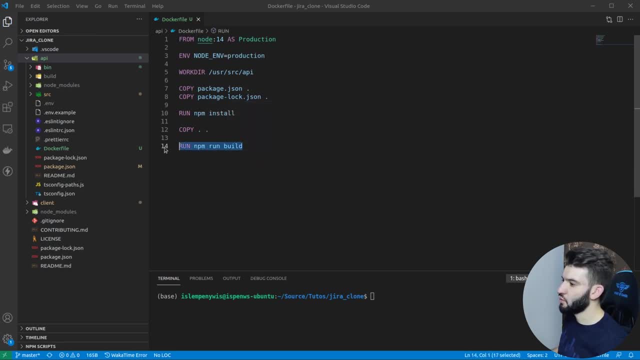 much NPM run build sorry, and this is of course, going to run the build. after some dependencies, after having the whole source code putting their the whole projects in here, I'm going to run the build command which is going to build for us, or just like a: create this build. 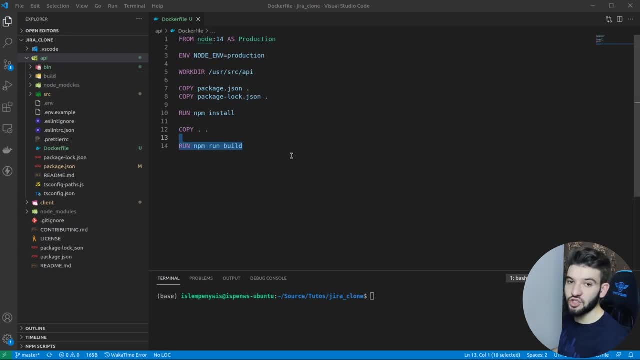 folder is going to create a fully sophisticated production, ready, built, for us to be able to use this. So yeah, hope you're all guys familiar with all of that, With no GS and everything, because you know this might seem a little bit kind of weird. 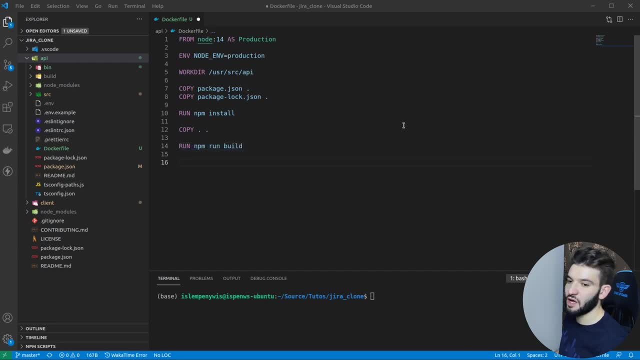 if you hear it for the first time. So make sure to get some knowledge, or grasp some knowledge before jumping into the video. So yeah, so this is going to run the build command. Now, the last thing on this, like on last thing on a Docker file you have to provide, like 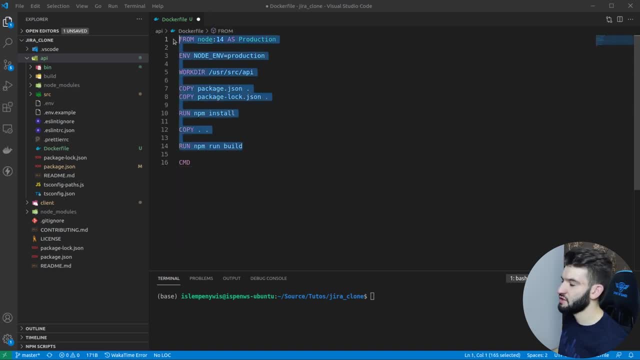 an entry command that, after running all of this, this is a pretty much just like a preparation is going to be done behind the scenes just to prepare for the startup of the actual container. Okay, This is going to be run by this or this, this image in here. 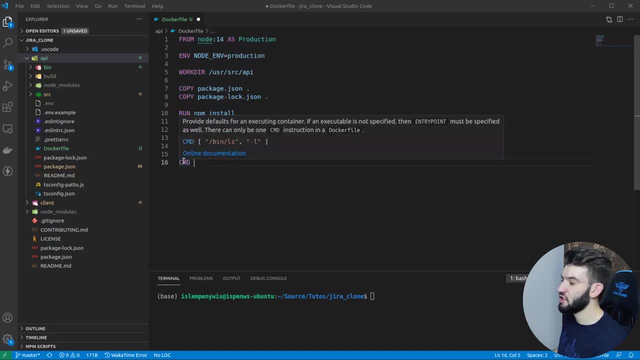 So the CMD in here is going to be like the main command executed by default by the entry or buying, like when starting the container. So this is like going to be the running command, That is, the main running command on the actual container. So you can imagine this like running or starting up your server or something like this. 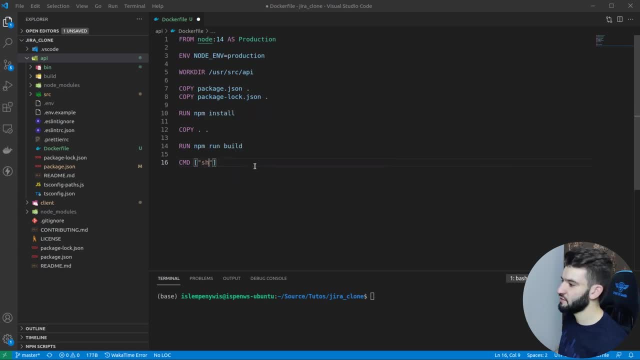 So this is basically what we're going to be doing in here. So the command takes first like a couple of arguments. We're going to use the CH or the the shell kind of like command to run this. So make sure to use this, because this is actually a really safe way to do it. 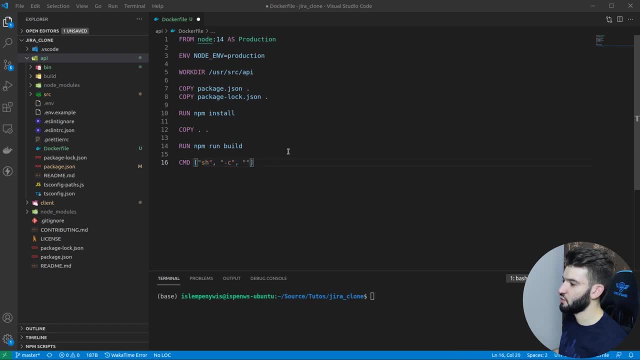 It really perfect to do is and run it on a shell environment just to make sure that is running perfectly as you want it to be. So that's why I'm putting shell and providing, you see, just to run an embedded custom command. And here what I want to run is actually run stars production. 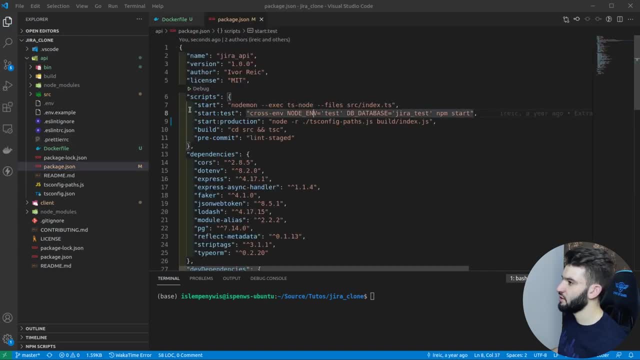 And this one is going to run us the production script, So take a look on the screen. Okay, So we have a package of Json. exclusive is a star production and it's going to run node GS with a built from the build folder in here and everything's going to be running as expected. 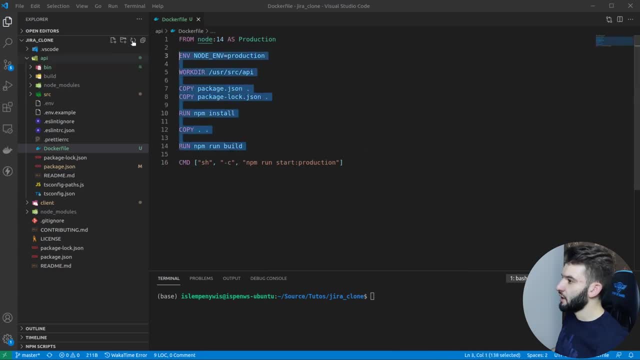 to be All right. So that should be it for this Docker file. And yeah, so the Docker file now should be ready. Just like that Simple. We we just some in V, five variables. We change the work directory copy, the the new files for installing and installing dependencies. 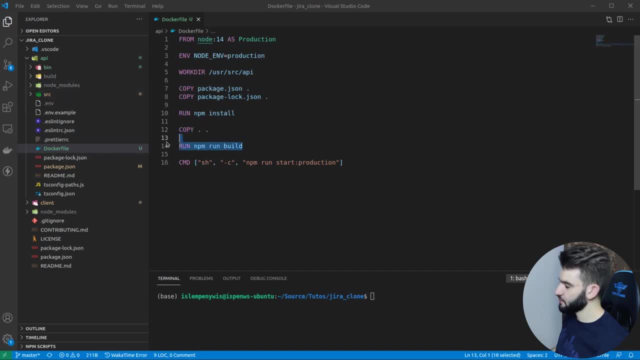 and basically just copying the rest of the source code. Last one is just like build everything from the source code and dependencies and the installed modules and everything, Just like combine them all together. And, last but not least, we run or start up our server and that's basically where it is. 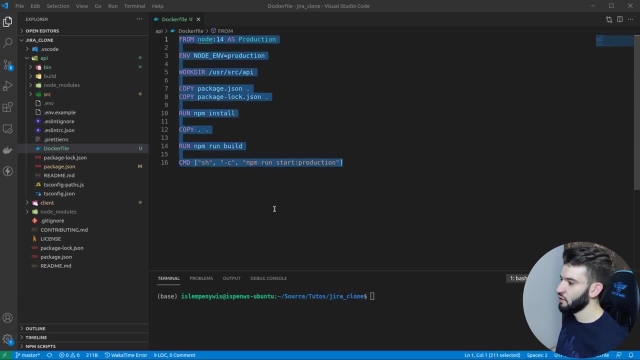 So pretty simple, right? So this is the image. Once it's built, you're going to have all of these instructions. uh, like you know, harboring they're going to be like just like crave there, And whenever we start the container, this instruction is going to be starting a one. 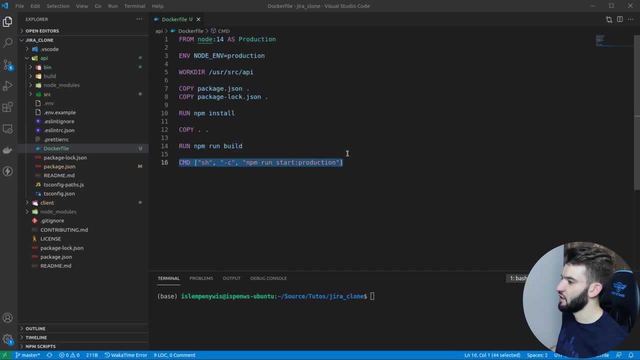 by one, just like doing all of the sort of stuff, and this command is going to be started once we start our, or our container, uh, in production. All right, Pretty sweet. Now that's what we should do as well for the second one, which is the client. 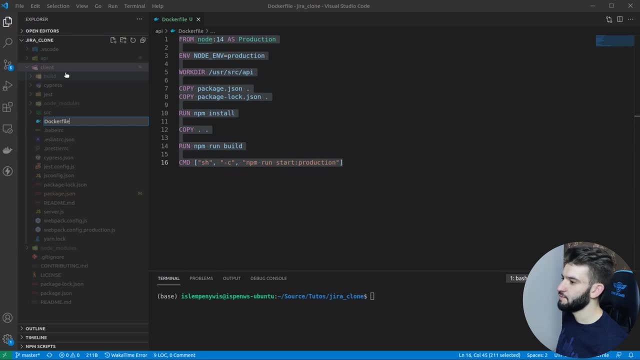 So that's why I'm copy pasting in here. I'm going to have another Docker file and this one gets like copy pasting. just change a couple of stuff Now. instead of like, for example, instead of like API, I want to go um, for example: 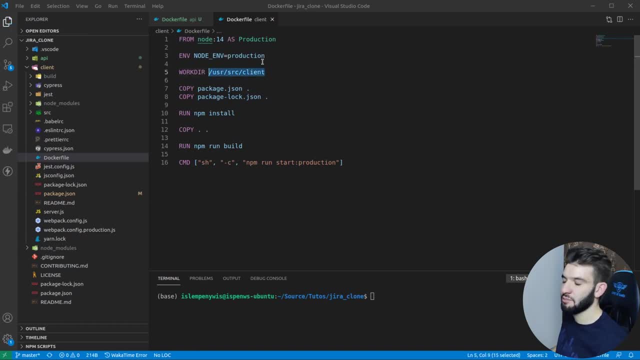 let's say, clients. of course, this is. this is not mandatory, You can completely ignore this, but I'm just like making sure that I set where the working data of team working on, because later on for debugging or stuff like this, that will be really, really useful for you guys. 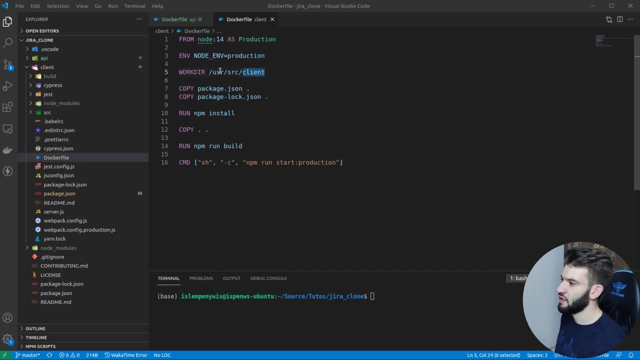 Just like go ahead. Oh, I know that I'm putting my code in in some of these like user associate client directory, So yeah, Why wondering? So just like access the um the shell of the Docker container or running Docker container. 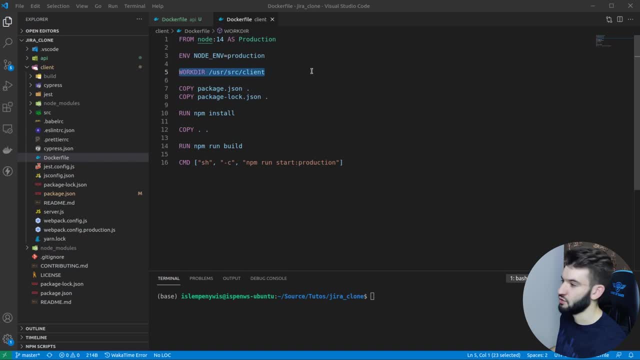 and you can directly go into this directory and find some logs or debug something inside of there just to know what is exactly happening And, of course, copy back packjson. Okay, So let's go ahead and run npm install, run the build and run the production. 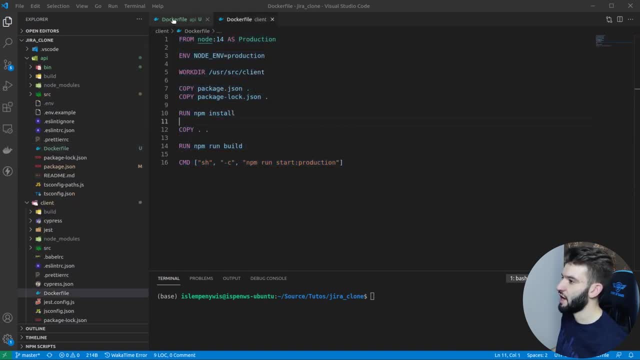 Pretty sweet. So there's basically identical both of Docker files on how they should look like and how they should run. All right, Pretty sweet. Now to build this images. all we have to go ahead and run is actually the Docker build. 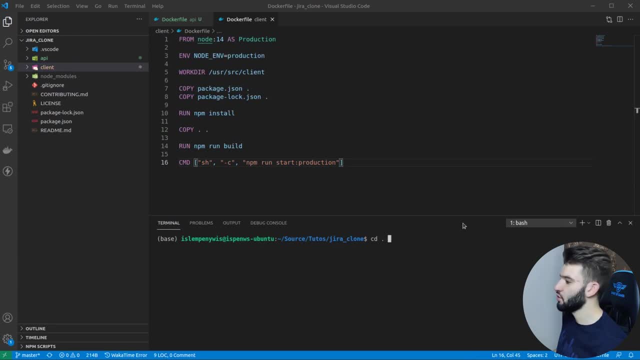 Now, for example, going to CD into um, the actual clients. So I'm going to do CD clients and I'm going to do Docker build and you give it like where the directory that build resides in. Of course it is inside of that cause. I actually it's going to see, it's going to run all these. 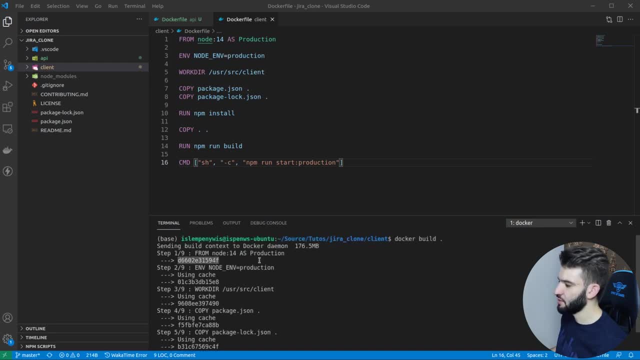 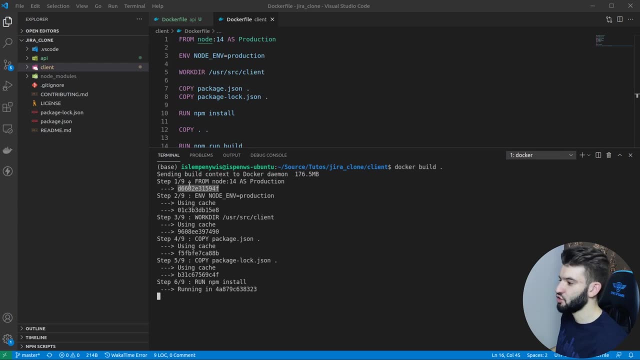 commands. It's going to run, uh, from nodes, So it's going to grab this node and if it doesn't exist inside of your machine, so what it does is going to go ahead and pull it from the Docker register, the Docker hub it brings. 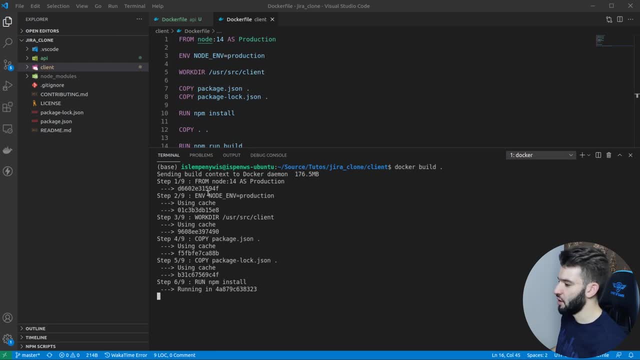 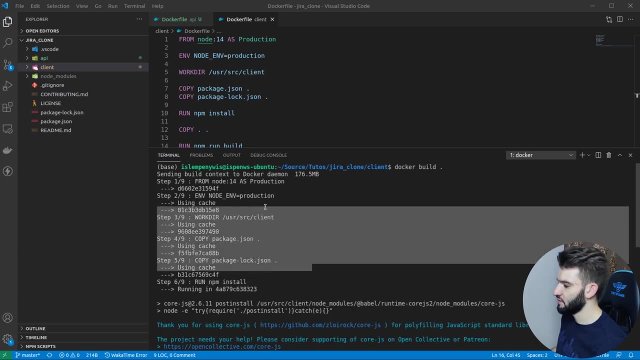 it first. then you start building, But for me it's already there. I already use that. So yeah, that's, that's all good. I was curious in here just installing the dependencies after copying back to json and everything. 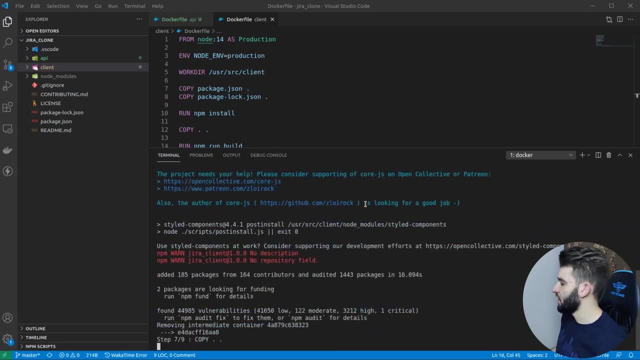 It starts, you know, doing some regular NPM install stuff, uh going on behind the scenes and everything. So now it's copying the whole source code, So it's copying basically everything right here, uh into the actual container, and that. 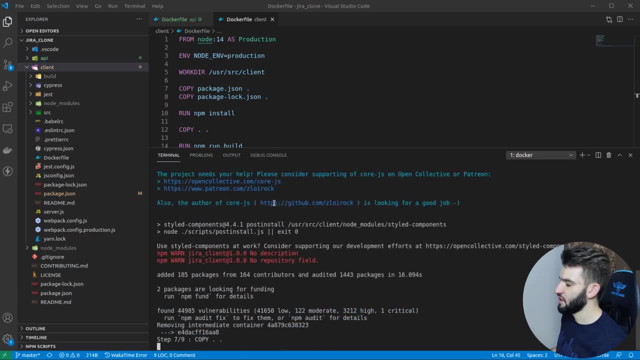 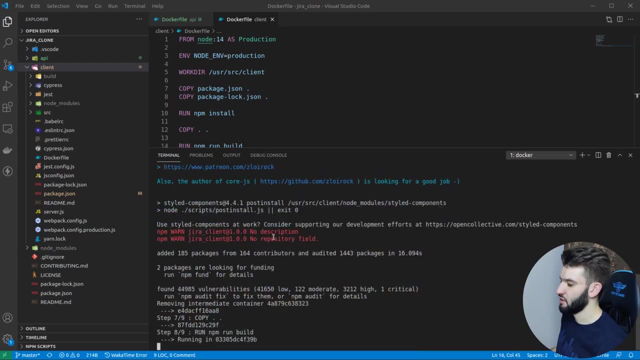 should build the whole image for us. So just like wait a couple of seconds. of course, the build might take a second to a minute, depending on how, uh, how much big the project says and everything. So, yeah, that should be a. that should be all good. 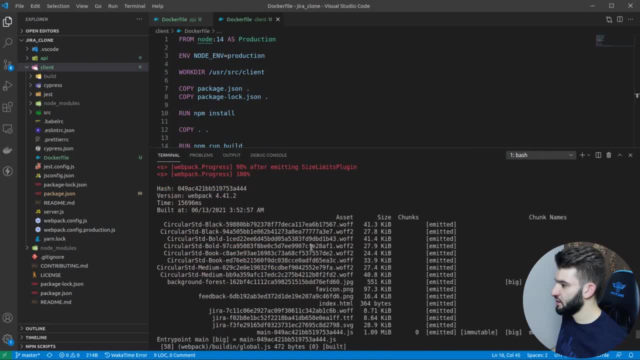 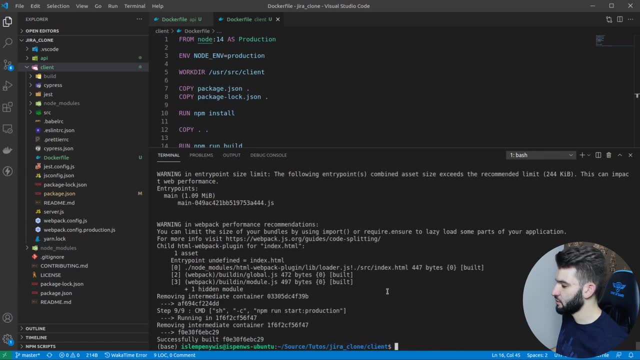 I was curious in here did the whole build after installing dependencies. So it did a full webpack build for building the all assets into a production ready kind of a distribution folder. And yeah, so the building is actually successfully done for building the image. 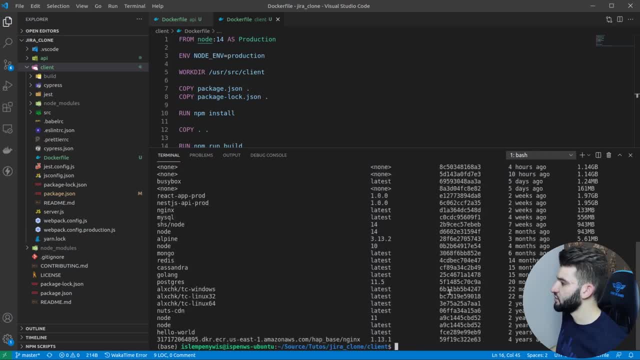 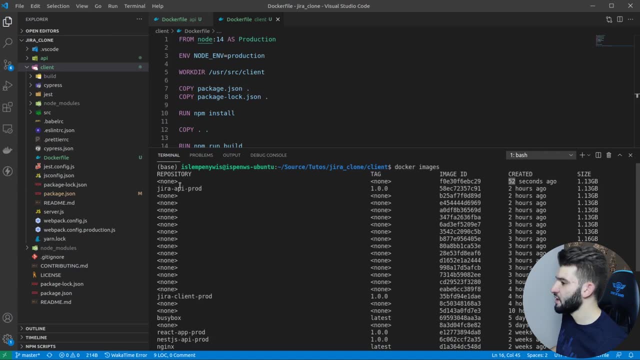 Now let's check out the image. What we can do is actually Docker images, and it's gave us the list, So just take a look on the most recent one and there you go. So there's the, the number of seconds that we created, and you see none in here, because 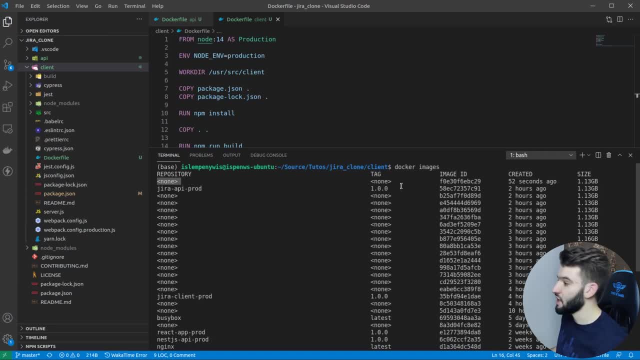 we don't have a. we didn't send it any kind of like tag or a name for this image. We just said: Oh, Docker, you got this Docker file, Go ahead and build me this. And we didn't actually specify anything. but what we can do is actually go in and do like. 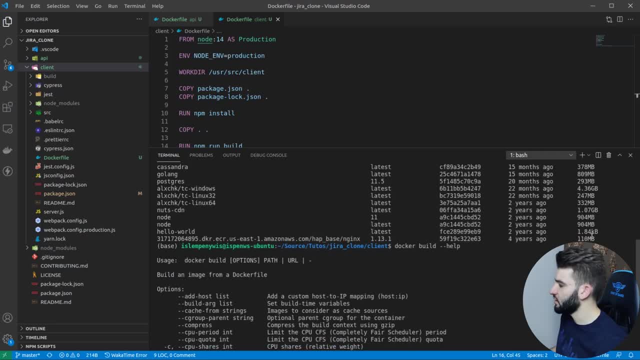 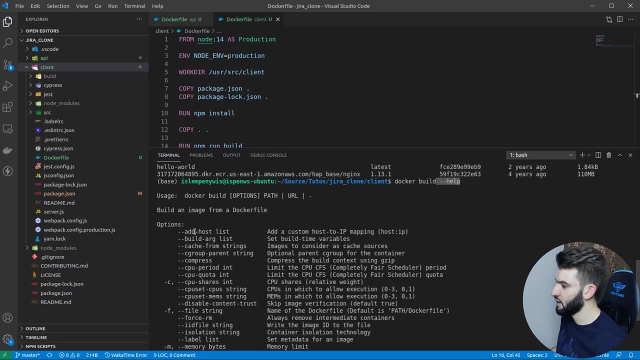 Docker build And if you want to check, for example, what kind of like um flags are in there, So just like, do Docker build, dash help. This is actually going to give you everything for this build command and what you can tweak. 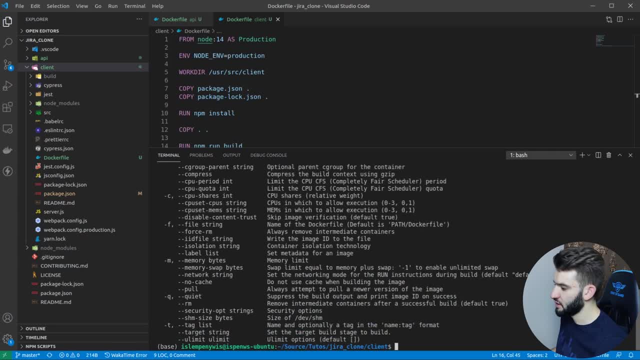 And, for example, we can take a look in here: um, where is that? So? um, so you can seriously need to set a tag which is going to Name: is for an optional tag in here that what you want for your particular image or you. 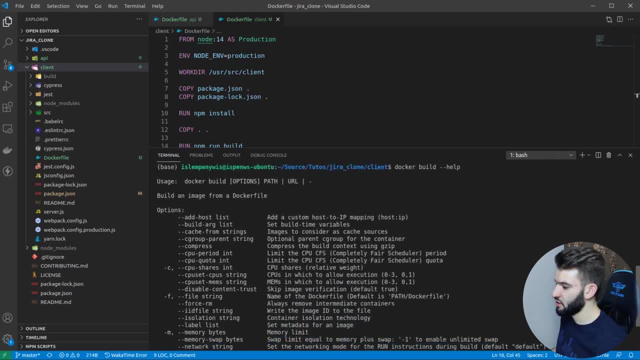 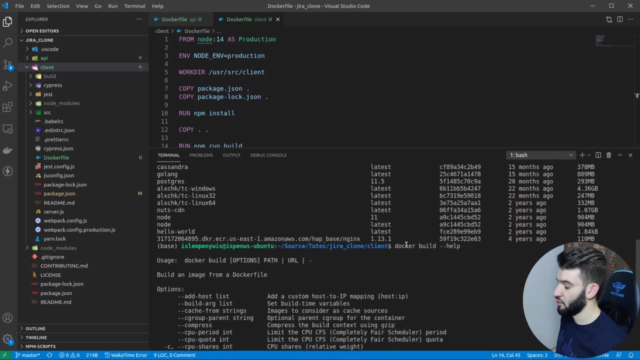 can give it like a name or flag what the name is, So you can use a dash and or and name just just to name this and how you want the image to be, uh, or the build image to be eventually, and how it does it look like. 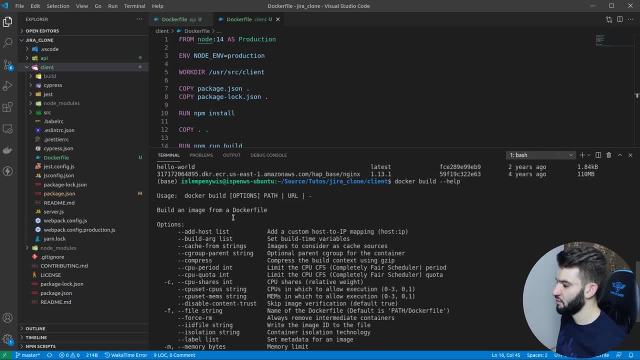 All right. So that should be all good for this, this Docker build and how it builds out the image and it puts it inside of like your own kind of memory. Of course, you can take this image after like building and everything. You can go ahead. 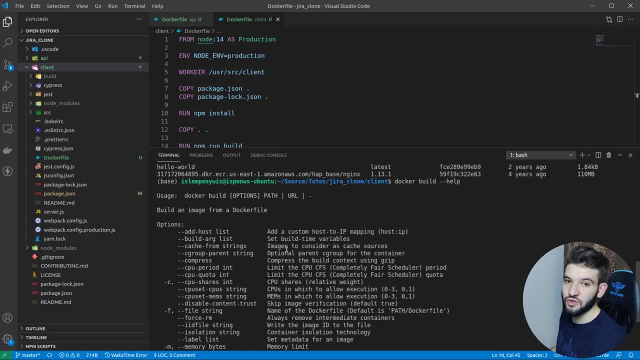 And then push it into your own custom repository on Docker uh registry hub or on your own private repository- Why not? Or on Amazon, ACS or something like this. you can. you can have it actually pushed out there and you can reuse it whenever you need. just put it out and you can run it on your servers. 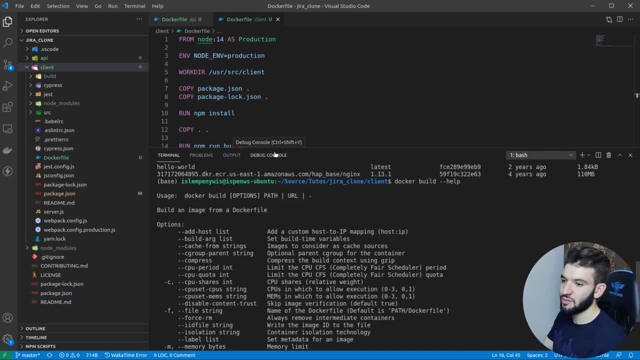 or whatever. So this is basically how distribution works. Of course it's a little bit more complicated with pipelines, CI, CD and all that sort of like dev ops things. But yes, this is. this is. This is basically how Docker is being deployed and how it works with this kind of built images. 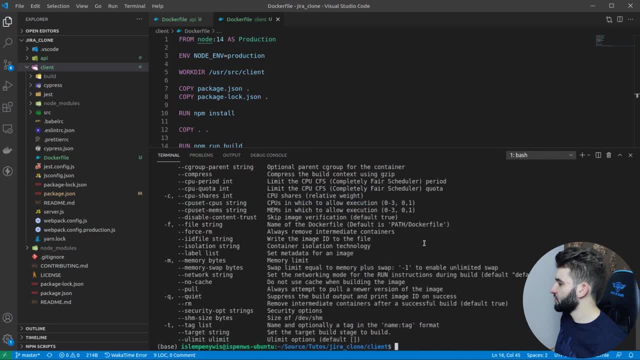 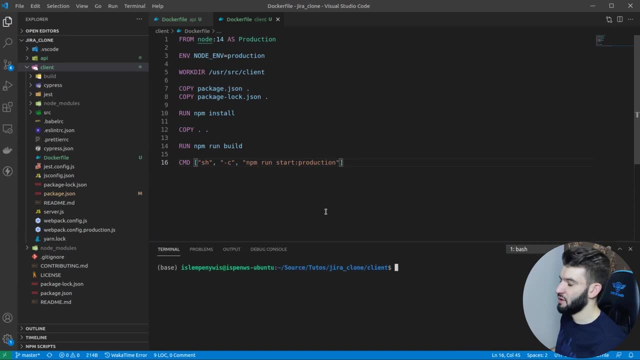 behind the scenes. All right, Pretty sweet. So we've got the build and how to build this from a single simple Docker files, But what it wants actually we don't want to do it this way, because this is actually kind of like horrible way to go go ahead and build this uh, particular folder or particular. 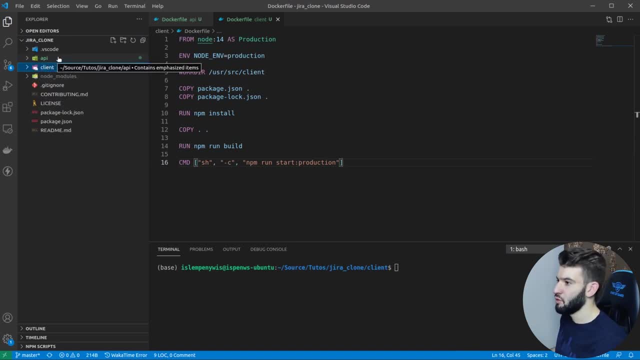 Docker file, like the client's one, then go to the API, build it alone, then just like, have all the bills, Then go back into, like, running each container by itself, Putting a bunch of commands that you probably can actually forget about, and all this sort. 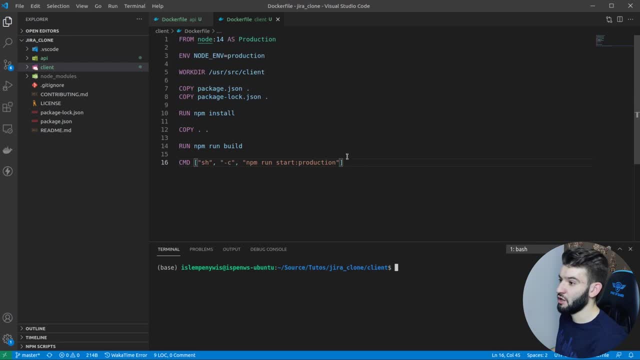 of stuff that doesn't really make it that good to use Docker for deployments in this big projects. So imagine, for example, for this particular case, we've got the client within API and the API basically needs behind the scenes a Postgres server running on the local machine. 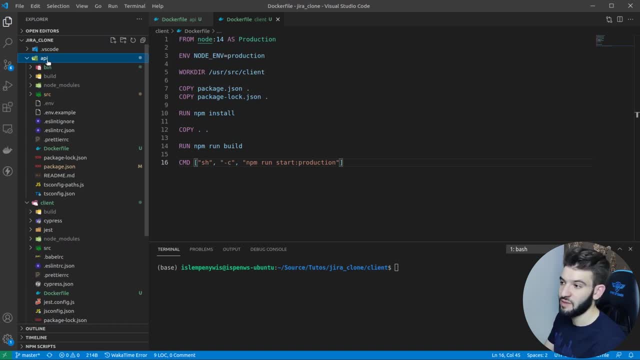 or on the local host, in order to be able to connect and start up the API. Otherwise, the API will fail and you won't be able to connect to that particular client. So that's what we're going to do: We're going to connect to that particular database. 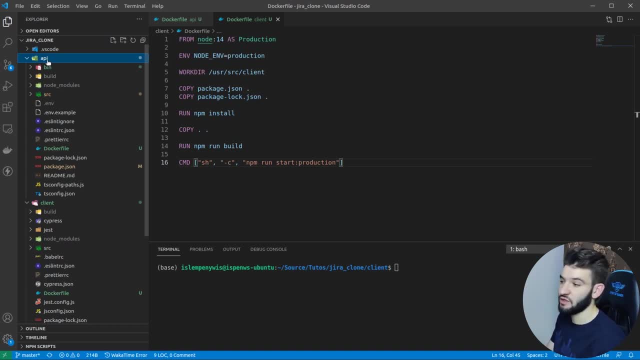 So we need actually a Postgres kind of database already started. It doesn't matter if it's Docker or not, but of course Docker is preferred because everything is in Docker, So make sure to have your whole stack in Docker. And this is where Docker compose comes into the play. 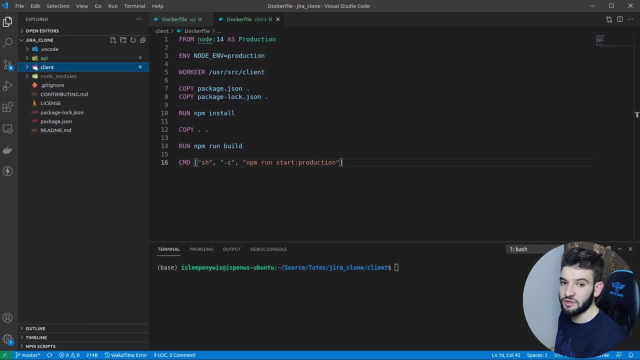 So what Docker compose is pretty much like relies on a, on a Docker engine. So it just like allows you to have all of your Docker kind of like uh, kind of builds and Docker files, like little, these Docker containers, for example, for the clients and API and a. 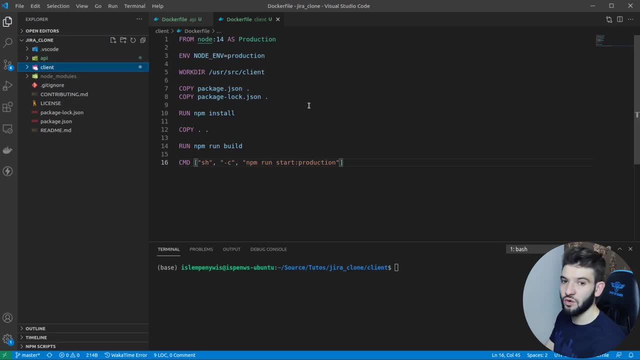 Postgres, which are called services. So have this, all of these services combined together into a single simple, minified and really well structured file with the whole kind of configuration, the whole kind of commands to run. uh, images tags. 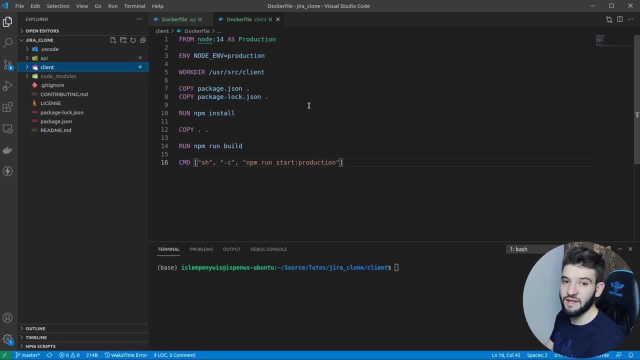 You can have them like with volumes and different networks, set up everything inside of like a simple, easy and custom YAML file. Yeah, That whole configuration, all these services- So this is basically what Docker compose- is just like a CLI that allows her to manage. 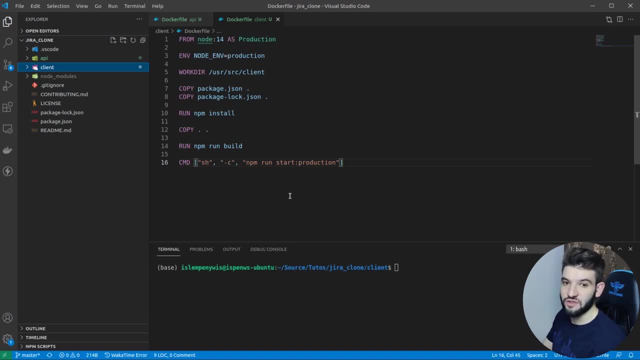 and read this kind of like YAML file and pretty much run these services alongside the Docker engine. Of course, just going to like read the YAML file and just like provide everything to the Docker engine in a really nice and smooth way. So first things first. Docker components is not a start with the Docker engine, just to 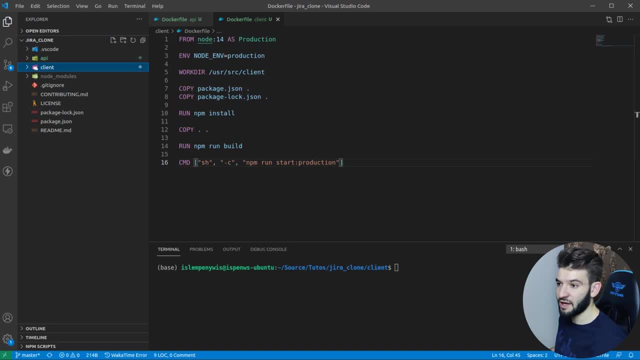 be sure And to be clear, uh, for windows and Mac, yes, it is throughout the the whole disk stop installation kind of tool set. So, as soon as you just like, install it once you get it everywhere. So, windows and Macs, you're good to go for Linux. 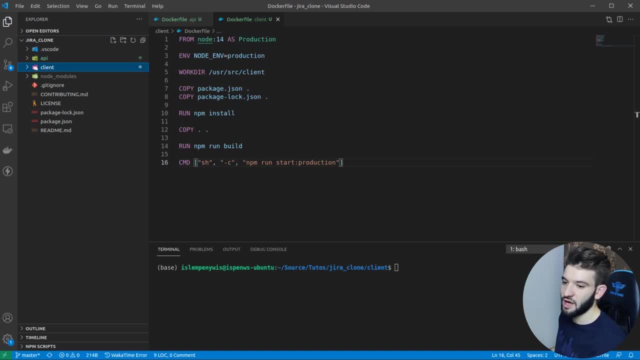 Like me? Well, you're still not. You've got to just go ahead and install this again. Of course, you can go and install this um throughout different ways, but the most perfect way is actually to go in and follow up the documentation. 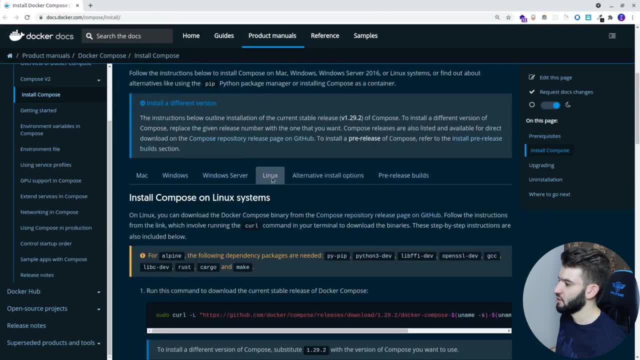 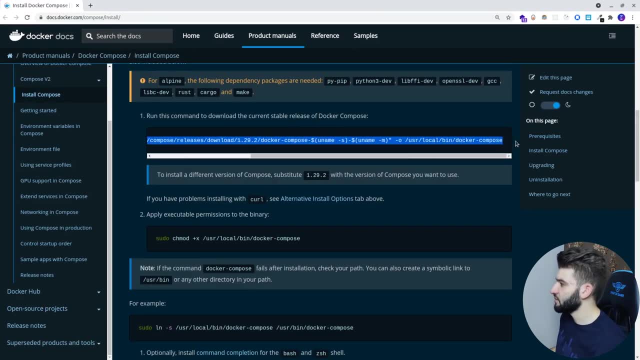 So let me just bring you the documentation real quick in here on how to install. So I chose Linux in here for a started Docker compose and this is basically what you need. So go ahead and like, run the studio Scripts, which is just basically a simple script that allows you to, um, basically have. 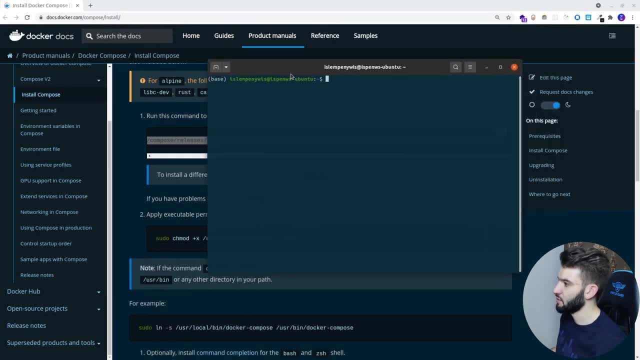 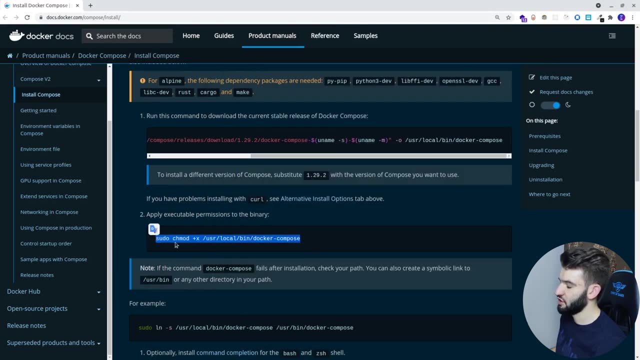 the Docker, compose CLI running throughout your shell just to install a couple of stuff. So you can go in and run this one, uh, which I already did, of course, And then you can go in and change the like, use the change mode, which is like changing. 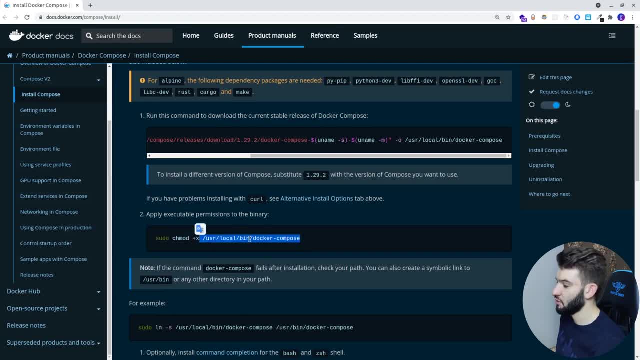 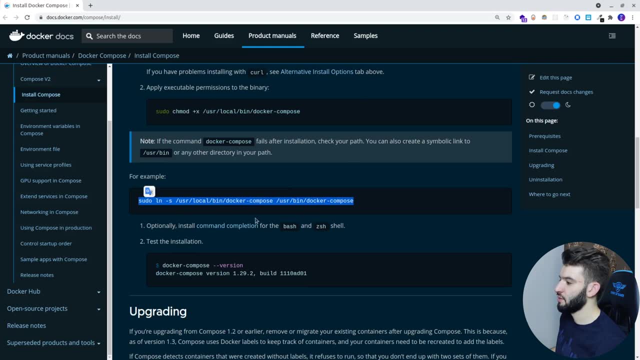 the permissions for the Docker components. that is already put inside of, like user local bin Docker compose, So just put it there. And last but not least, you can go ahead and like do a pseudo that compose in here Just to complete the installation or everything. 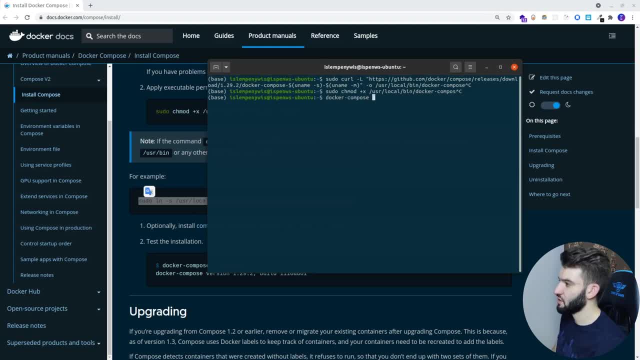 Then yeah, that's it. Just to make sure that the proposed install, after running all these commands, all you have to do is go and do like dash V is going to give you. oh, that could compose version 1.29, whatever. 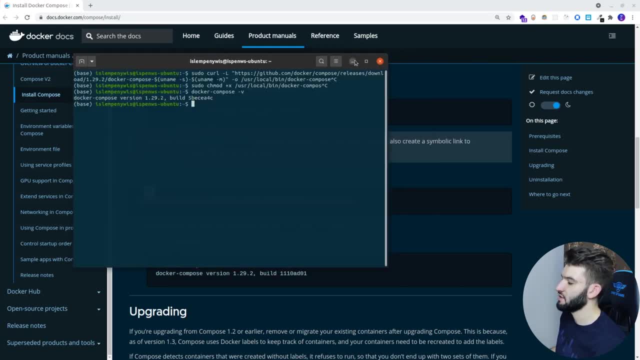 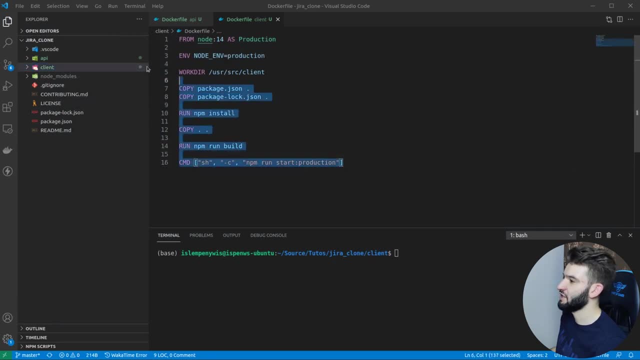 And there you go, So you make sure that dark compose is actually running inside of your machine. Okay, Hallelujah, We've got Docker compose. Now let's go ahead and start composing our application throughout Docker compose. So what I want is for you to have, uh, another file. 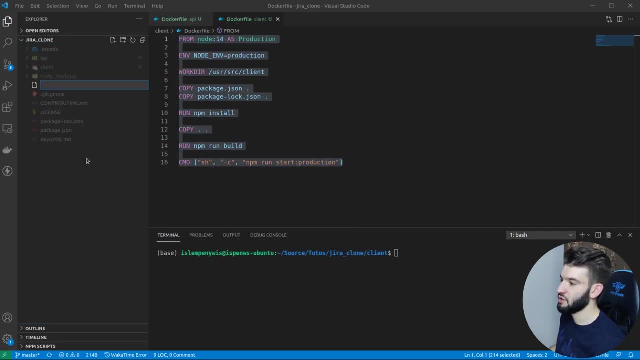 So let's go ahead and start composing our application throughout Docker compose. So what I want is for you to have uh, another file Instead of the root folder, because this file is going to be a Docker compose. It's going to be linking both the clients and the API in a single place, plus the Postgres. 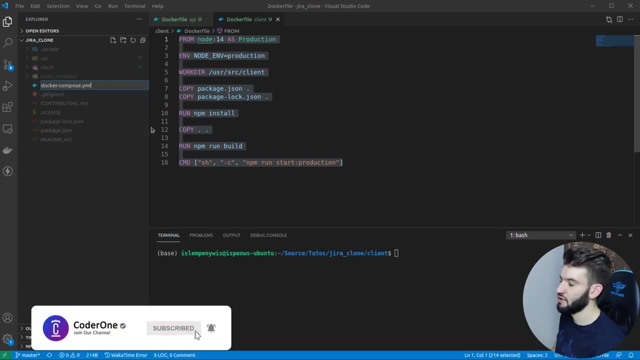 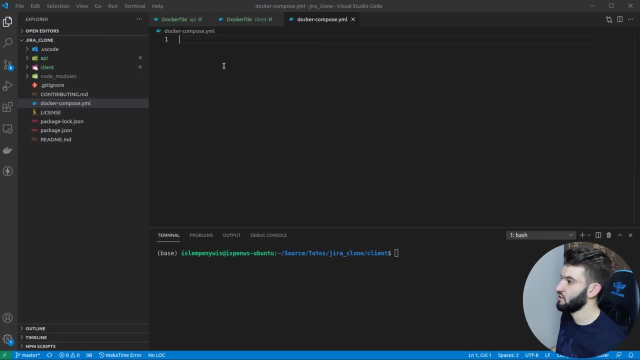 server as well. So I'm going to have this life code, Docker, compose, and this is pretty much the um, the kind of, like you know, standard way to pretty much name it. So make sure to like use a standard name in here, because that's, that's really, uh, really. 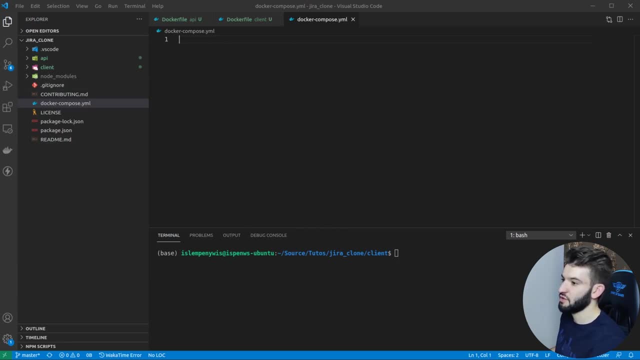 well, in compliance with developers and all that sort of stuff. So this is pretty much for the YAML and how it looks like. Now, if you're not familiar with the Y or the YML kind of like syntax or how it works, just like, basically, if you're familiar with JavaScript on how kind of like key value pairs. 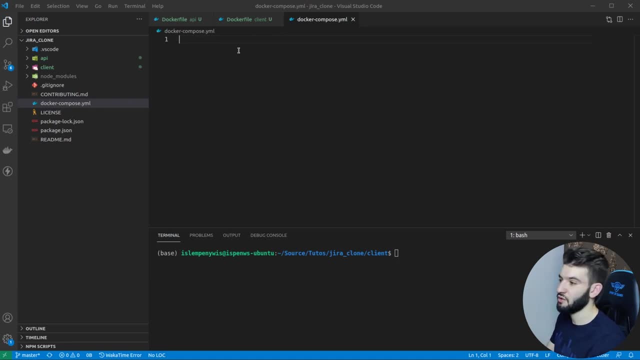 works. that's basically what it is. Just like I give it a key, then I give it a value, and that's it. Now, to start off, we're going to have to first define a version and what type of- like Docker Compose- version we're going to be using. 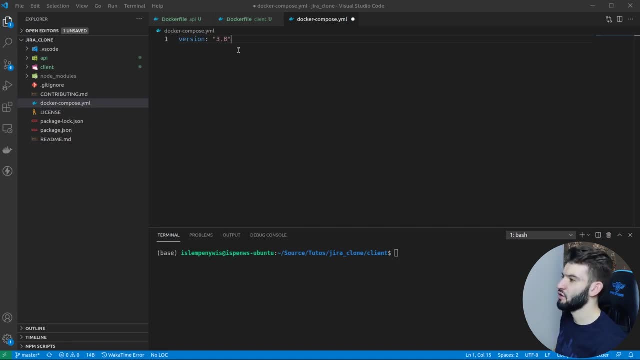 The last version, as far as I know, is either 3.8 or 3.9, so I'm going to use 3.8 respectively in here, because it works really well, And the second here, the second directive I'm going to call is going to be the services. 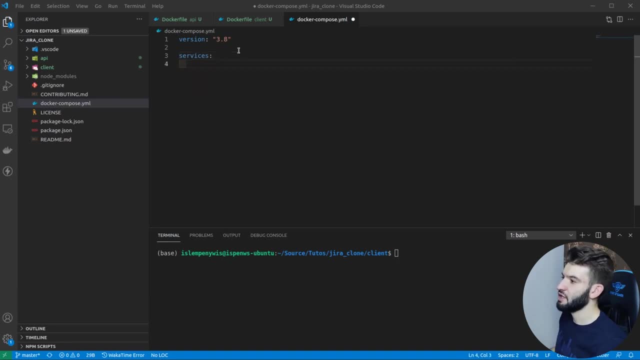 which is the most important one Now. services in here are actually each service or pretty much represent each kind of container you're going to be running. So, for example, the client is actually a service, the API is a service and the Postgres. 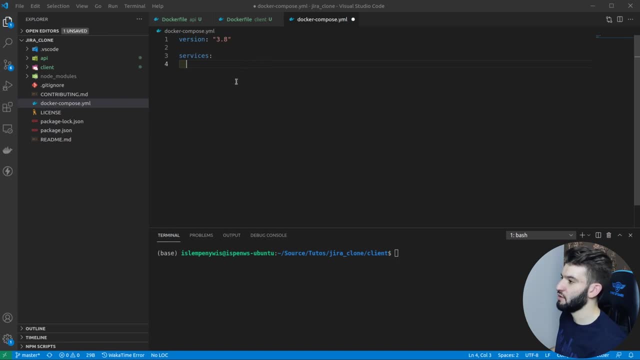 server is a service, So I'm going to put in all of these services behind in here, with a different configuration from one service to another. So for this experience I'm going to be using- I'm going to name this- Postgres. 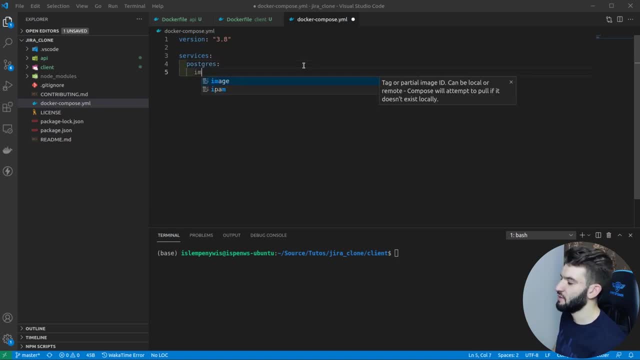 You can give it whatever name, however you want. So this is going to be the Postgres server. Now here I'm going to give it the image. what like the image name I'm going to be using for this particular service, like what image name I'm going to use it to run this Postgres. 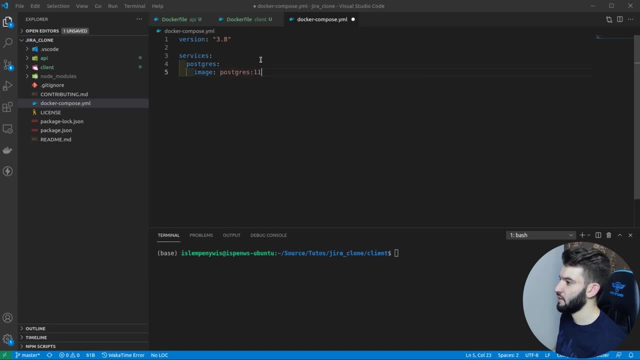 service. So the image name: I'm going to use Postgres and I'm going to use 11.5.. So the same way we did it before when we did like Docker run and everything. So this is basically the same way how it should look like. 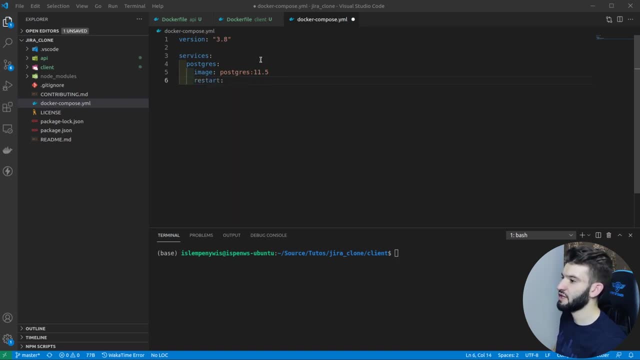 So the second one: I'm going to use the restarts and the restarting here tells it, like when to restart this container. So what kind of condition happens to restart the container? I'm going to do always. So anything happens, any crash, anything happens to the containers is going to pretty. 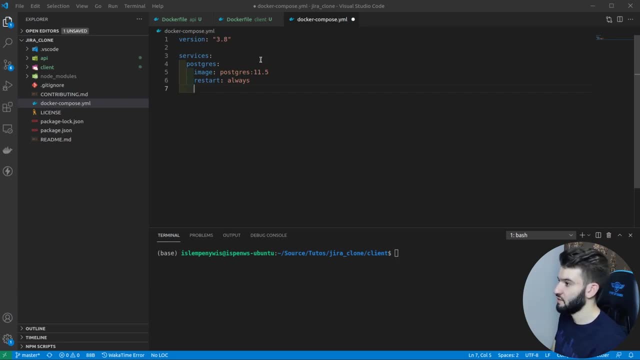 much allow it to always restart the Postgres, because this is very important. We want always to make sure Postgres is actually up and running, Whatever happens. All right, pretty sweet. We've got another one, which is called environment. Now, environment, here you give it, like, what environment variables you have, and as we've 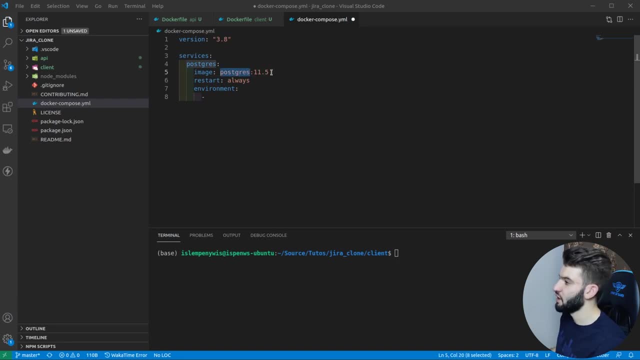 seen before. Postgres in here has a couple of environment variables to make it work perfectly, For example the Postgres password, which sets the actual Postgres database password for you. So that's why you want to pass in in here. 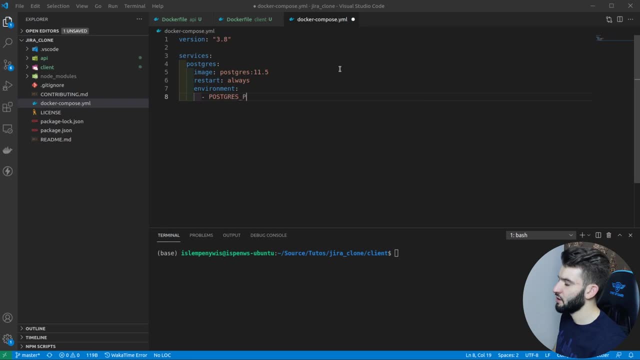 So, for example, we're going to put Postgres password and you give it like what type of password you want, excluding using this like dash in here, which just basically annotates and tells that we're going to use an array kind of type in here, because there's different. 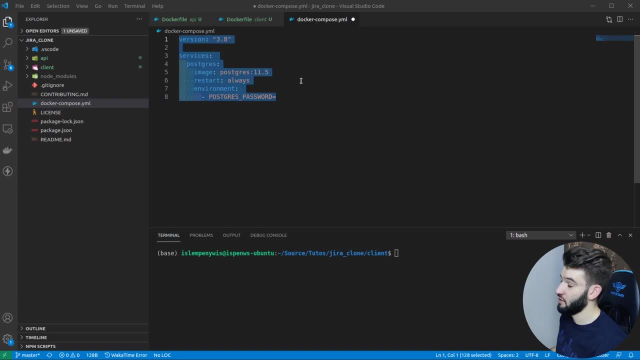 types of this YAML format if you're not familiar with that, but that's basically where it is. So, for example, you give it a password like 123, and I want to use another environment variable which is like the Postgres DB, which basically tells it what is the database name. 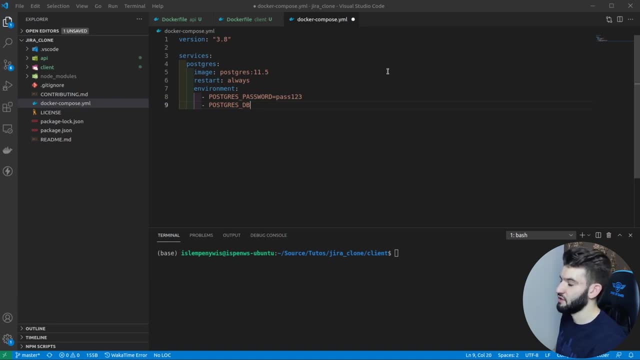 I want to create by default Once I start up this particular service. so I want to, for example, create a database called Jira development which is going to be used for our, of course, our- API kind of clients in there to connect to. 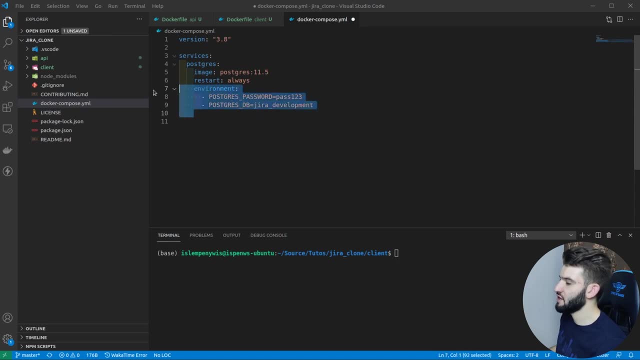 All right, Bruce, we've got the environment variable and this is what's going to be created, and set it up for us on the Postgres kind of image. So, and if you're actually saying, oh, how do you know this? like, this is the environment. 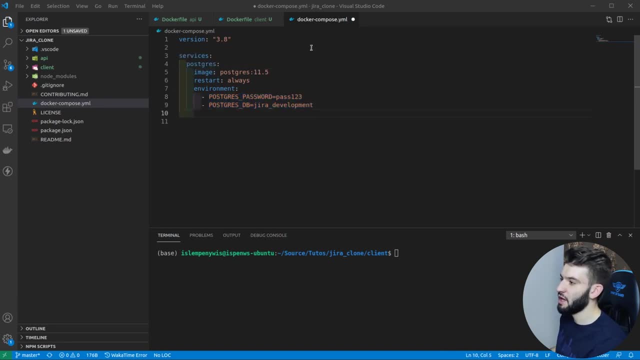 variables and how do you know all that sort of stuff? Well, this is all about, like the Postgres, This image, and of course it depends on every single image, on how it works. So make sure to check out the documentation, or pretty much the docs, or the description. 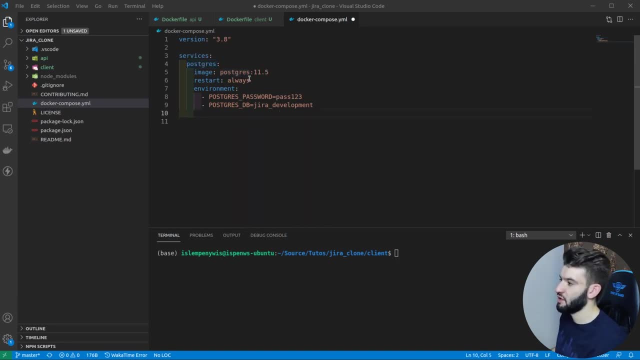 of the image on the Docker Hub or whatever other image, before jumping through, just to give you all the details on how that works. All right, The other part we want to do is actually the ports, and this is pretty much: we're exposing ports. 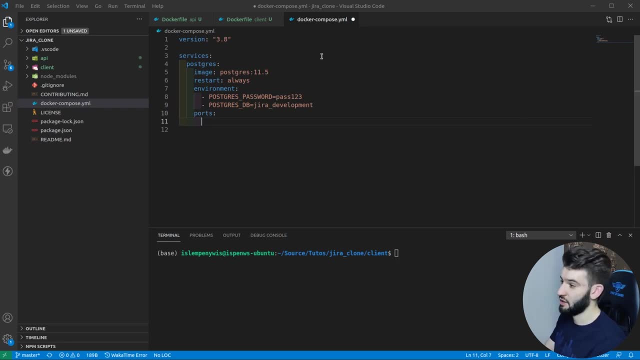 So, as we did it before, where we expose ports like expose internal ports to the export, like external ports, Another part where we do it in here and I'm going to explore basically three, or the same port pretty much from outside or pretty much from inside, which is this one represents. 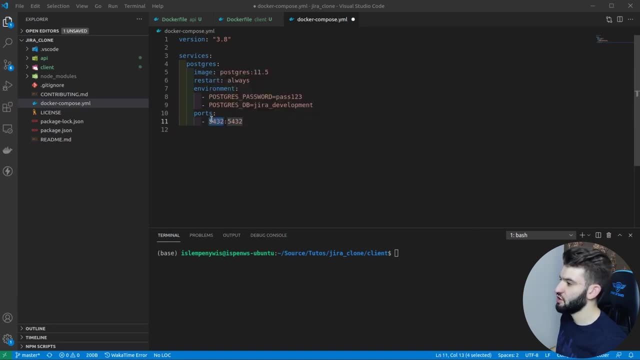 inside of the container to outside the container, to our host machine. for this one You can of course choose a custom ones, but that doesn't really really matter for that particular part. All right, We can use networks now, for example, for networks in this particular part. what we can do like 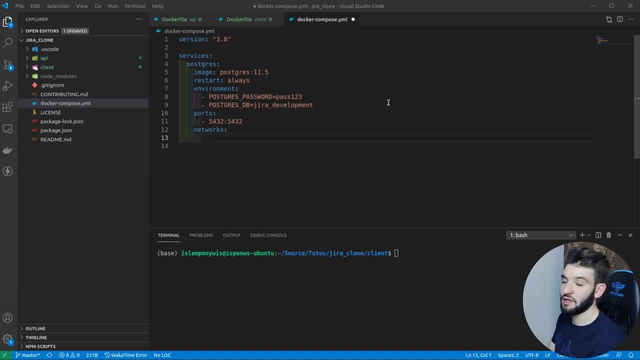 if you're familiar with Docker and how it works, You pretty much there is this by default, or shared network between all the services or all the containers running on the house. Well, of course, you can create custom networks. In our case, what I want is actually create a custom network, but still I'm going to use 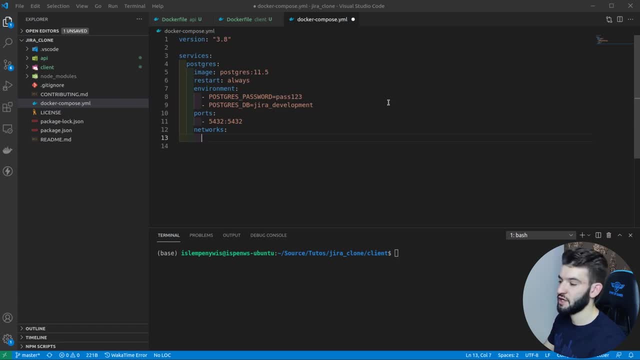 the same network for all the containers or for all the services to connect to and communicate through, and to be the whole containers running on the same network to be recognizable, if that makes sense. So I'm going to name this my network. I'm going to name it shared network. 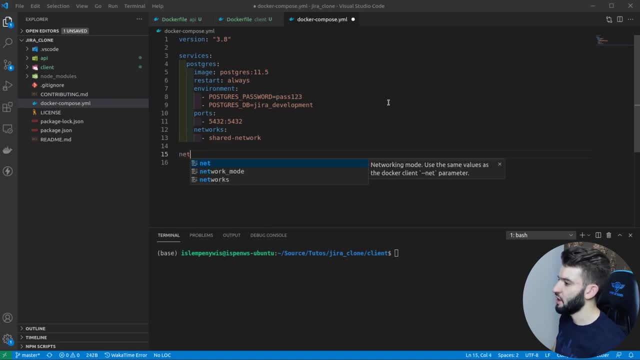 I'm going to create the network. I'm going to create the network in a sec. So to create a network, just put in another network directive in here which is the same level like on the root level or the same level of the services. 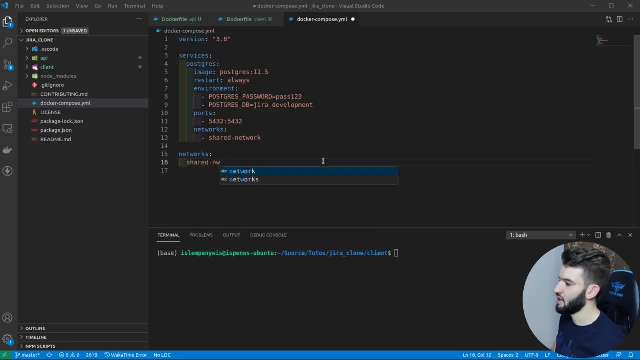 Just don't be mistaken and put in like a shared network, the same name And this is you. make sure you put a column in there, because this is the creation, like he'd sign that. Oh, this is the objects of it, All right. 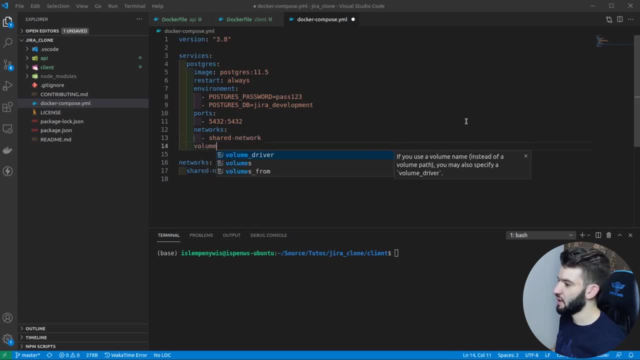 Pretty sweet. Now we've got the network and everything. Now, last but not least, and this is only specific to this- Postgres. if you're asking why now you need a volumes Now, volumes in here is like the volumes to be created as part of your application. 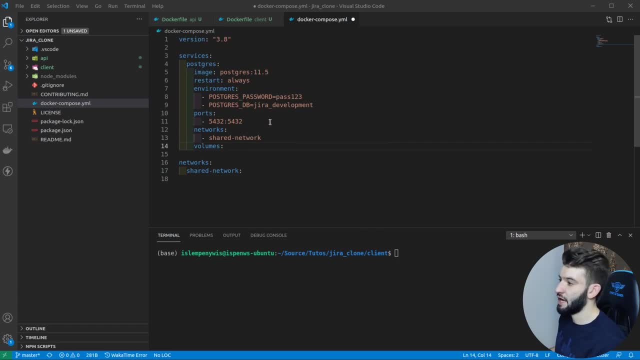 So the volumes, what it does? it basically actually exposes data inside of the container and binds it or links it to another kind of like directory or a file outside of the container, which what I mean by outside is actually on the host container, on the Linux machine, in. 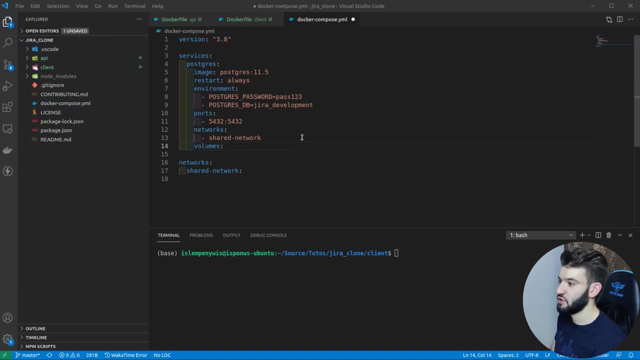 here and this for this, for this data to be actually persistent. That's basically why- Yeah, I should be looking like this way, So I want to make sure it's persistent. and for databases, this is a very, very important step because it's going to allow it to expose data, because if you lose the container for 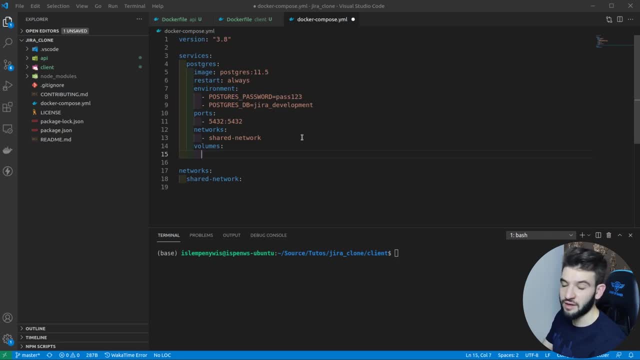 example, if you remove the container or the container is stopped, you're going to lose data and you don't want to use your database data. This should be really, really bad. So make sure to use volumes to actually bind data inside of the container which is going. 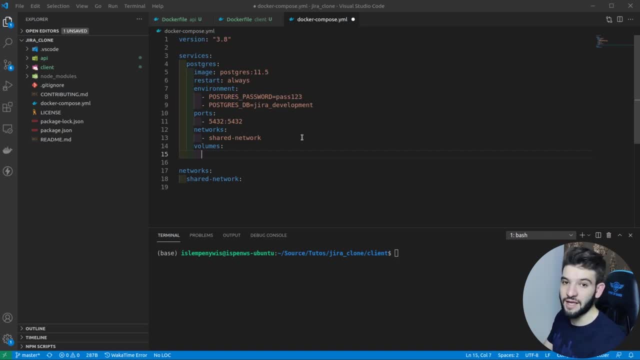 to represent the actual database data and bind it or link it outside of the container. So the data to be written in outside of the container and to make it persistent to live outside of the container and inside of your server, if that makes sense. 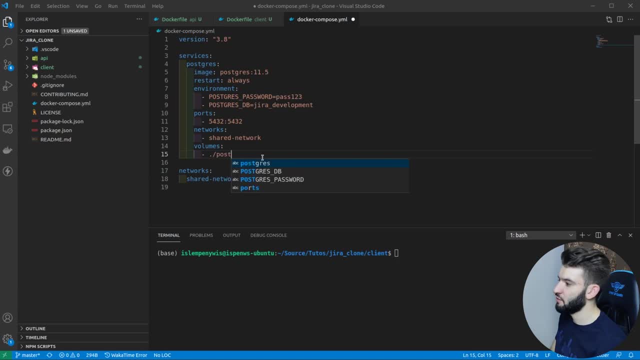 So just the volumes in here, what it takes. it takes a directory where you want to put it, For example, when I put it, for example, Postgres DB. so I'm going to create this folder and I'm going to link it to the data file or the data directory where data exists for the Postgres. 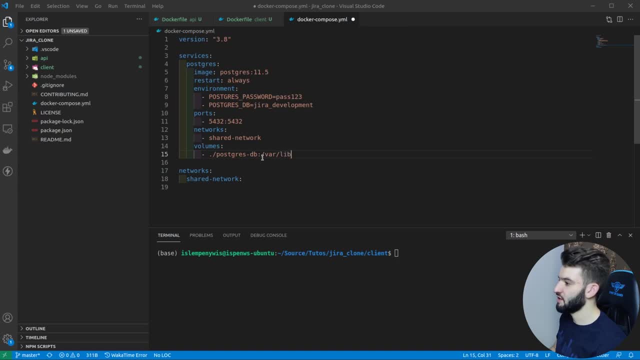 inside of the Postgres container. All right, So it exists inside of var link. Yeah, So let me show you what this is going to do. So this is going to do a simple pimp and Postgres, SQL or PostgreSQL, whatever you want to call. 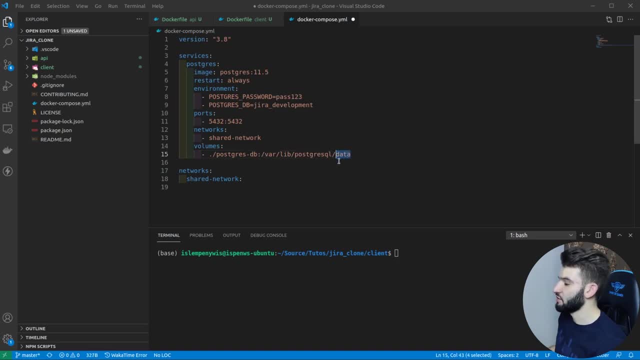 it and for slash data. So this is the folder or directory where the data is going to be put from the Postgres database. I'm just going to link it to this directory, which is going to be created for us right here on the loop rebel automatically by Docker, so we don't have to do any other further steps. 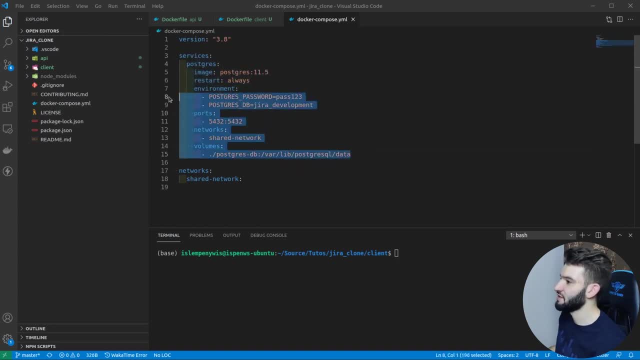 Sweet. Now we've got this Postgres service already done for us in a really, really awesome way. So we're going to go ahead and go ahead, and go ahead and go back to the Docker server to see how it works. way like it. okay, I'm gonna copy this one. I'm gonna create the rest of the. 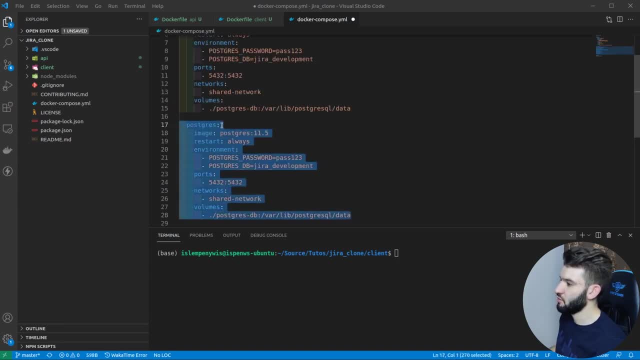 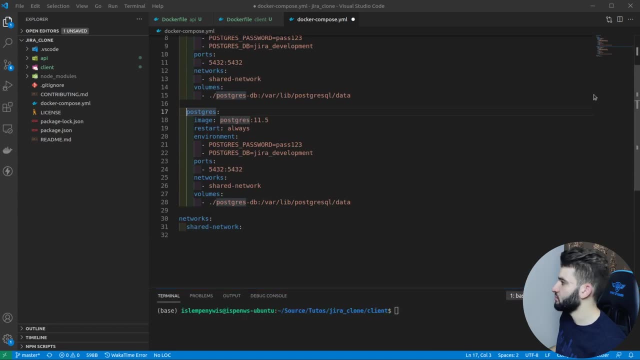 services. now the second one: I'm gonna make sure, like always, to match the levels, otherwise it's gonna like yell at you with random errors, and you don't want to do that. no one loves yelling, okay. so the second one in here: what it wants is actually to run the actual API, and for the API we're not gonna use an. 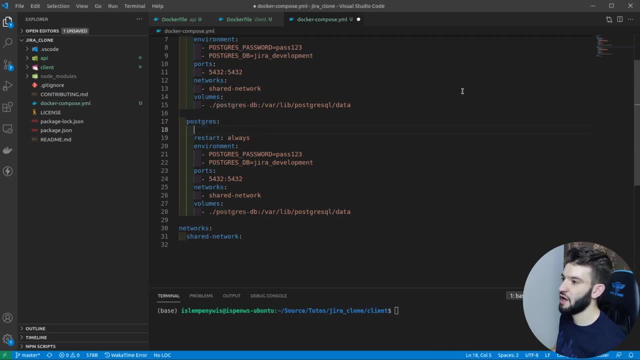 image. so I can completely get rid of this, because we're gonna use the docker file to build everything. because we've got the docker file in here. we're gonna use this docker file, tell each: oh there's this docker file and take me this docker file and build me everything I want it to be. so I'm gonna use this. 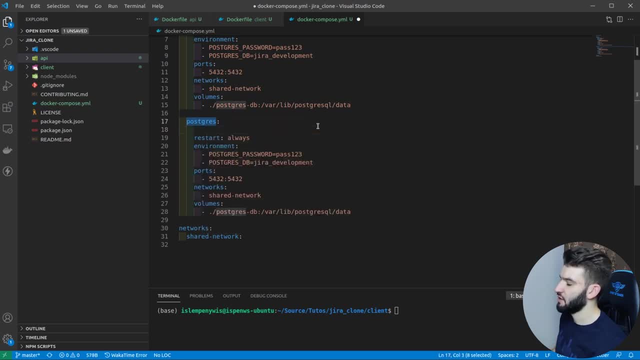 I'm gonna tail, for example: oh, let's go and change the name first. their name is API. I'm gonna give it container name. like what is the container name? I'm gonna be naming this after run it. let's say, I'm gonna name this, for example, the: 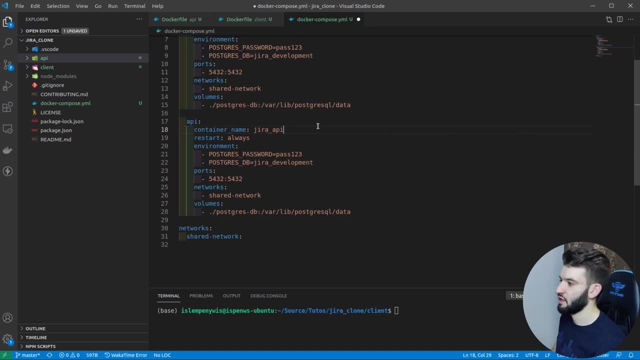 JIRA API, just just to be agnostic and kind of like, simple, for the RST Hill starts, I'm gonna do endless stops, so only restart this once it stops, just to make sure that we always keep it update and always keep it running. for the image name I'm gonna be creating, I'm going to name something. 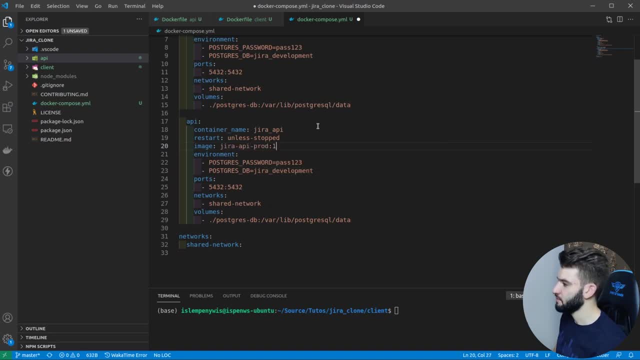 like JIRA-API-��S 0.0, just like for some simple versioning. alright, the second one. I'm gonna have a build this actually, So I'm going to get rid of this. Now for the building here. it tells it how we're. 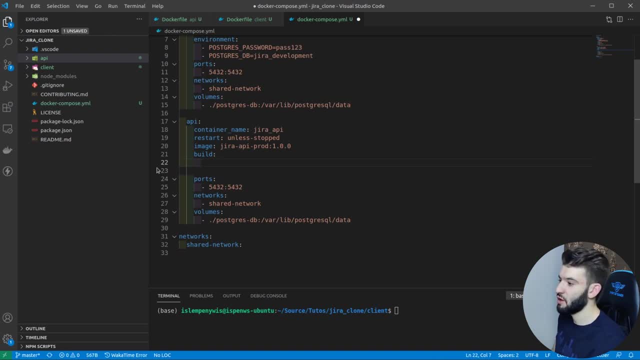 going to build, like tells it what is the Docker file, or which Docker file we're going to be using, and the context and everything Now provide the context, which is basically represents what directory we're going to be using. So for the directory, I'm going to go into the API, So I 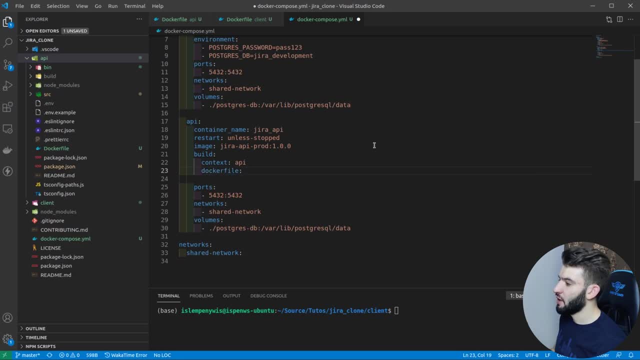 want to use this API directory For the Docker file. I want to use the Docker file inside of it which is named Docker file with a capital D, It's capital D And, for example, when I put as well a target like what is the target version I want to target in here I'm going to target the. 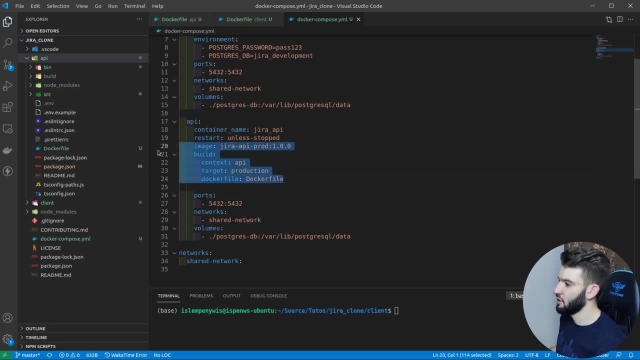 production. Alright, so that's, that's simply is going to tell it to build, to go into the side of the API folder and pick up this Docker file and build it for us. is going to build this API image for us in a really simple, easy peasy way. Sweet, Now the port in here. I want to export this port. 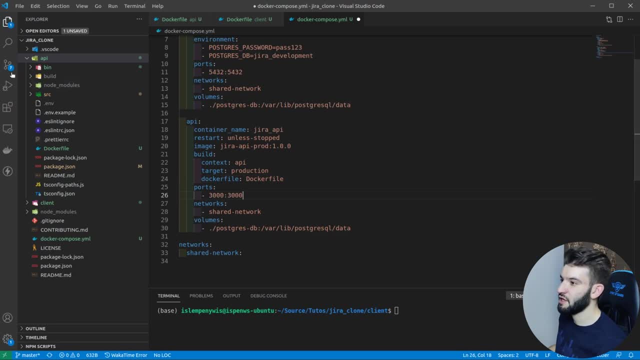 and for our server, for our application, like the API in here is by default configured to listing on port 3000 internally. So the of the container is going to have 3000. And I want to bind this 3000 to outside of the container which is going to be exporting to our host in here as 3000.. So that's. 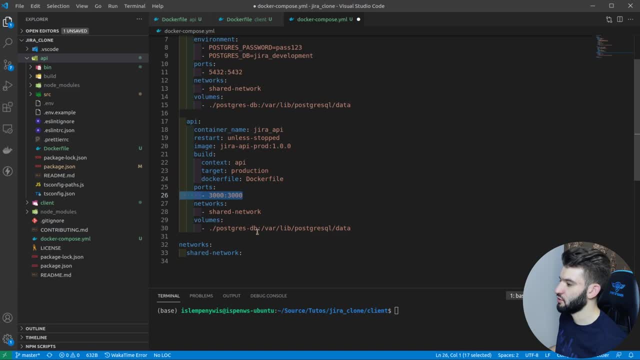 that's what I'm doing here And just like exporting this to be able to run all the plays there And for other containers to listen to. otherwise it won't work perfectly. For networks it's going to be shape: same shared networks and volumes. we don't need any volumes. That's it we. 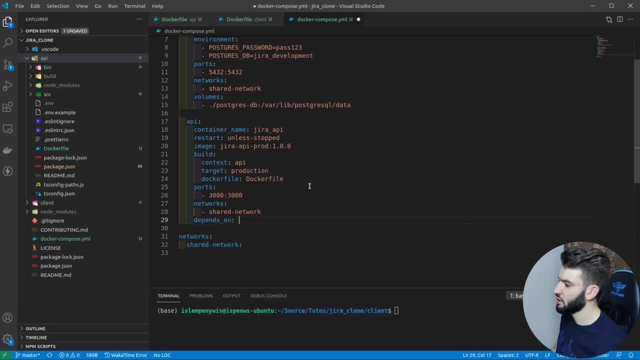 just don't need any kind of volumes, But what we need is actually another kind of attributes And this one it's depends on. So here we give it like a list of kind of like services of what this particular service depends on. like this API service has or needs Postgres servers or Postgres. 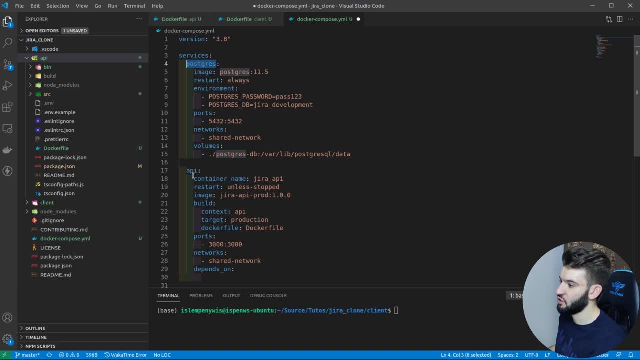 database to start up first before this API should start. Otherwise this API should just like wait for this. Once this is started, this API should start. So this is pretty much the logic. So for the depends on in here, I want to tell it: Oh, this one should depend. 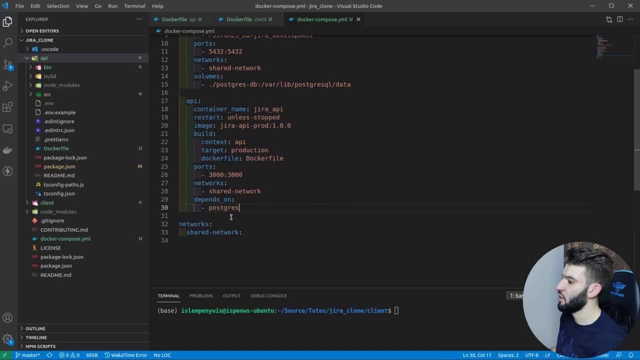 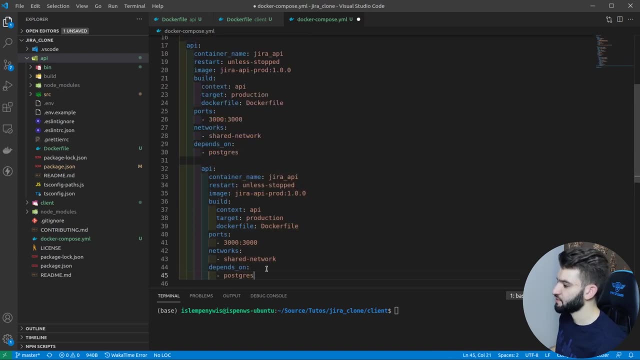 on the Postgres service, And that's it. So that's, that's basically what we need for the API in this particular sense. Now, this is for the second service. Now the search or the third service- sorry- is going to be the client, So I'm just going to try to be quick in his and copy paste it. 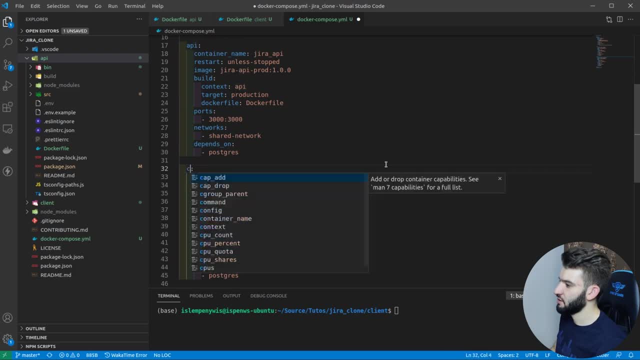 So just your API may be your clients, And here we're going to be a client, For the start is going to be the same thing: You're going to have a client as well. The context is going to be inside the clients folder. Remember, I'm gonna have it right there. 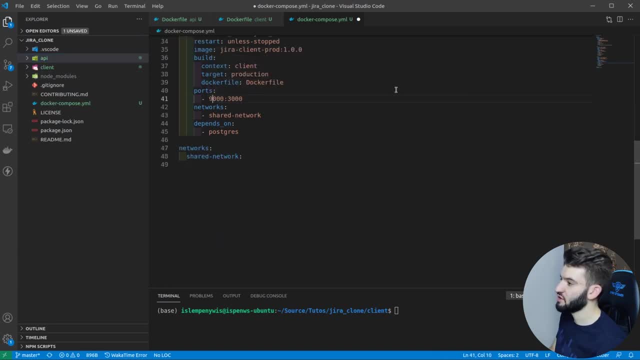 production and Docker file. the same for the ports. This one is going to be exporting. our internally is going to be running inside of like 8081. And I'm going to just like go ahead and export this to 8080 or something, just just for the sake of simplicity. All right, sure that's really going. 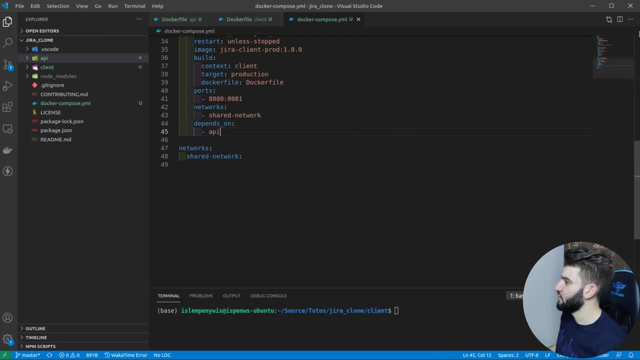 to be the same, But this one depends on the API For this one. it's going to be the same, But this one depends on the API. For this one. it's going to be the same, But this one depends on the API For. 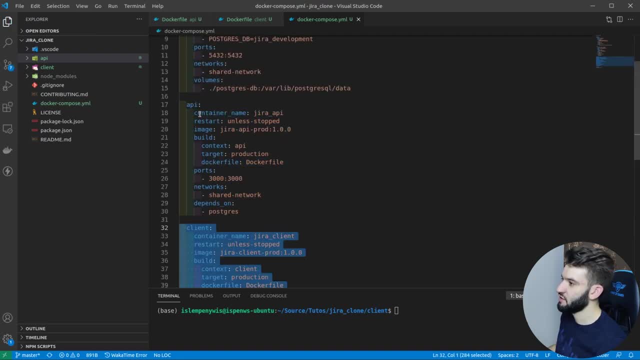 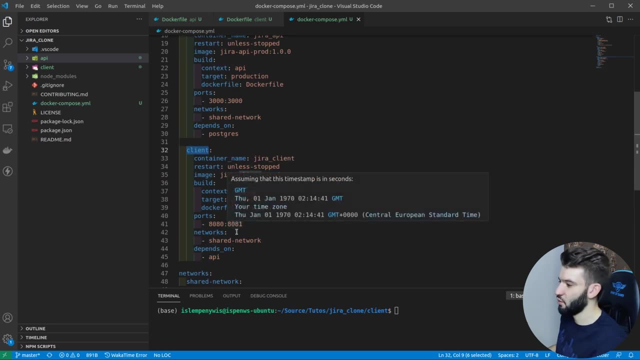 this to work, So he waits for the API. So they're pretty much like a chain, since the API waits for the Postgres to run and the clients was for the API to run. So it's kind of like a waiting chain. 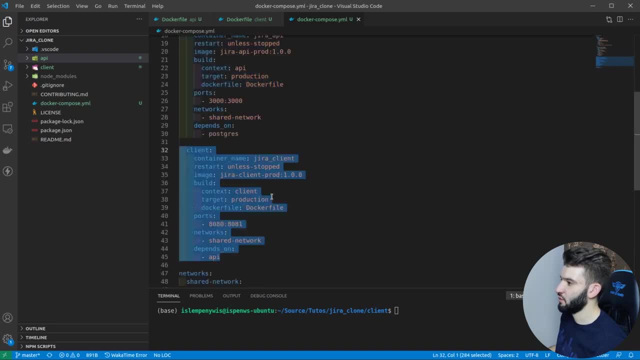 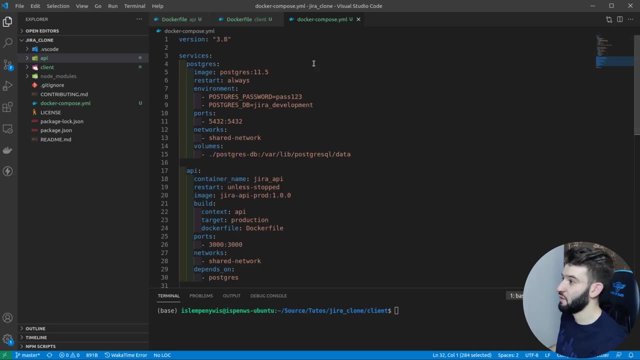 each one waiting for the other, And that's basically what it is. All right, we've got a pretty well made up configuration, our Docker compose, And it's pretty simple. Now, this Docker compose or this whole kind of services tag in here, what's going to happen is actually going. 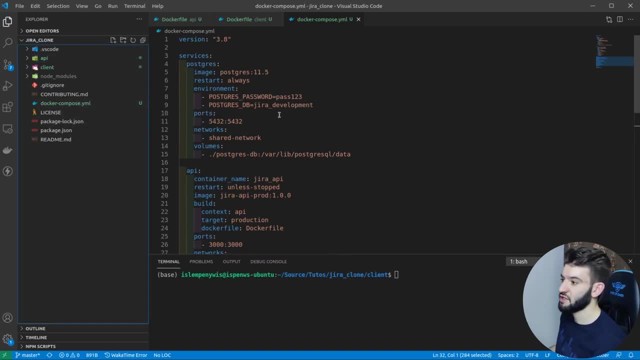 to end. we're going to run it on the, run it on the routing here, And what's going to happen? the Docker compose is going to take the file, read it and you know, oh, there's three services. So if there's like kind of like services or these containers are not already built, which means 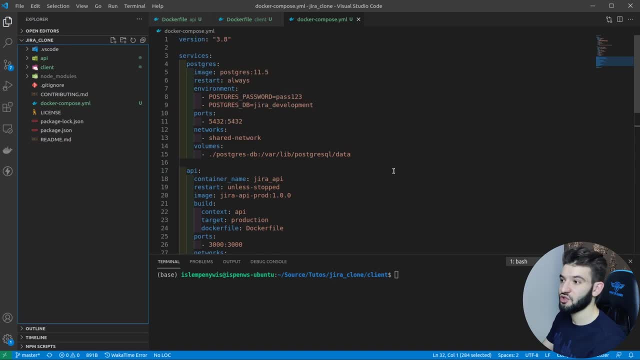 they doesn't exist as images inside of like system, is going to try to build them from scratch And after that it's going to try to go ahead and up those or like, start them. And it's going to start them, of course, depending on the 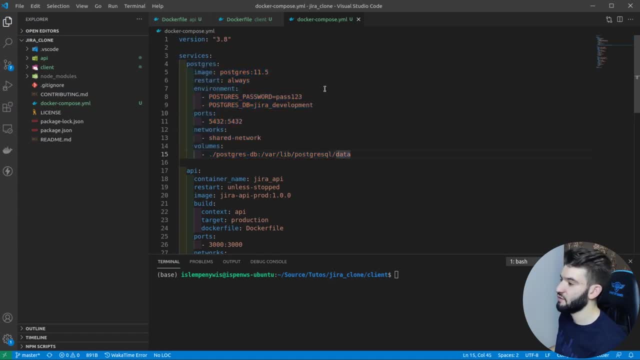 pretty much the criteria provided in here: the pores, the environments, variables, the Docker files or what image you're going to use already or all that sort of stuff. So it's going to start Postgres, it's going to start API and it's going to start client, all at the same time with a. 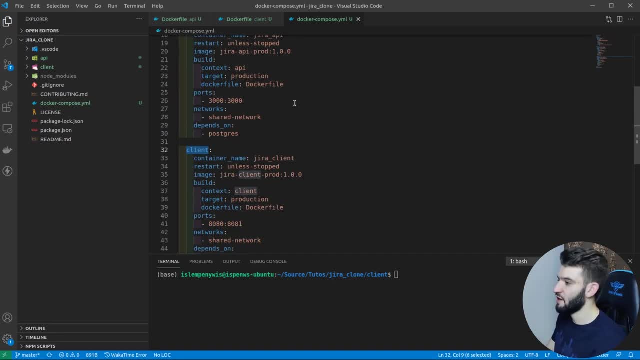 single command And that's it. that's, that's all you have to worry about. And Docker compose even it has like this kind of demon mode where you have to run it once and never just. you know, think about it before, Because servers, of course you've got to. 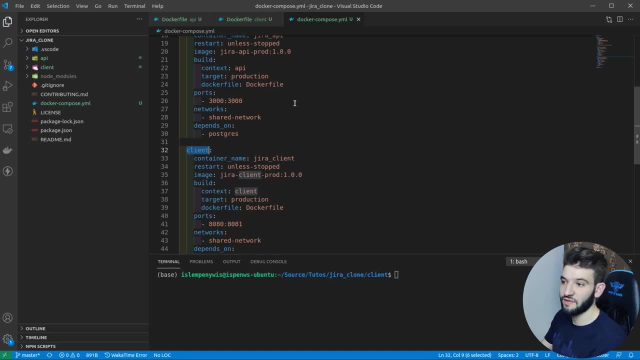 run those on a demon And once a server is restarted or something like this, like a composer is going to take care of this behind the scenes for you. So, simply, all you have to do: just go ahead and run the Docker compose command And Docker compose is going to take all the rest. 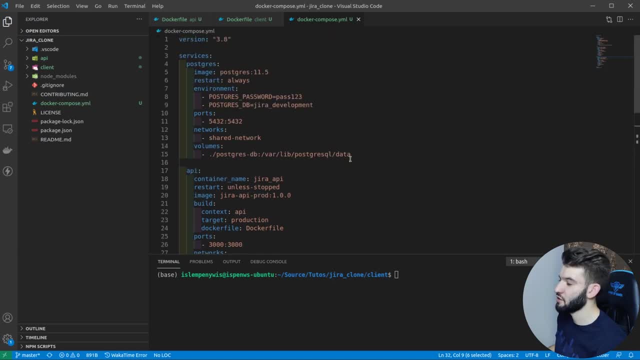 depending on the Docker compose YAML file you provide in here with all of these configuration. How sweet is that? Pretty, pretty awesome, And that's what I like about this. Alright, so let's go ahead and run all of this And, first things first, we're going to use a Docker. 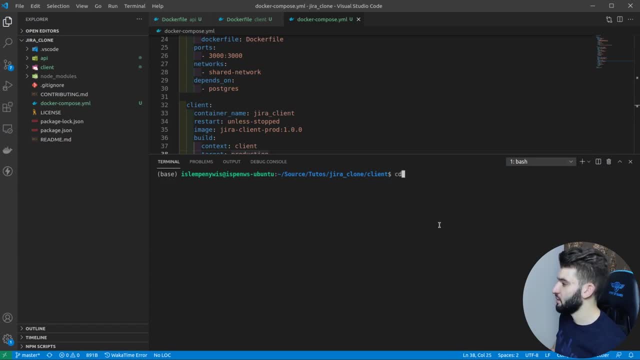 compose. make sure you are on the route, which I'm not. So we need to go ahead and back into the routine here where the Docker compose actually exists and run, Docker compose build, And this should go ahead and build us everything from scratch. So we start from take the log: where is? 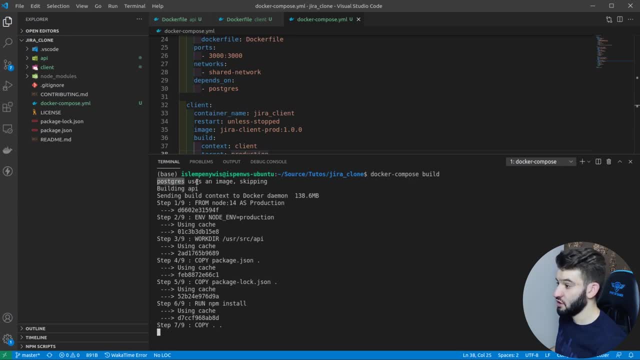 that. So it's going to build in API and Postgres uses an image already built. So this is why it's keeping it and just like going and building all of that And, of course, it's going to take a couple of minutes because you're going to build a couple of images. 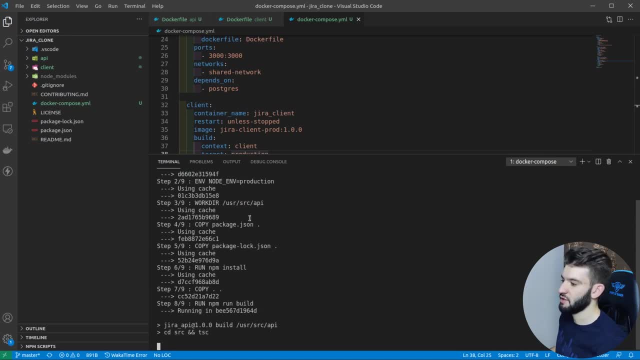 And it's going to install dependencies and all sorts of stuff, So we have to burn this and wait a couple of minutes to finish up, of course, And there you go. So that is. that is well made up. actually, took a couple of seconds to a minute to build up everything. So now we got the images. 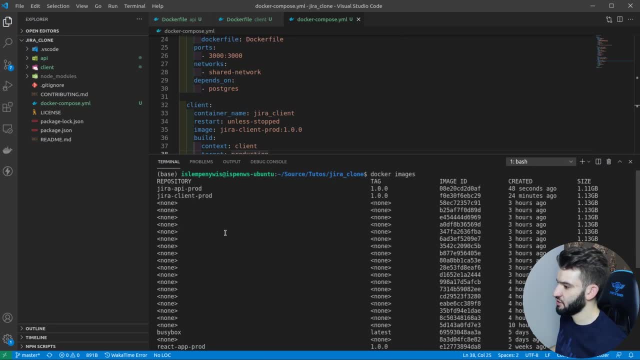 built up. of course you can go in and do like Docker images to check out the images built up. take a look on it. Those are actually our images built up. like you know, 20 or 40 seconds or whatever. This one has built 24 minutes. I think this is a cache version. When I 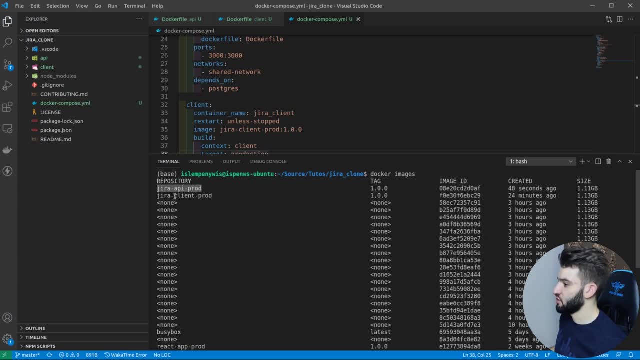 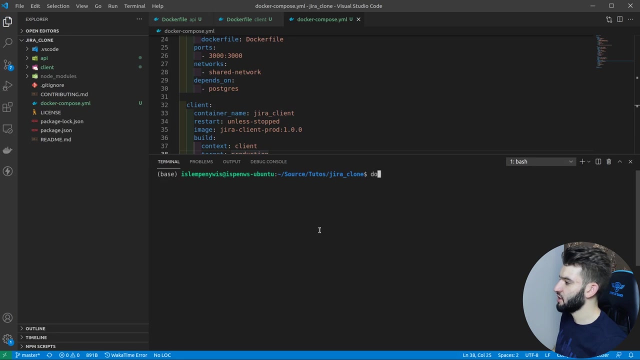 tried it before, but whatever. So JIRA API production, JIRA client production, version tags, image IDs and all sorts of stuff. Of course the size is tremendous because we got extended. the node is kind of like image and having our custom stuff going on. Now we got everything built up. 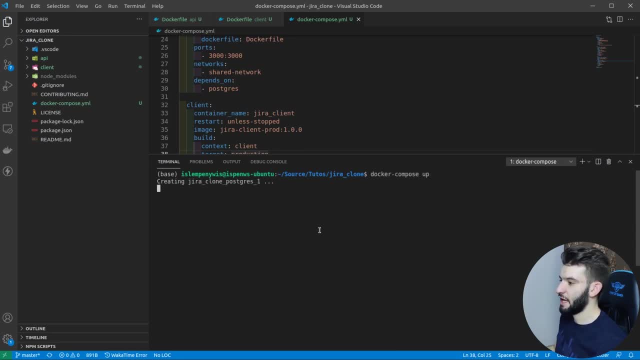 Now the second one we need to do is go ahead and do like Docker, compose, dash up, And this is the best command of the word And all it's going to do for us: going to take care of everything. from here, it's going to run all the actual 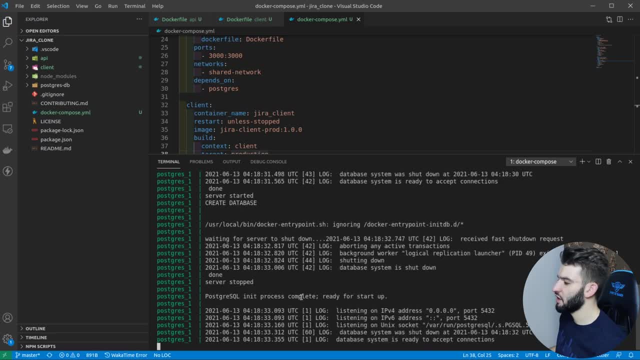 services together. as clear as he's taught. all the service is going to print out all the logs from different services in different colors, which makes it really really awesome and really well readable. And now the application started, the API started and the client started as well. Plus. 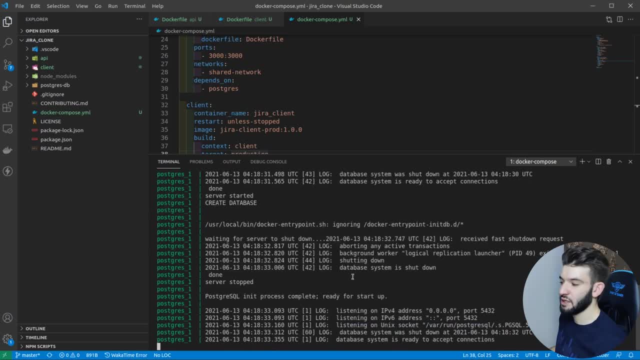 the Postgres now is actually accepting connections. So everything, literally everything, is actually connected together with a single command, with a single file And everything is actually Dockerized with Docker files and everything. How sweet is that? Now, if you go in and take a look onto this, 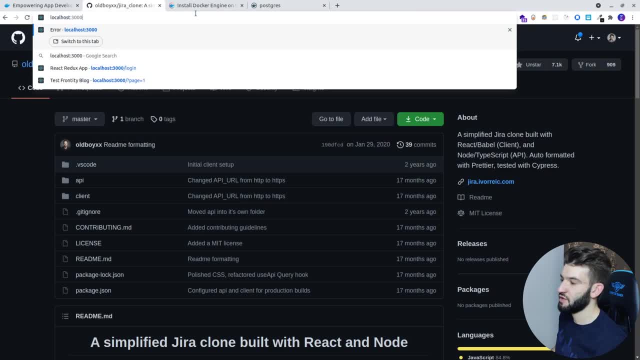 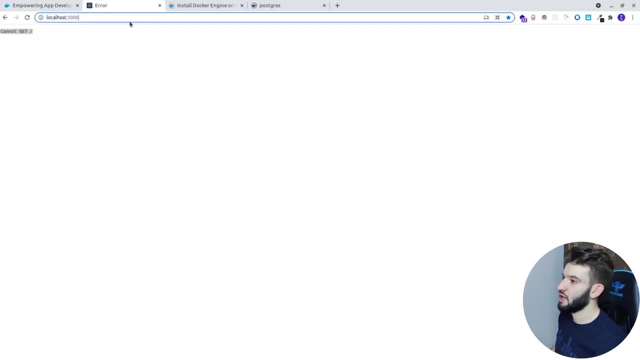 remember we already exported those kind of like. if we go to the 3000, where the server lives, there you go. we got this cannot get because the server is kind of like runs on different rounds. And if you take a look on 8080, where we got our client running, take a look on this and it's. 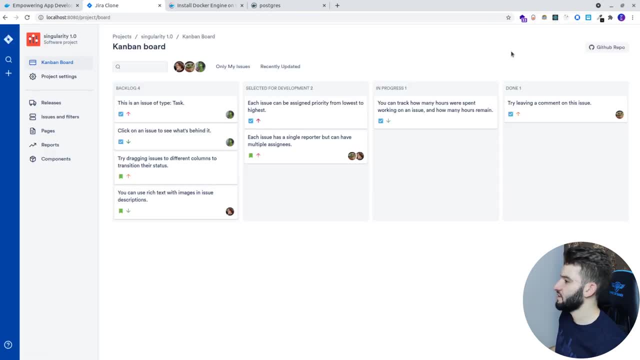 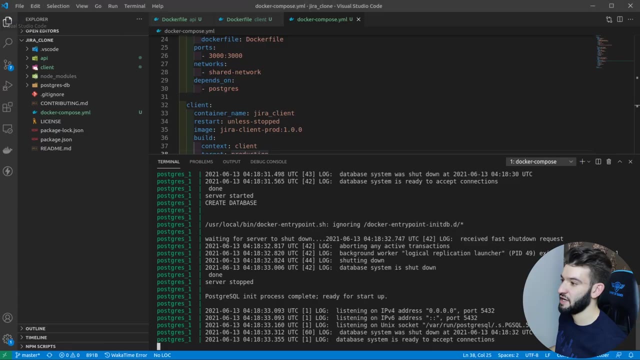 spinning, spinning, spinning. Hope that doesn't take forever. There you go. we got the whole application in here. it's kind of Jira clone and it does look really well made up as a Jira clone And yeah, I kind of love this as crazy. It runs from this: 8080 ports running on a Docker container On top. 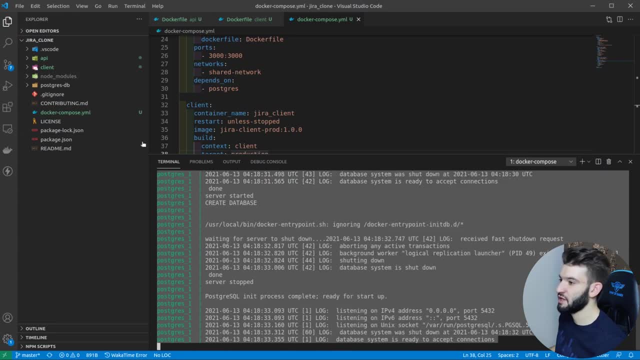 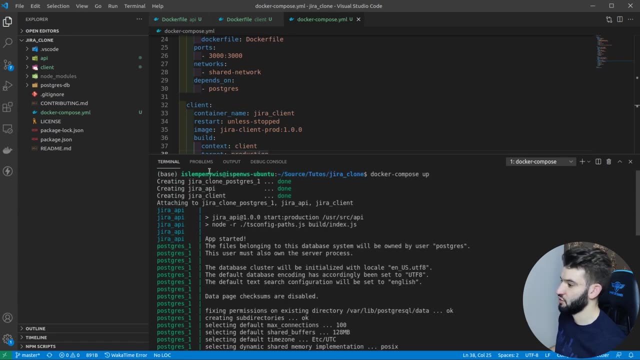 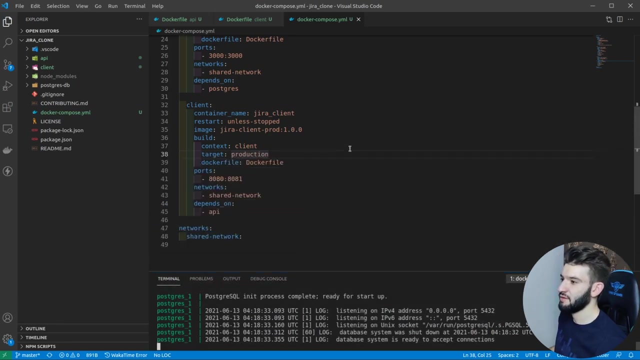 of this, everything is running And indeed the Postgres is running, is accepting connections, And this Postgres is actually connected to the actual client pretty much for the API in this real way. Now, one thing I actually didn't manage mentioned, which is kind of tremendous and you might find a. 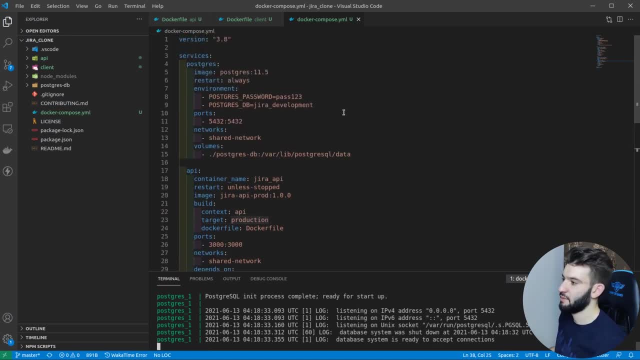 little bit issues, if you're not familiar with much of Docker composed on that particular parts, of how to link this together, of how to link, like the API together with with pretty much like the Postgres, like in terms of hosts, because right now they all run in terms of Dockers and the same network. 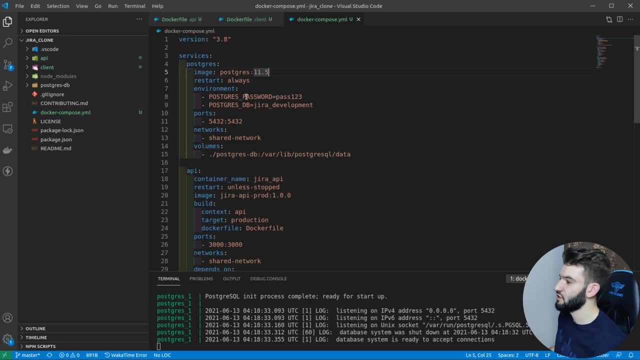 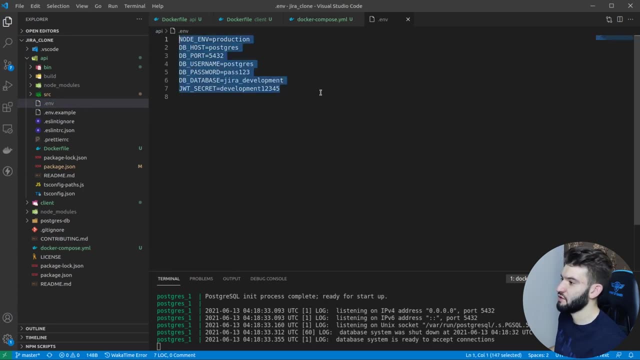 And they don't know, like, what localhost is or something like this. So how to link this one? what you need to go ahead, it's actually like, for example, like the MV it's created for the MV file, like where the configuration live, So you can have this anywhere in your code. 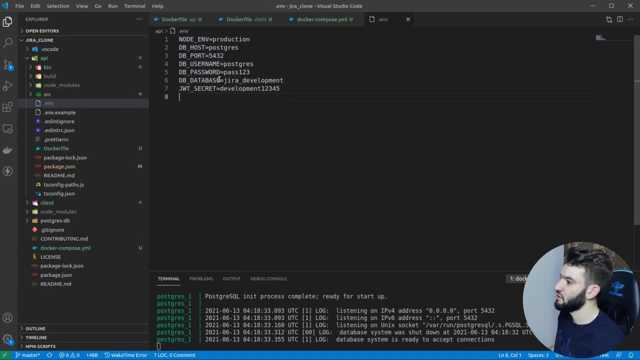 like where, where you pretty much do database setup or something like this. So for the password, I'm passing in my password in here, like the database name and the username and everything for Postgres And the other part in here, exclusively DB host and 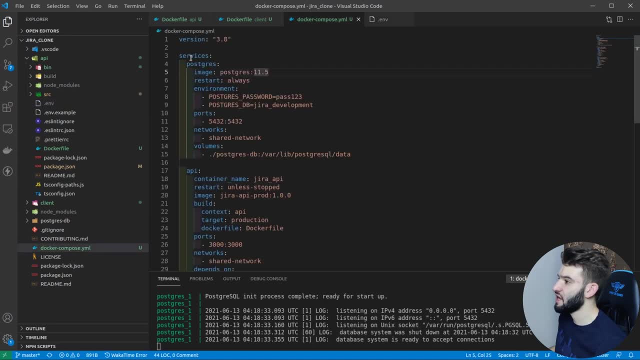 using this Postgres And this one represents the same name of the service, because that's how Docker internally actually resolves host names by just like their service names or Docker Compose. So that's basically how you point it that way. If you want to like point it to the like from the API, tell it I. 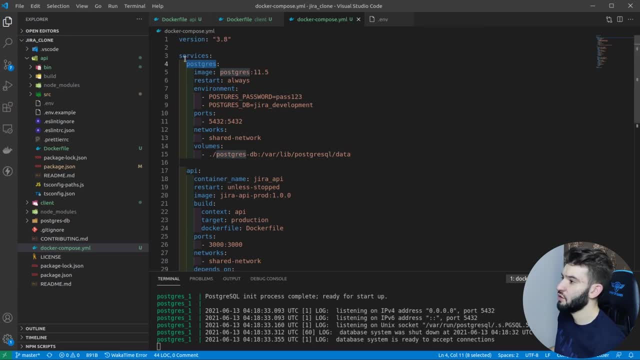 want to access the Postgres equals database server. we just like pointing to the service name in here, just like provide the service name. So whatever you change in here, change it there, of course, and that's it. So just like point it that way. 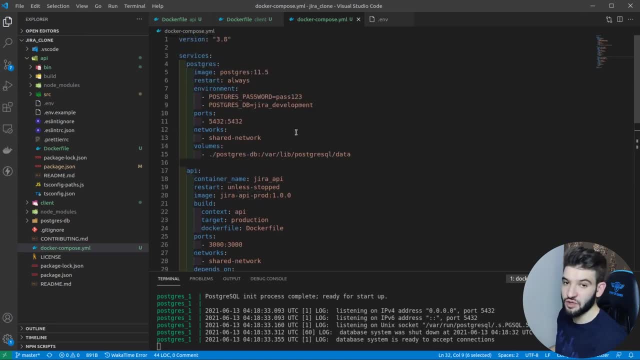 If you want to point the client to the API, like you want to have, like restful API, of course, connected to the to the API and do connections, So we have to point it to is actually this API service. So instead of doing like localhost, then 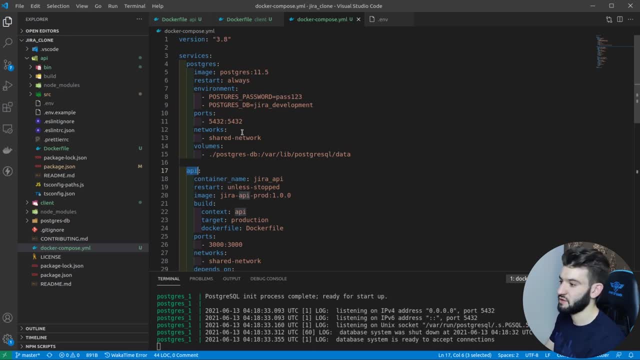 wherever routes you got. you do like API, then forward slash, whatever stuff like this, And Docker is going to do the job perfectly for your Docker Compose is going to like handle this behind. this is going to resolve. the right address for you is going to like bind it and everything, So all you have to 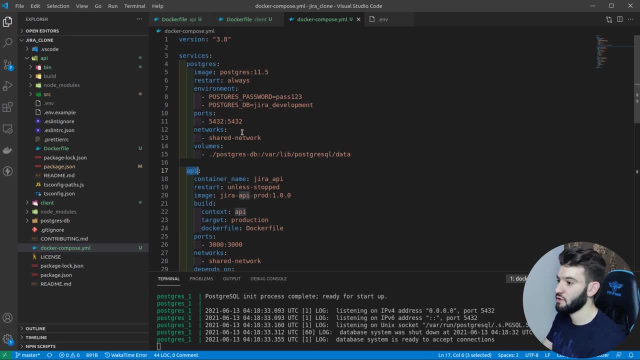 worry about just provide the right service name for your container to be able to communicate to each other's internally. Otherwise it won't work for you. So, yeah, that's that's pretty much it for these guys. Hope you guys enjoy this video tutorial. I tried to make this as simple as possible as 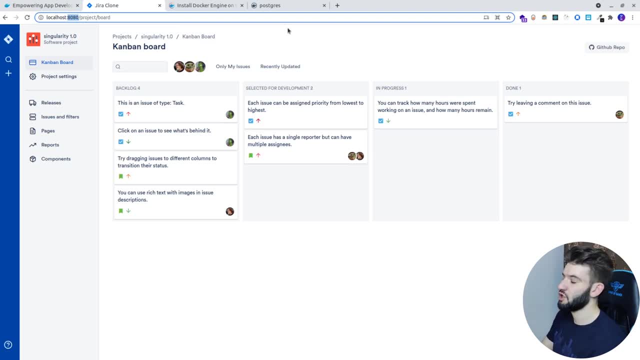 quick as possible. I tried to like provide everything as you need to actually take a Docker from start to finish on how dockerization works and how dockerizing a real world projects from start to finish throughout react nodejs with PostgreSQL And with a whole kind of like stack of servers. Plus, we also use some Docker. 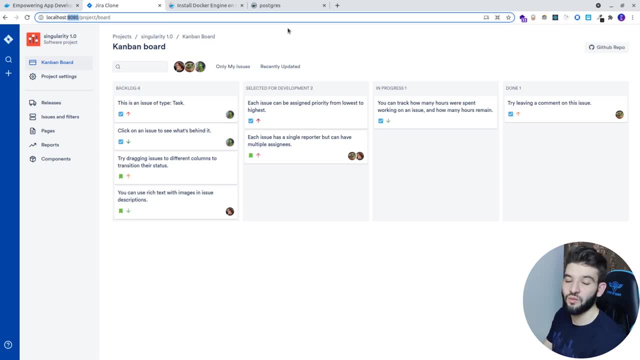 Compose to put all these services in a single file and have them running up with a single command. So hope you guys all enjoyed this one. I enjoyed making every single piece of this video and hope you all guys actually liked it. Without further ado,